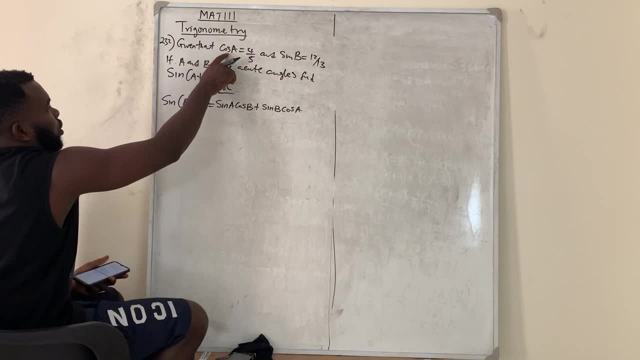 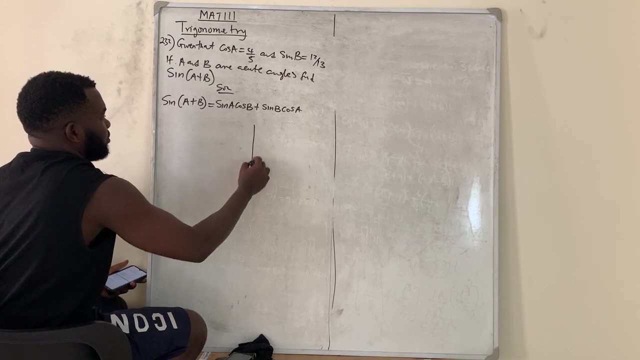 we need to get our our cos uh, cos b, and then sine a, so that's all we need. so what you do is just to draw. draw for me, if you draw this, you have that. draw two triangles. the two triangles we have are this and this. all right, so now, and they say that they are all acute. so i have that. this is my a. 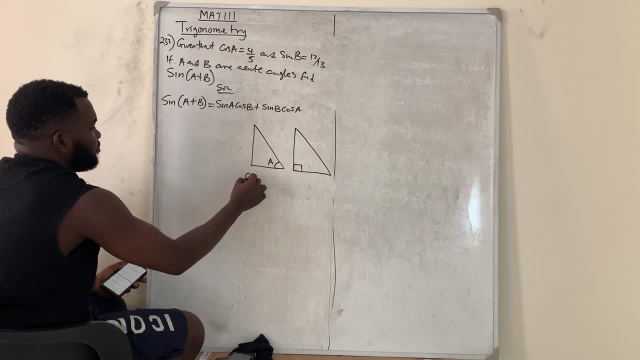 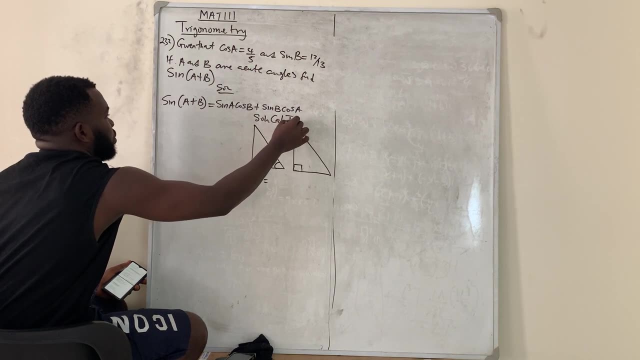 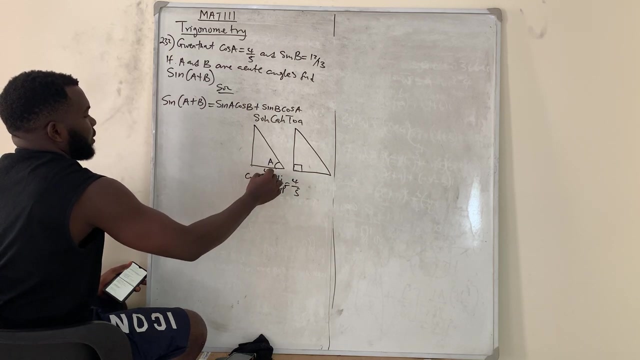 if here is my a now, don't forget that they gave me cos, cos a, and cos is what adjacent soca twa we are using. so car right cos is adjacent over hypotenuse, so adjacent over hypotenuse, so which is what they gave me as four over five. so which is my adjacent is four. 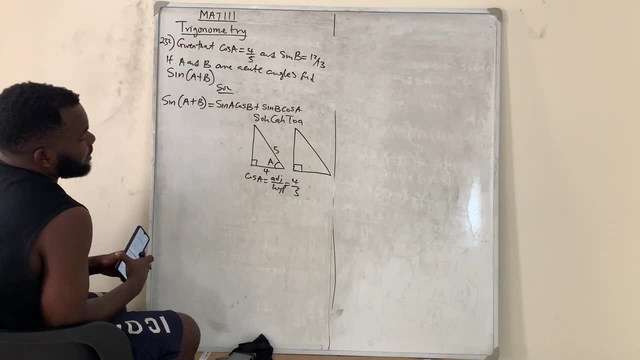 and my hypotenuse is five. don't forget that um other sense is just the remaining side. opposite is the side that is facing the angle, why hypotenuse is the side that is facing the 90 degrees right. so this one now is my b, so they gave me the same thing. okay now. so let me find my uh. sine sine a. 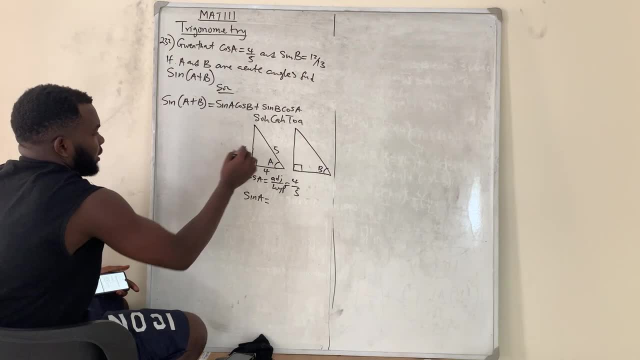 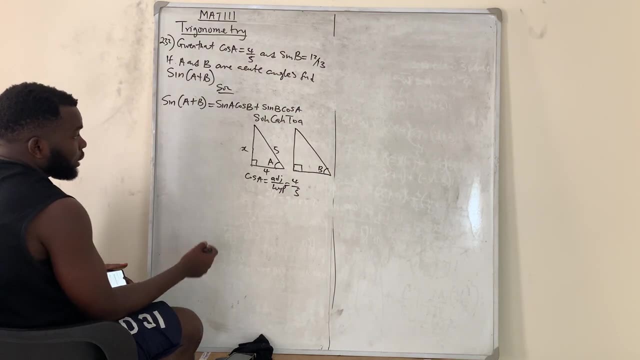 sine a. now, according to trigonometry, let us find here: okay, but it's supposed to be three, because this is pythagoras triple. three, four, five. so you're supposed to be three. but if you don't know that it's pythagoras triple, you can find it using your pythagoras theorem. we said: 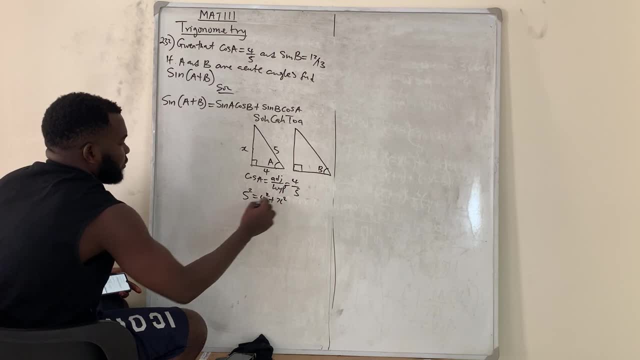 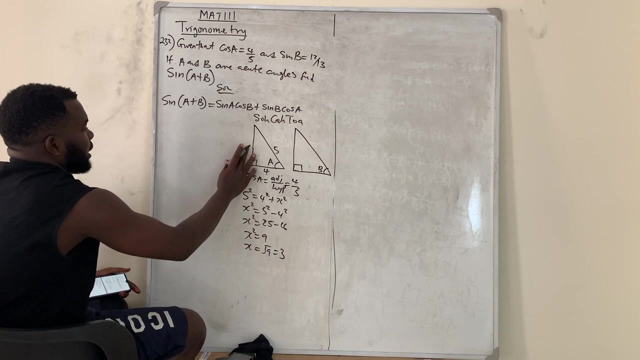 5 squared is equal to 4 squared plus x squared. so you have that x squared is equal to what, 5 squared minus 4 squared. so x squared is equal to 25 minus 16.. so x squared is equal to 9. so x is equal to the square root of 9, which is 3. so you see that here my x, here is 3. so if 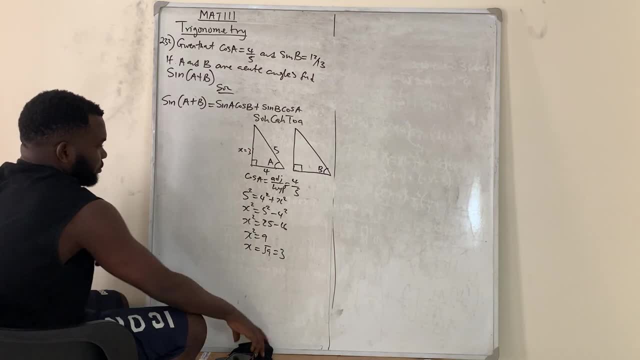 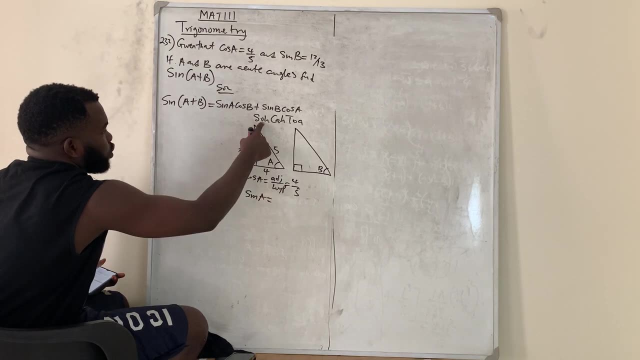 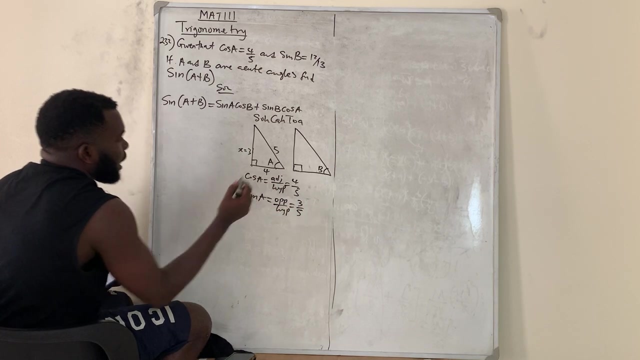 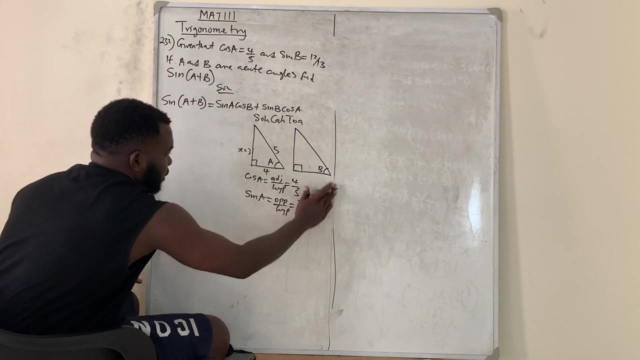 i've gotten that here is 3, so for you to get your your cos, theta, sorry, your sine a, your sine, sine a sine is what, opposite over hypotenuse. so opposite over hypotenuse and opposite is 3, then hypotenuse is what five, that is for for a. now coming to b, they gave us um 12 and 13, but what they gave us? 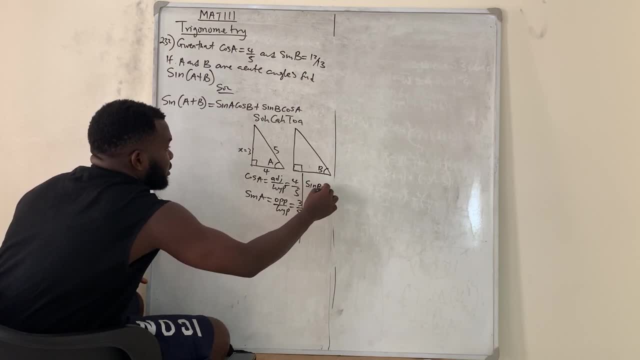 there is a sign. they say that sine b is equal to what. you know, that normally sine b is opposite over hypotenuse, which they gave us as well, 12 over 13.. so i have that here is 13, the opposite is 12.. 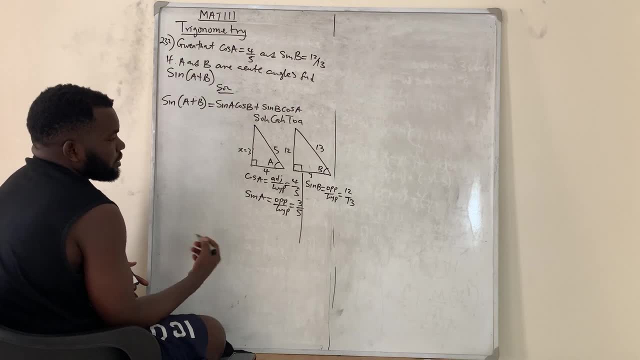 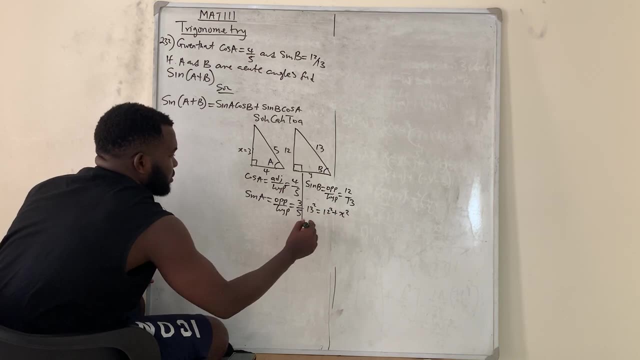 so the remaining thing is just to get my adjacent. to get my adjacent, we can use pythagoras theorem again. that says that 13 squared is equal to what 12 squared plus x squared. all right to have that. what x squared will not be what 13 squared minus. 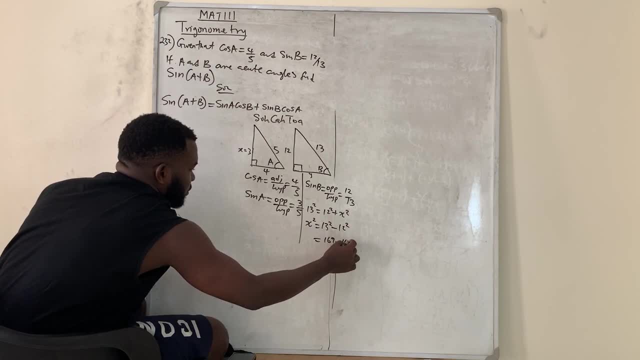 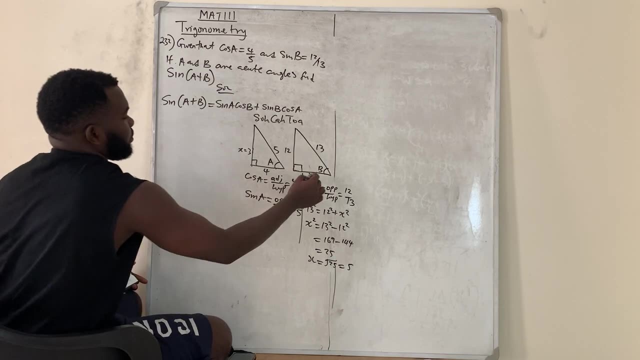 12 squared. so which is what? 169 minus 144, i think, is 25. so to have that, my x is not squared of 25, which is what five? so pythagoras would say: 5, 12, 13. so that is that. so from here i can get my cos b. 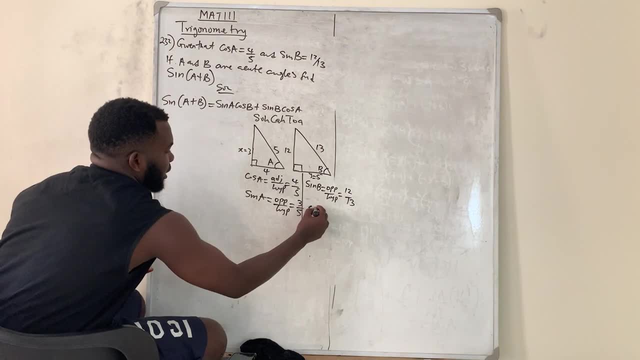 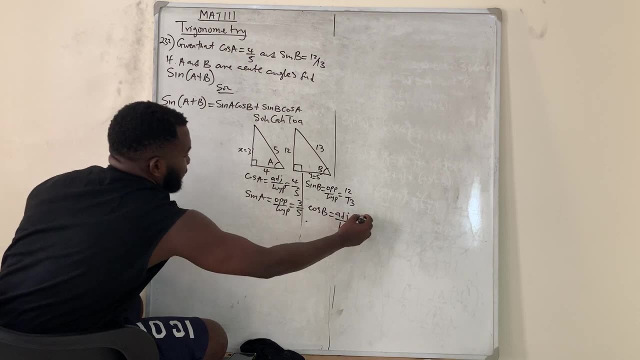 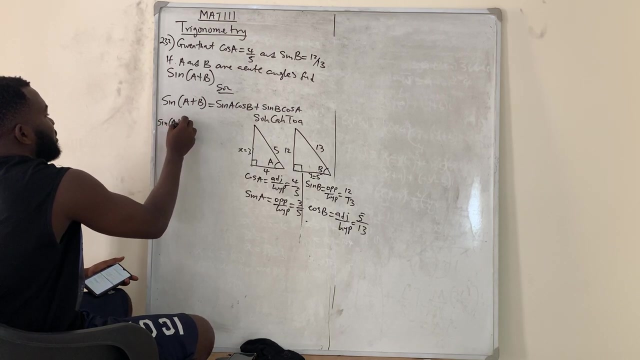 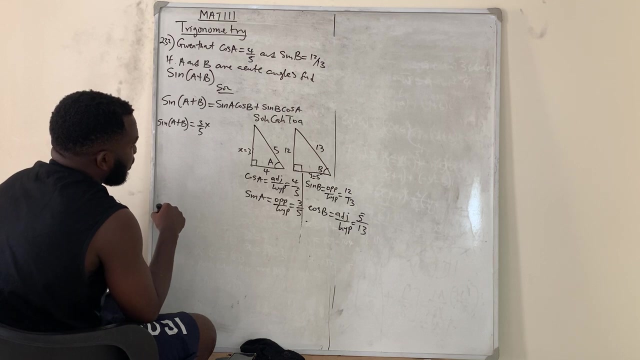 okay, from here i cannot get my cos b, so my cos b will not be what i just sent over. what hypotenuse which is adjacent is 5, then over hypotenuse is 13.. so if we cannot put it here, we have that our sine a plus b is equal to sine a is 3 over 5. 3 over 5 times uh, cos b. 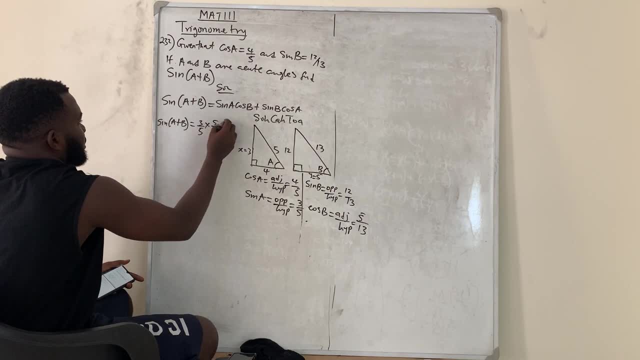 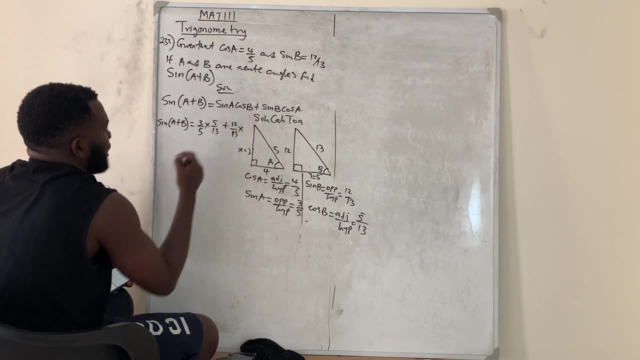 cos b is 5 over 13, 5 over 13, plus sine b. sine b is 12 over 13, 12 over 13 times cos a, cos a is 4 over 5, 4 over 5.. so if you look at that now, 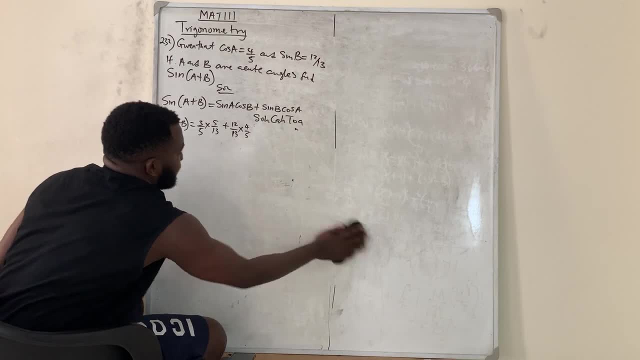 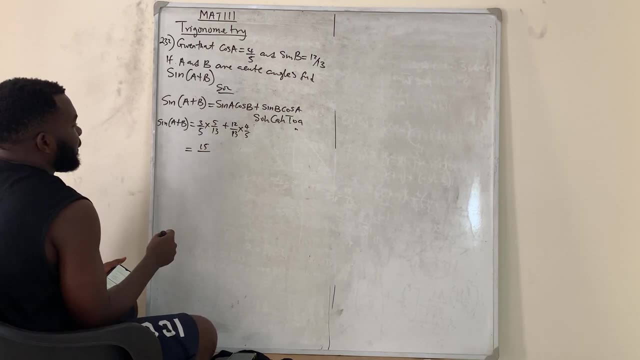 permit me to clean this one i've done here. so if you look at that, you're going to have um, you see that you're going to have that um. this is 3 times 5, is 15 over. or let me say this: take care of this to have 3, 3 over 13 plus. uh, can anything cancel the new? or let me just do it this: 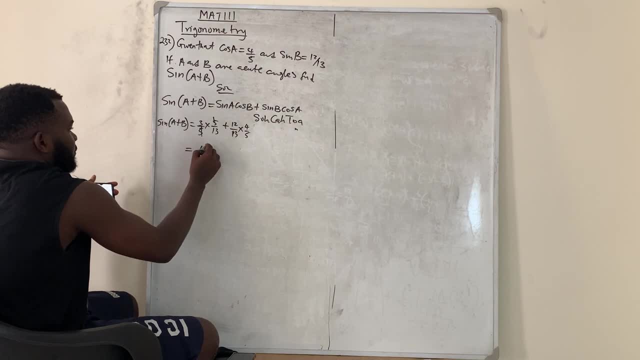 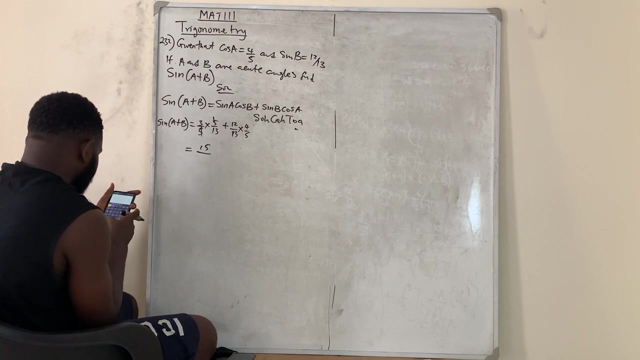 way with that cancellation. three times five, fifteen over five times, uh, five times- this is my calculator- five times thirteen, five, five times thirteen, i will have what? 65.. so 65 plus 12 times for 12 times 4.. i have 48, so this is 48 over 65.. so the lcm is now. 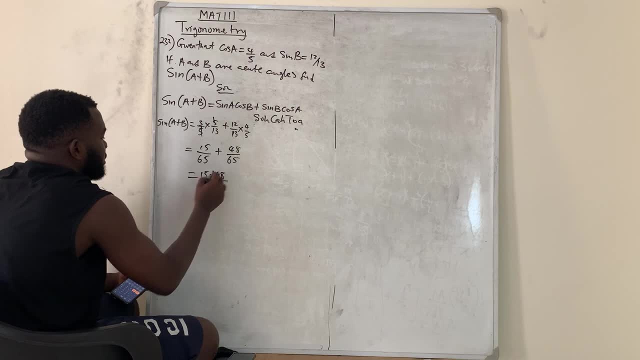 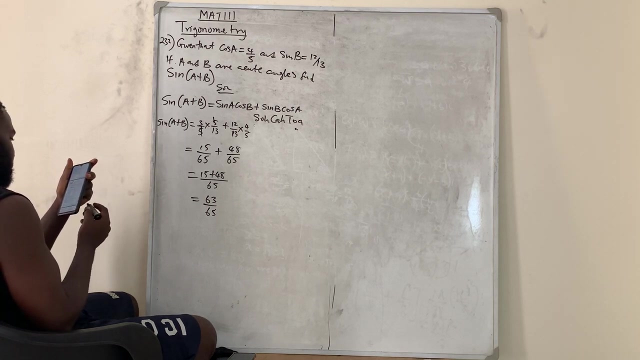 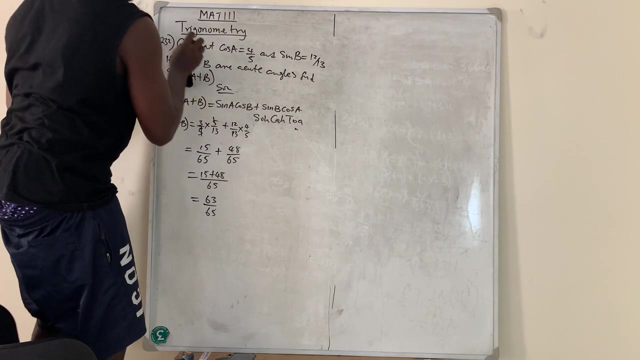 lcm is now 65, i have 15 plus 48, so which will give you plus 40? uh, plus 15. so which is what? 63 over 65. so that is the answer to that particular question: 63 over 65. okay, so we move to the next question, question number 233. 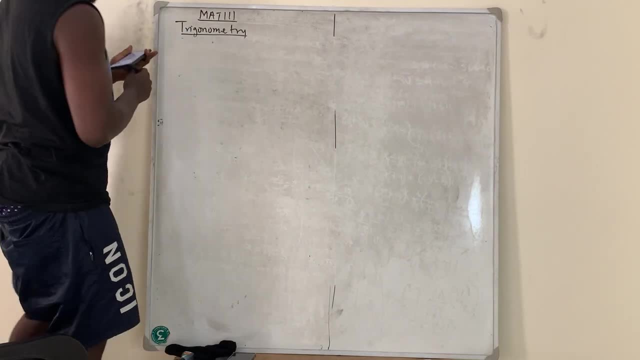 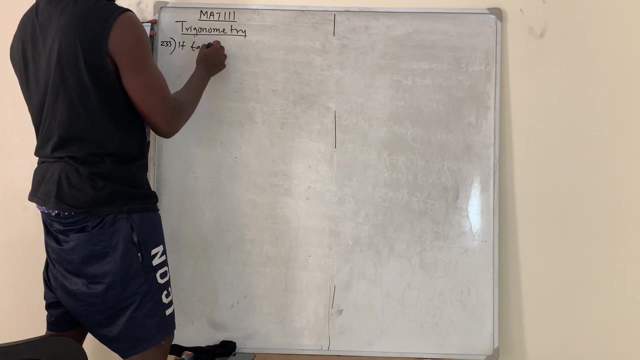 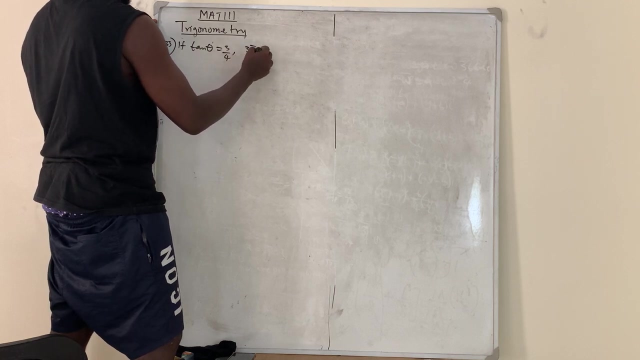 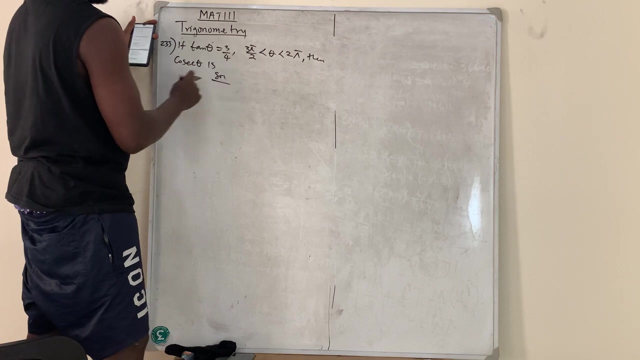 so question number 233 said that if, if tan theta is equal to 3 over 4 and theta lies between 3 pi over 2 is less than theta which is less than 2 pi, okay, then i say then, then, then, then, then, cosec, cosec, theta is solution. now, this is, this is very, very important. they say that it. 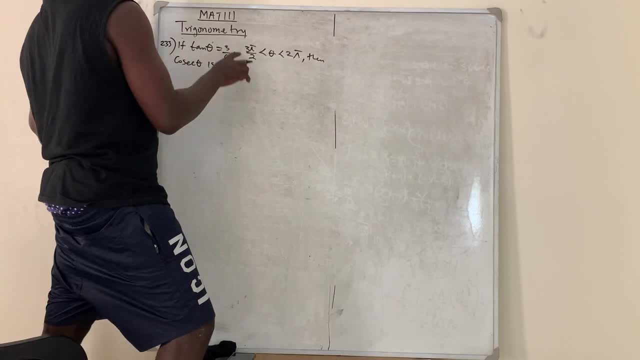 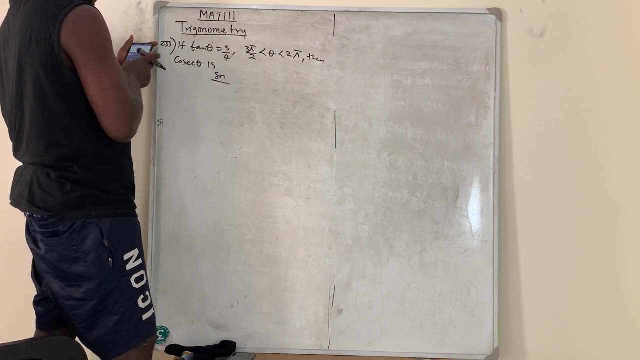 lies between 3 pi over 2 and 2 pi. 3 pi over 2 means 3 times 180 divided by 2, we're going to have 270. so 3 times 180 now divided by 2, we're going to have 270. so which means, if you draw, 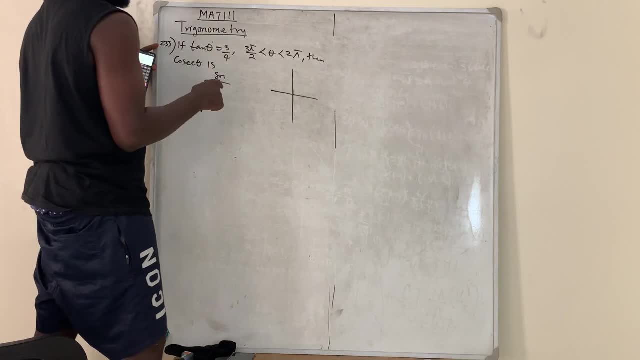 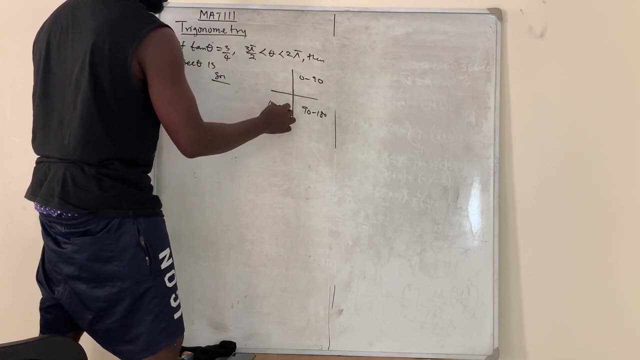 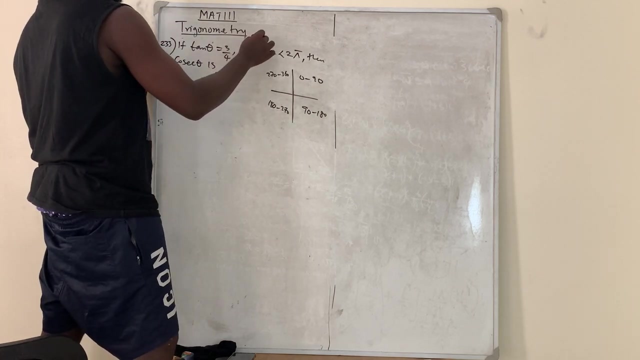 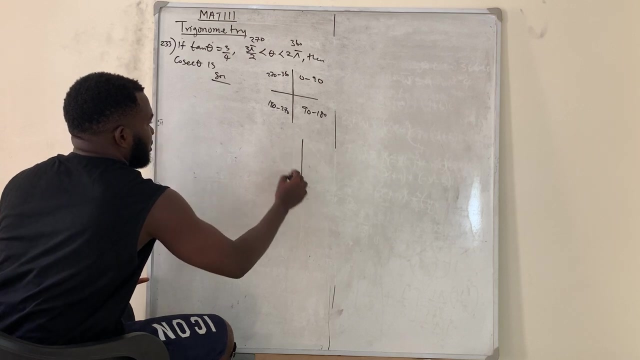 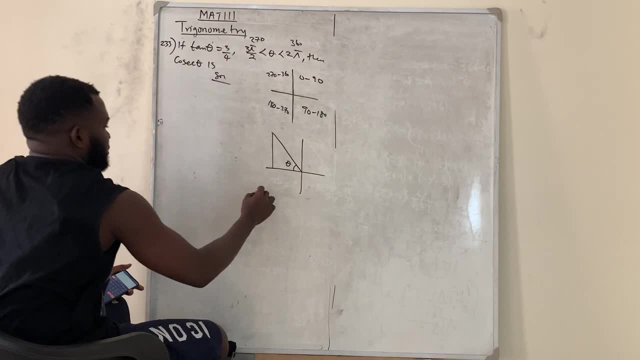 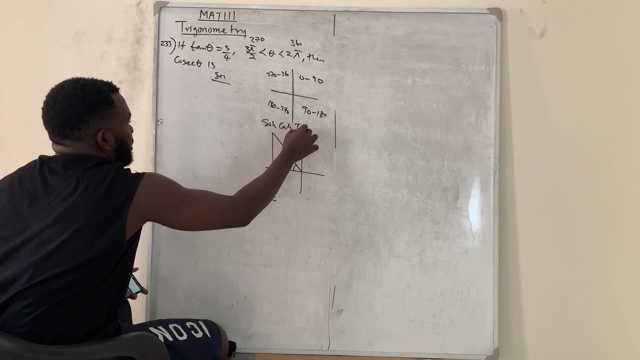 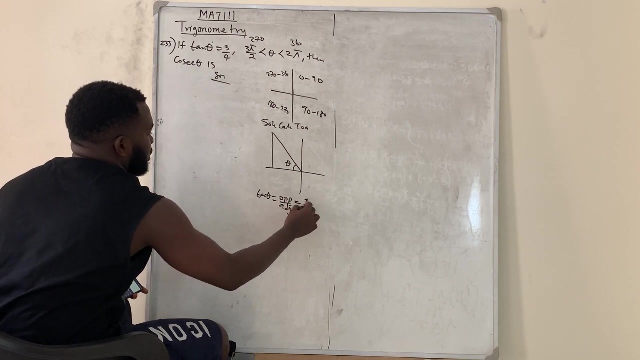 tan theta is opposite over adjacent, so tan theta is tua soca, tua soca tua. that is opposite over adjacent, so opposite over what adjacent, which they gave me as what? three over four. so my opposite, my opposite, is three, but my adjacent is four, so but the four is in the left hand side of x, so it's: 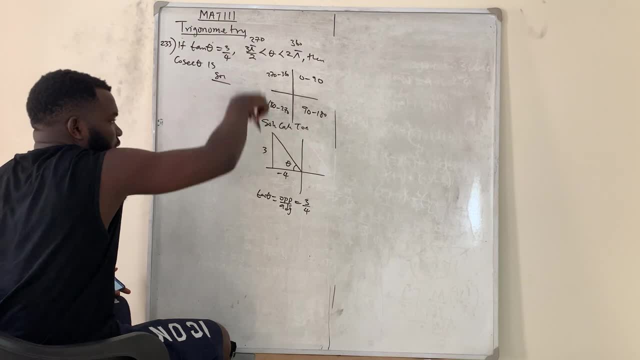 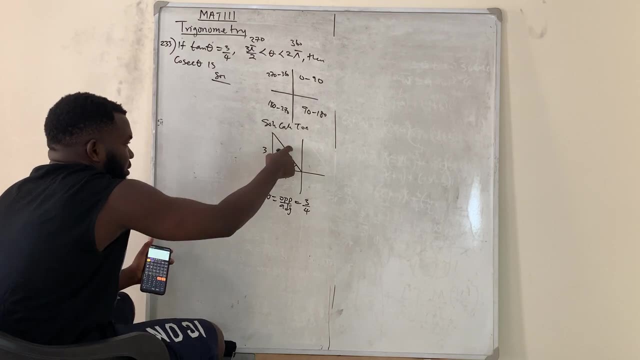 going to be minus four. all right, my three is in the positive y, so that is why it is three, but this is in the left hand side, so it's going to be what minus four. so i'm going to use pythagoras theory to get here. if i three, four, five here's supposed to be five according to pythagoras theory, so you: 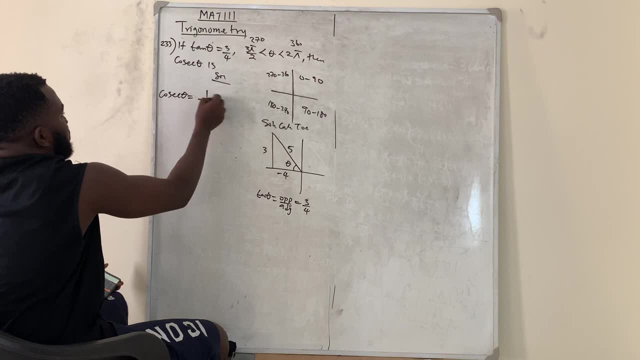 know that what cosec, cosec theta is equal to one over count three. one, two, three- i'm seeing x here- so one over sine theta. so which is what? one over sine theta is what? opposite over what hypotenuse. so one over means the inverse, so it's going to be hypotenuse over what. 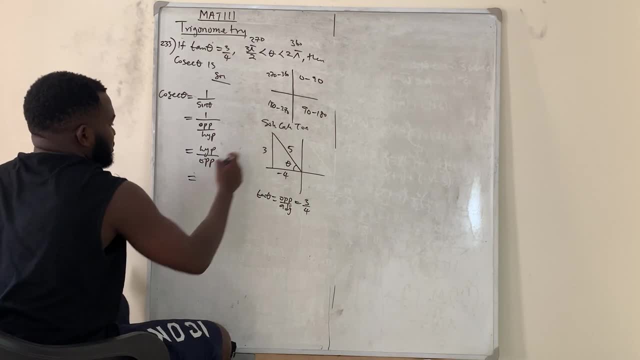 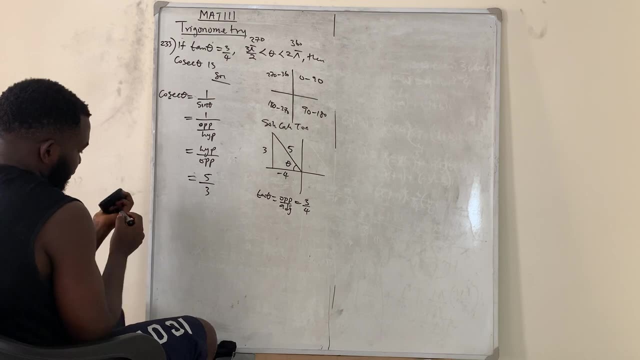 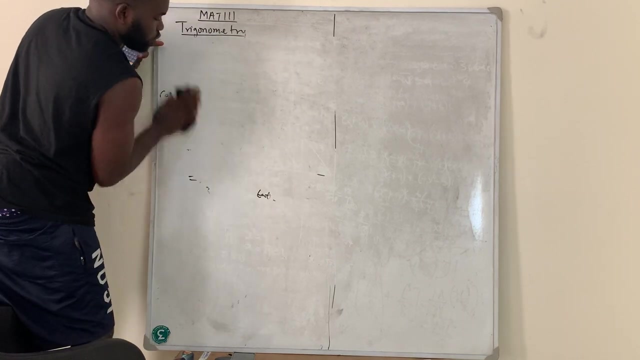 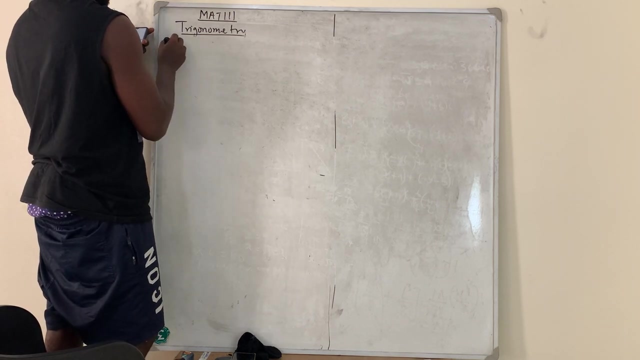 opposite. so what is my hypotenuse? my hypotenuse is five over my opposite. my opposite is three. so five over three is the correct answer there, right? so that is that we'll go to question number two, two, two, four. question number two: two, four. two, two, four. 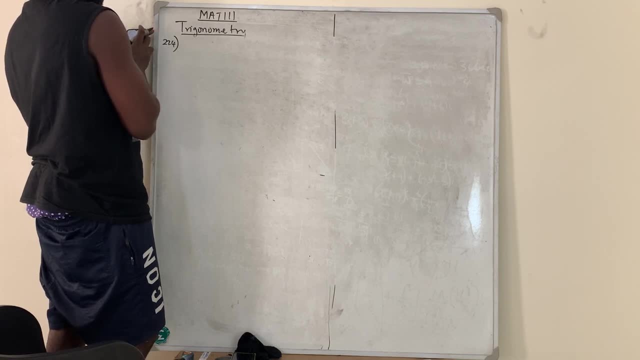 okay, question number two, two, four. where is my three? question number two, two, four said: if okay, two, three, four. two, three, four. the other one we saw, sorry, the other one we saw was two, three, two, two, three, three. this one is two, three, four. please correct the number. so two, three, four said: 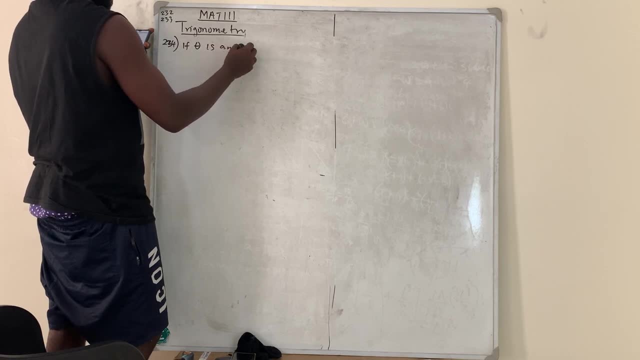 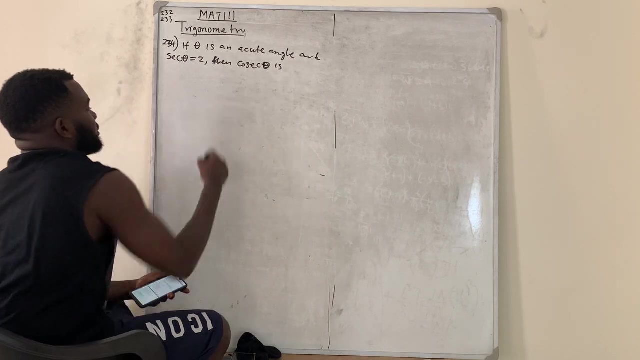 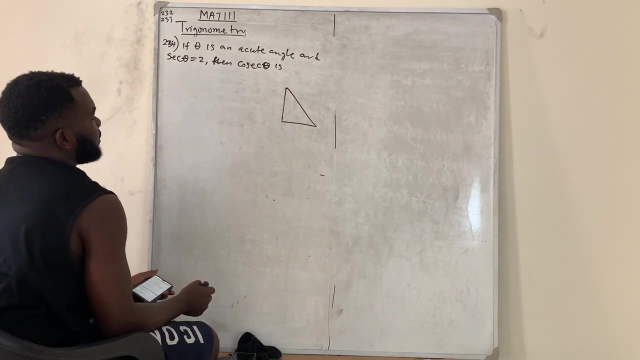 if theta is an acute angle and and the sec theta is equal to two, then the nasif, then then cosec, cosec, theta is okay. so now, since it is an acute angle, we don't have any problem at all. it's in the first quadrant. so, and this is my first quadrant, so now one. 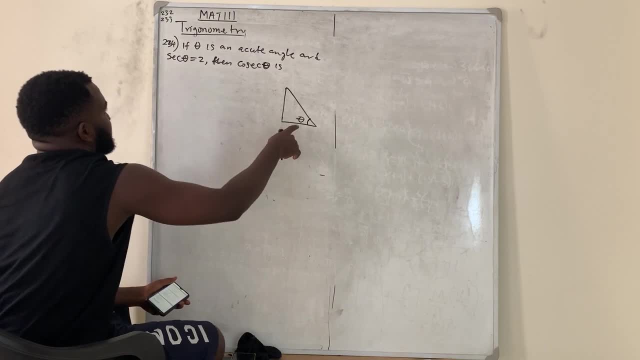 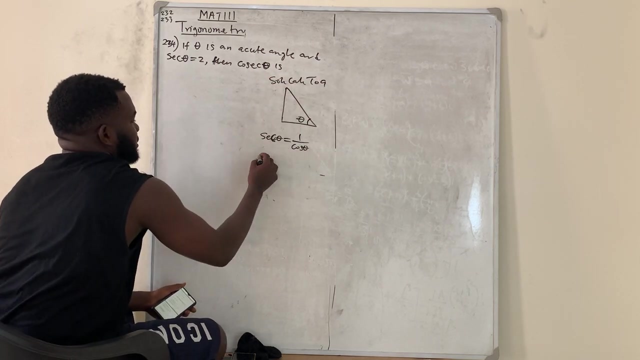 do we have? uh, we have that. this is our theta. okay, this is now sec, sec theta. sec theta is equal to say count three, one, two, three. i'm seeing c here, so that is one over cos theta. okay, according to so car tour, now sec theta is the inverse of course. cause supposed to be adjacent over hypotenuse. so 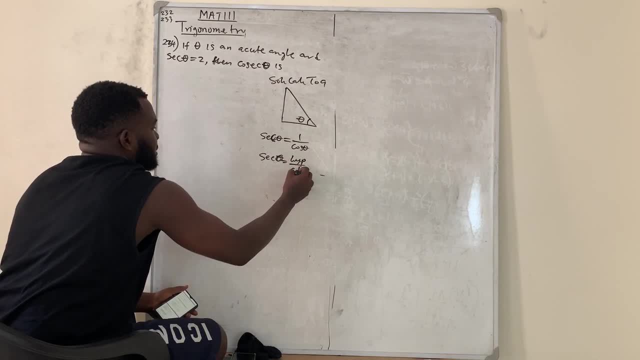 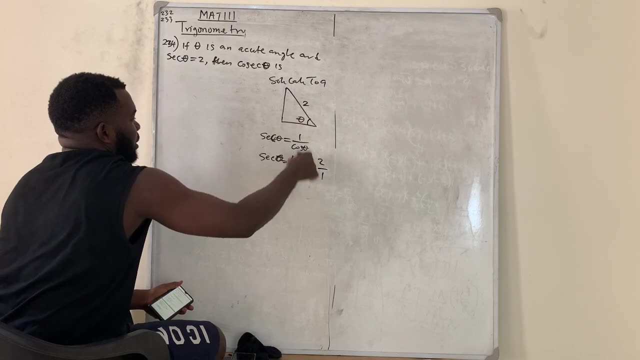 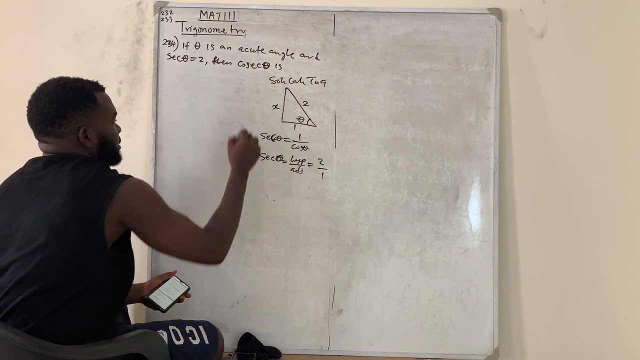 the inverse is going to be hypotenuse over what adjacent. so which means they gave me that is equal to what two. two is that saying two over one. so which means my hypotenuse is two, my adjacent is one. okay, my adjacent is one. so if i use pythagoras theorem to find this side, i will say that what? 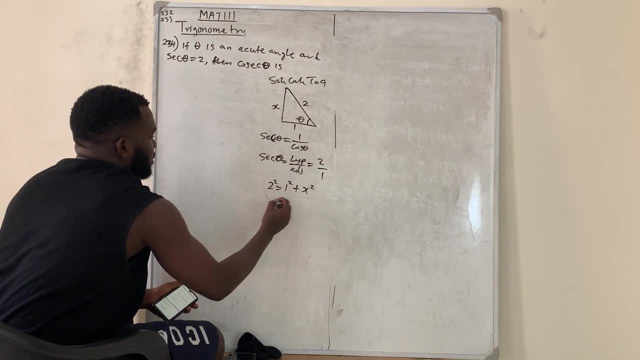 two squared is equal to one squared plus x squared. so therefore, x squared is equal to two square minus one square, which is what? four minus one, which is three. so my x will not be the square root of three. okay, so here is equal to what root three. so they say i should find my coast. 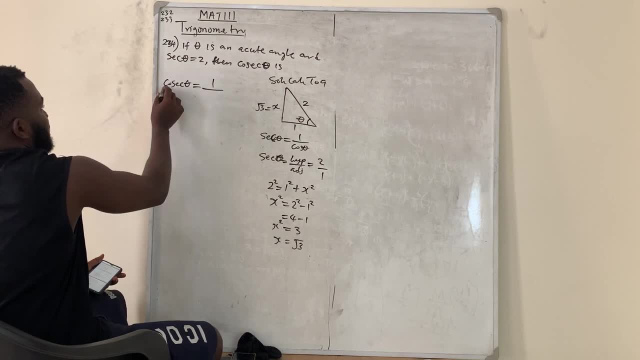 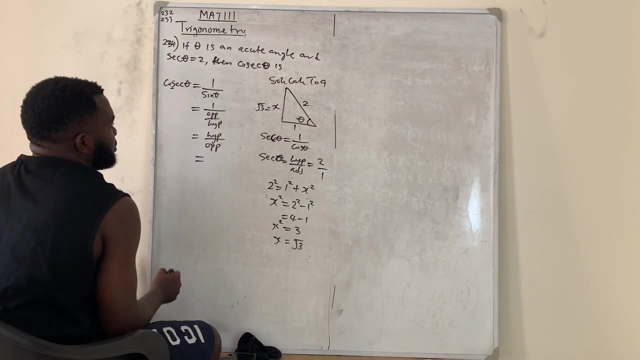 cosec, cosec, theta, cosec is one over count three, one, two, three x one over sine theta, which is what one over opposite over hypotenuse. so inverse of it will now be hypotenuse over opposite. so which is what hypotenuse is two and opposite is what root three. so it's going to be two over root three. 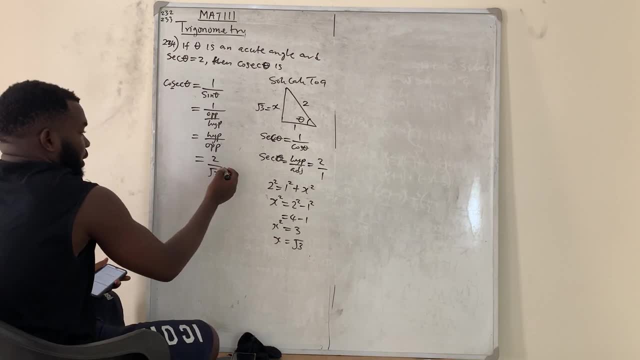 so two over root three is here, but if not, you are supposed to rationalize. if you rationalize, you're going to have two root three over three if you rationalize. but since this one is in the option, so this is the answer. so since this one is in the option, this is the answer, right, so we'll go to the 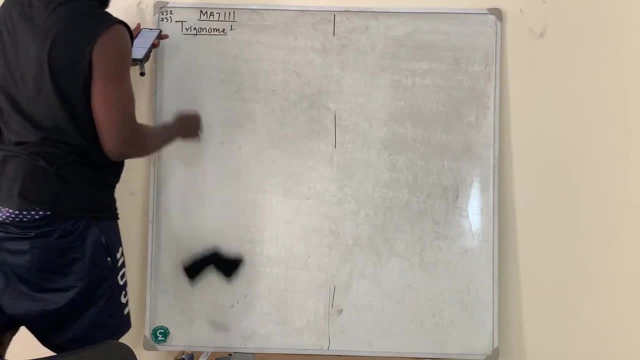 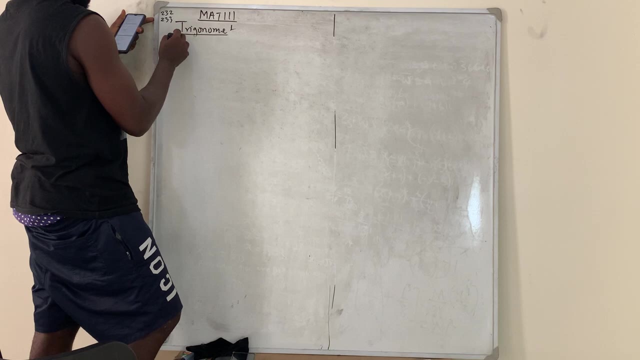 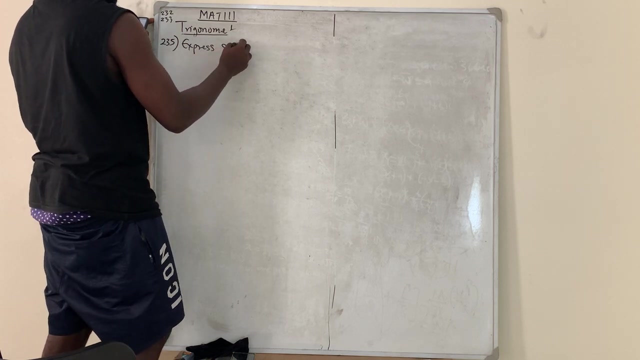 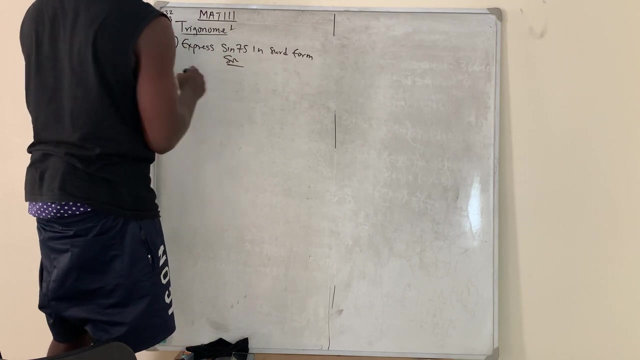 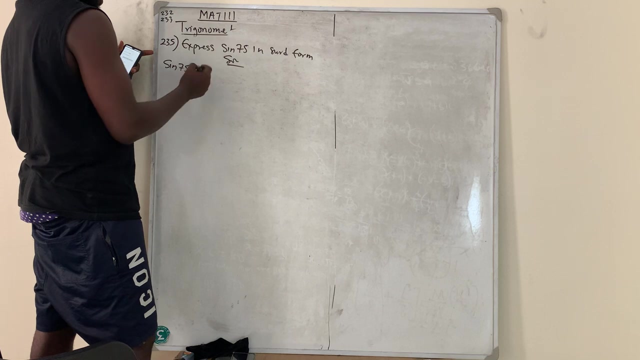 next question. so the next question is question number two: three, five, two, three, five. we said express express sine seven, seven, seven in sword, in sword form. okay, solution. this is very, very simple: sine 75 is equal to which two special angles can give you 75 is 45 and 30. so i have sine 45 plus 30. so according to: 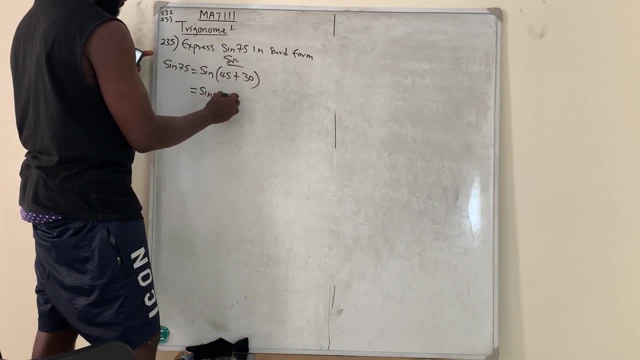 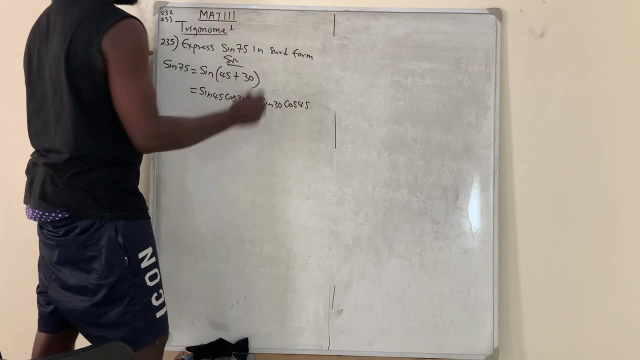 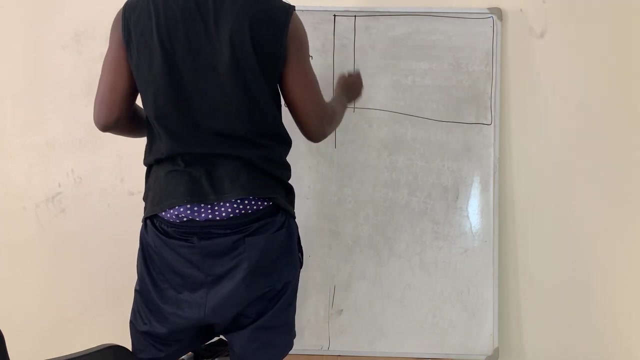 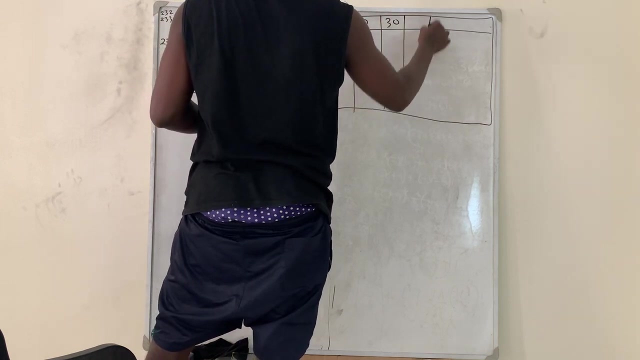 sine rule is going to be what sine 45 cos cos 30 plus sine 30 cos 45. so according to my, let me even keep my special angles here, so i can keep my special angles here. i will not be taking it as i'm solving my questions. so this is my theta, this is my zero: 30, 45, 60 and 90. 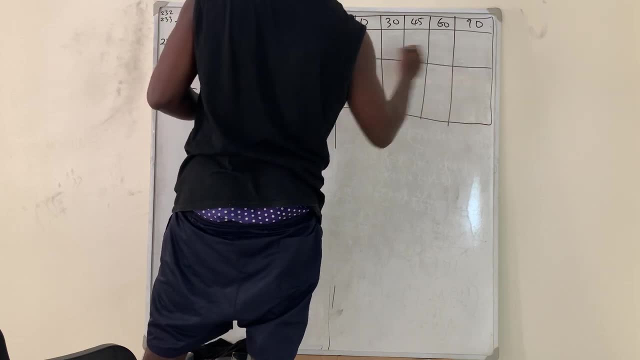 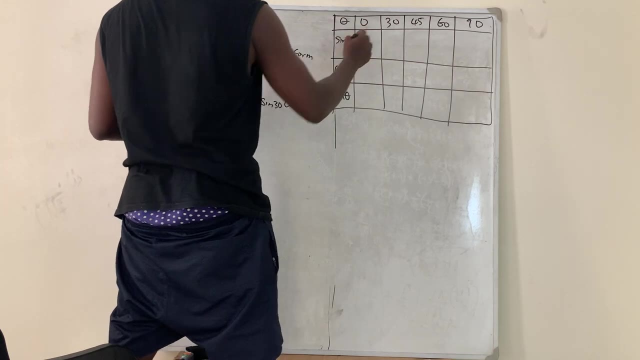 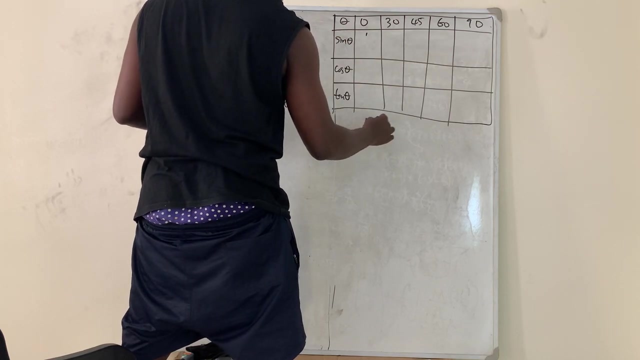 so for sign theta, cos theta and finally tan theta. so how do you get it? so just just say this is uh one. okay, let me just do it for the side of sign. is one, uh, one over four, the. the next line two over four, the next line three over four. then, sorry, zero over four. you start from zero, sorry. 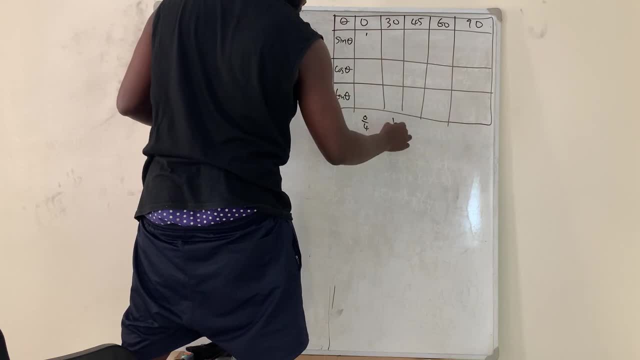 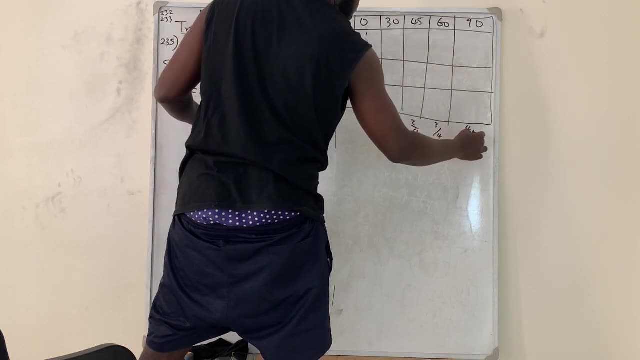 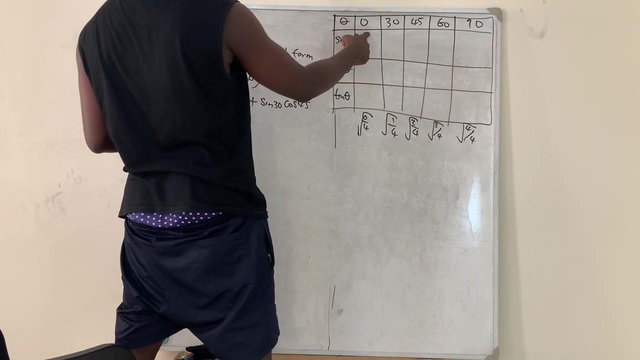 the first line is zero over four. the second line is one over four. this third line is what? two over four. fourth line: three over four. fifth line: four over four. then cover them with a square root. cover them with a square root, then you have gotten the answer. so sine zero means zero divided by four. 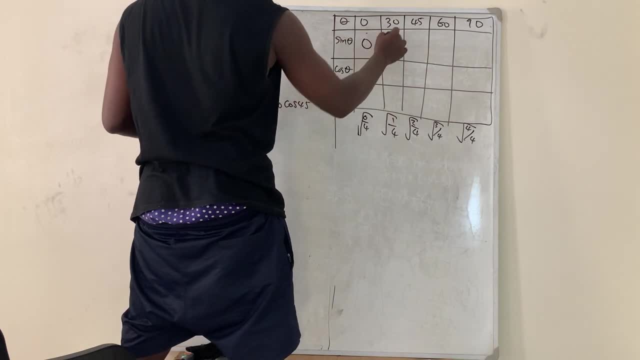 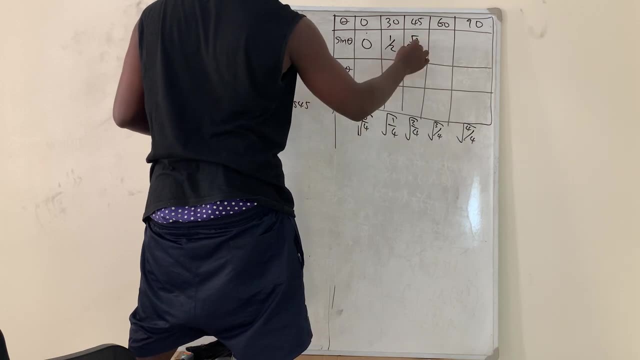 is zero. the square root of zero is zero, so here is zero. square root of one is one. square root of four is two, so here is one over two, square root of two. we don't know it, so it's root two over square root of four is two. square root of three. we don't know it, so it's root three and square root of four. 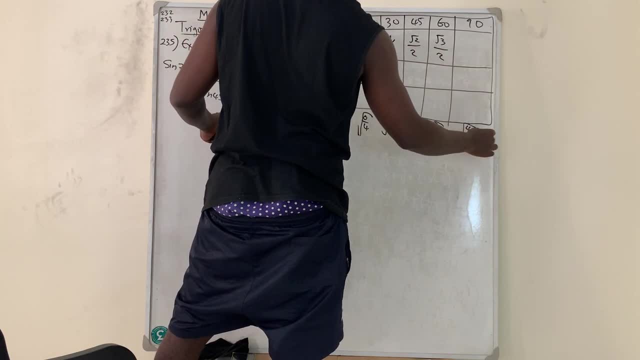 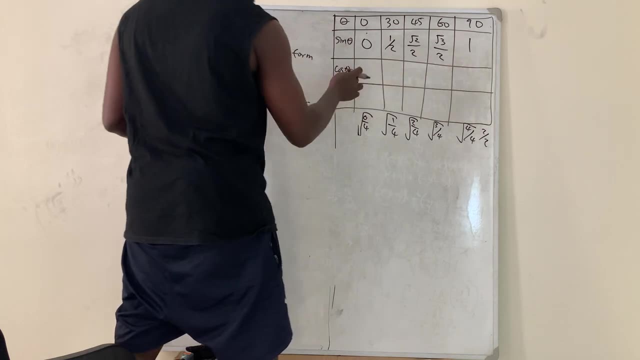 is two. square root of uh, four is two. square root of four is two, two divided by two. here is one. okay, once you have gotten this one, you have gotten the rest. how do you get the rest? now? start from this side. and right, we have started. you started from this. 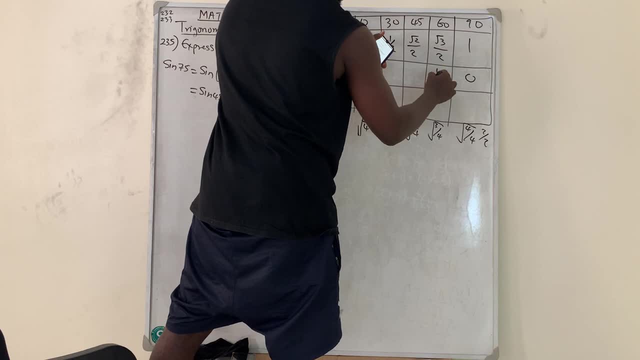 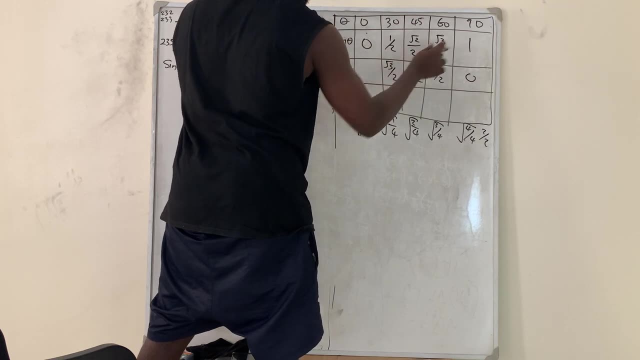 side writing. so start from here. so here will be zero. here will not be one over two. here we'll repeat: root three votes two over two, okay. here will not be root three over two and here number one: okay. so getting this side is d divided by this, this value, this will give you this, this divided. 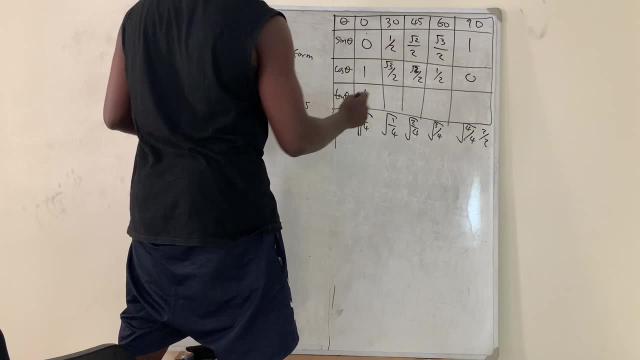 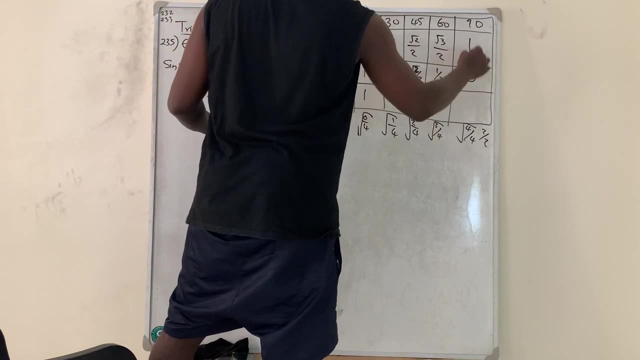 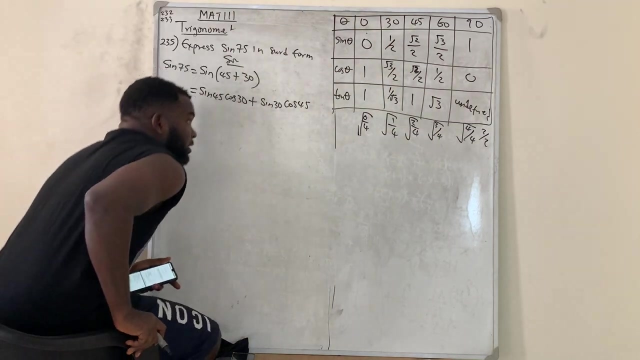 this will give you um one over root three. okay, these devices will give you one. these by this us root 3. this will give you undefined, because anything divided by zero is undefined. so that is how to get your special angles. so the reason i did that is because of this particular question. 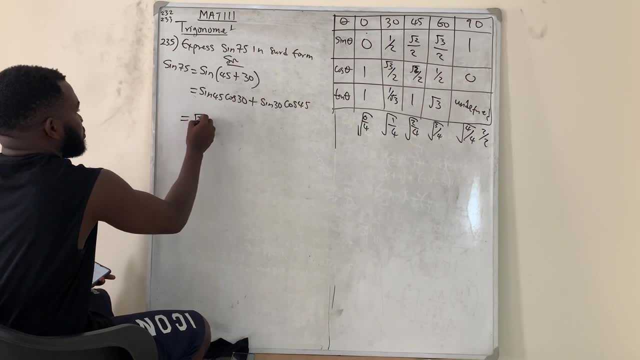 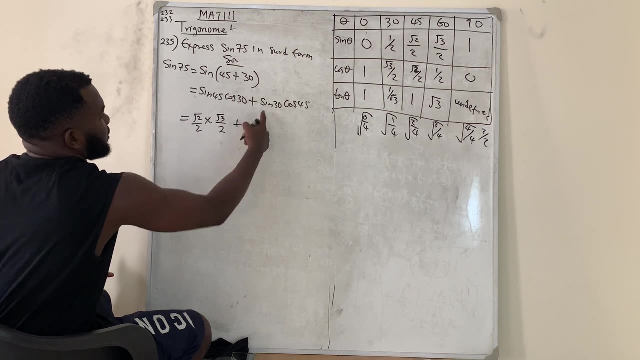 so therefore, sine 45, sine 45 gave us root 2 over 2 times cos 30. cos 30 gave us root 3 over 2, plus sine 30 is 1 over 2 times cos 45, root 2 over 2. so i'm left with this time, this: 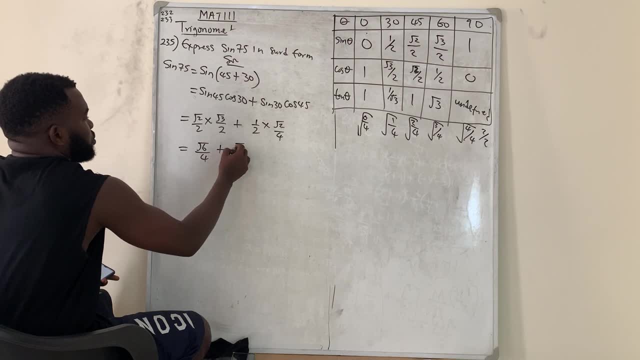 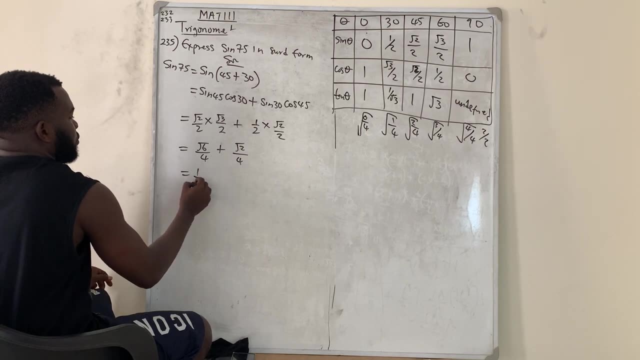 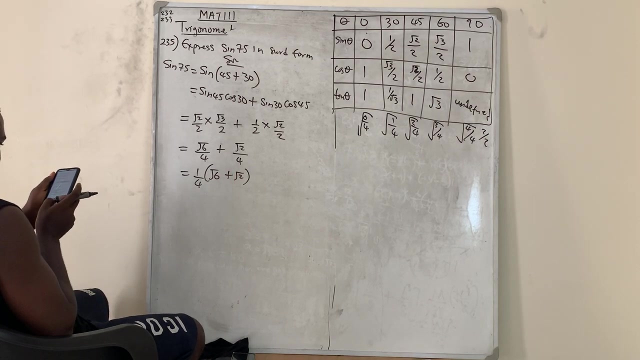 will give you root 6 over 4 plus root 2 over. how did i get, sorry, root 2 over 2, so over 4. so my answer is now 1 over 4 in bracket of root 6, plus what root 2. so it depends on what you have in the 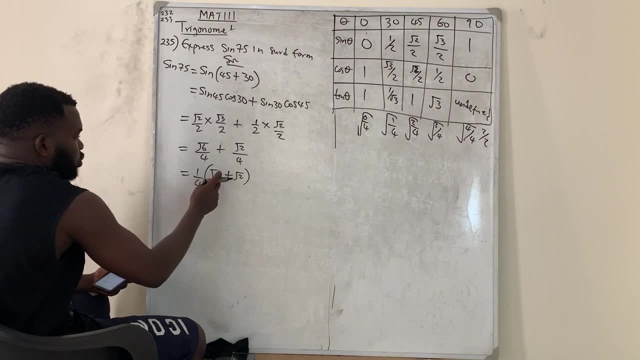 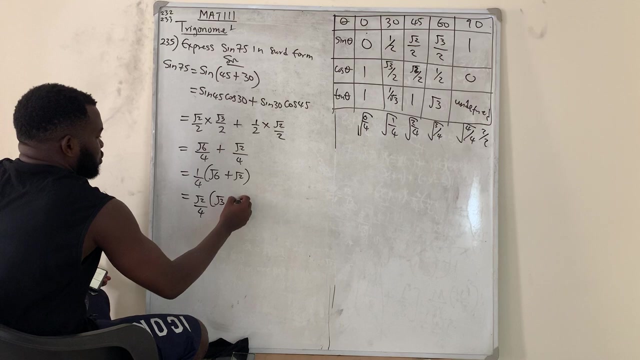 option. that is what will tell you what to do, okay. okay, they decided to bring out root 2, to bring out root 2, to bring out root 2 over 4, even from here itself, to bring out root 2, root 2 over 4. i'll be left inside there as root 3 plus 1. so this is the the answer in the option. so we 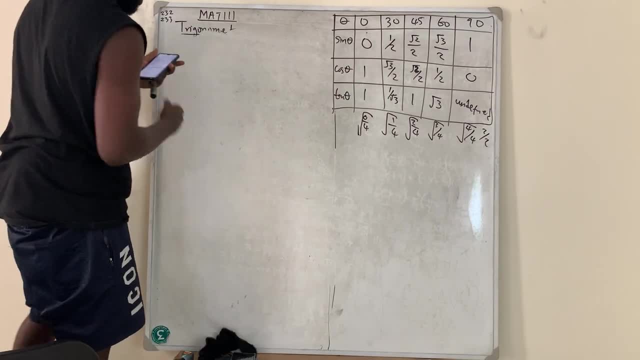 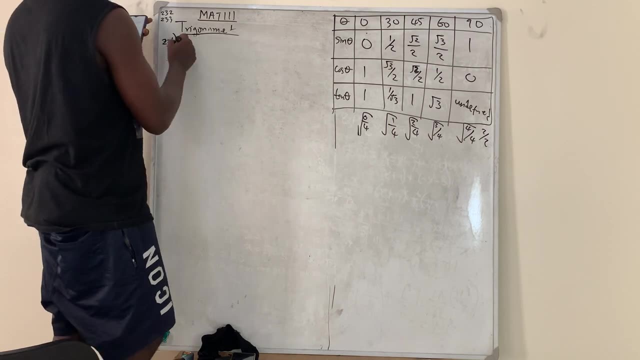 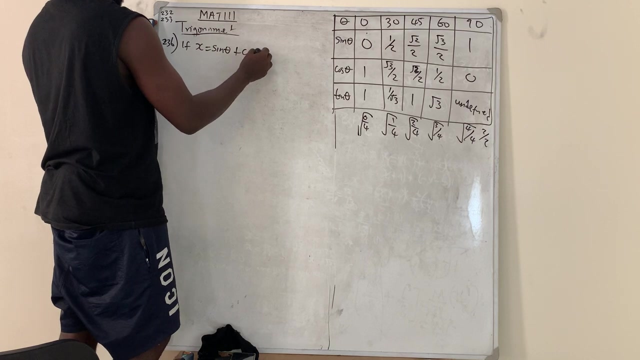 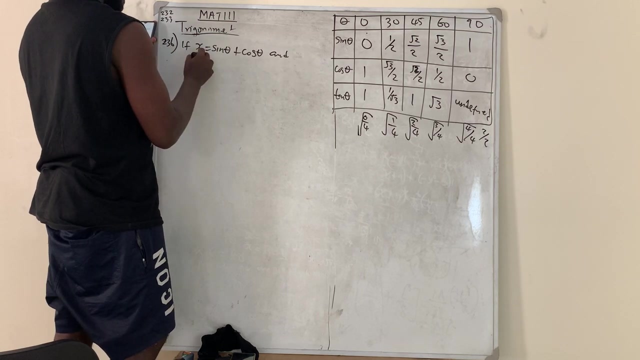 move to the next question. we move to the next question. that question is question number two three, six. question number two three. she said that if x is equal to sine theta, sine theta plus cos theta, okay, sine theta plus cos theta, and and and y is equal to sine theta minus cos theta. 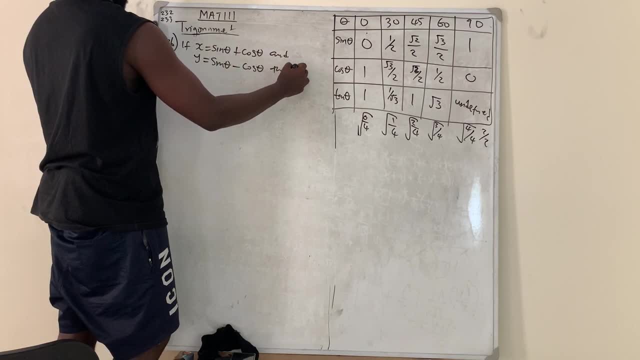 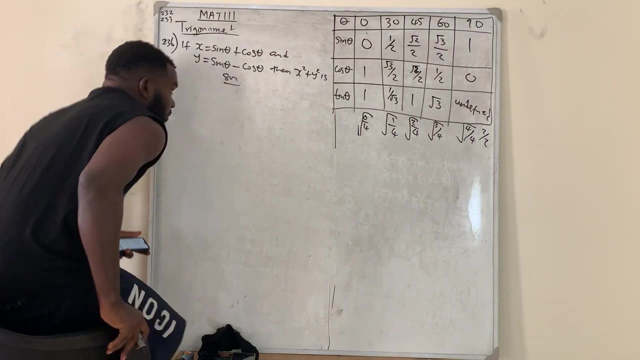 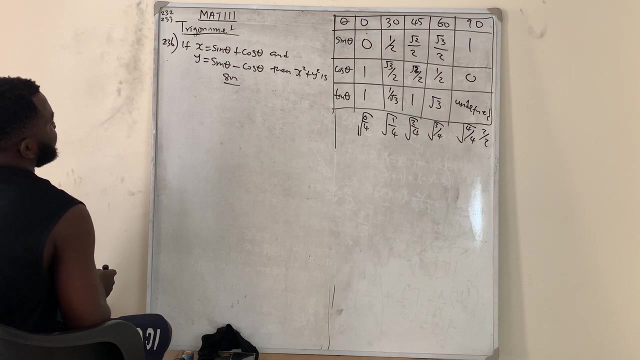 then i'll say: then then x squared plus y squared is okay solution. they need to find s squared plus y squared, all right, um, okay, s squared plus y squared will give us, um, what am i seeing? okay, so here in depth, so i'm going to have that. s squared plus y squared simply means 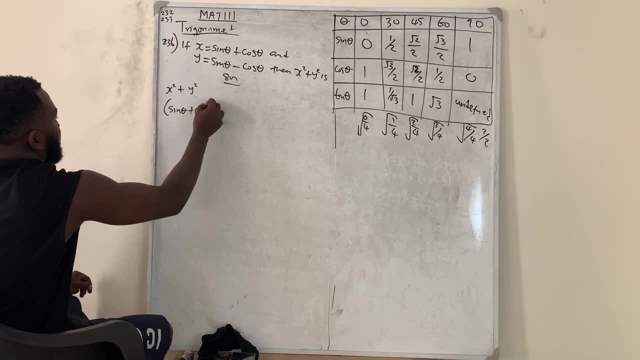 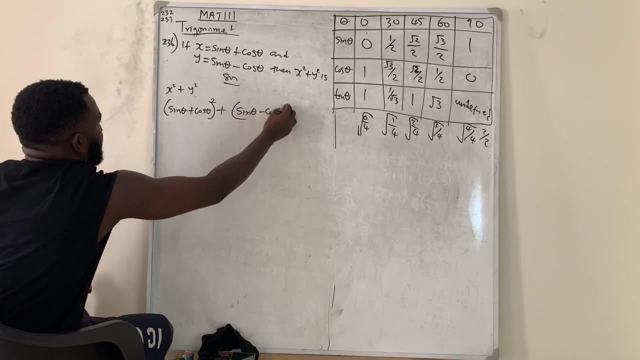 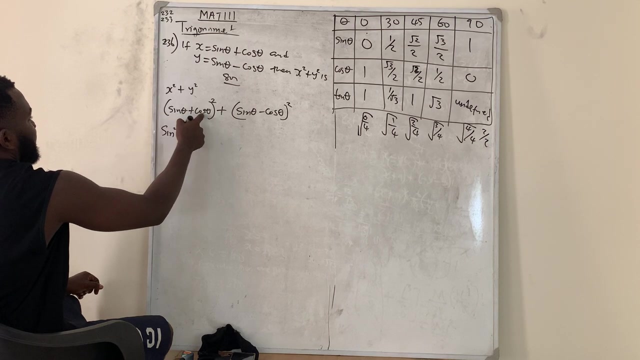 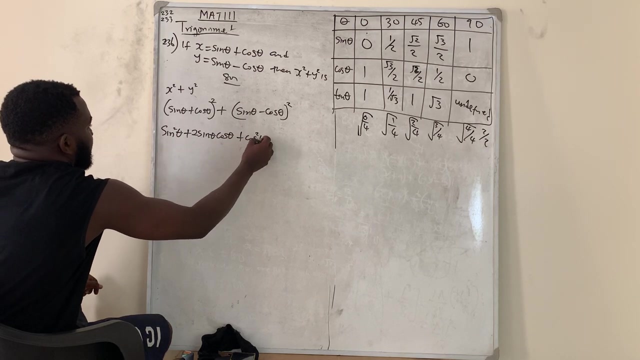 sine theta plus cos theta all squared, plus sine theta, minus cos theta all squared. so let me open the bracket. square the first one sine squared theta. this is vinegar. first one: multiply the second one, double it. two sine theta cos theta. square the last one plus cos squared theta. do the same thing here, plus square the first one sine squared theta, multiply the. 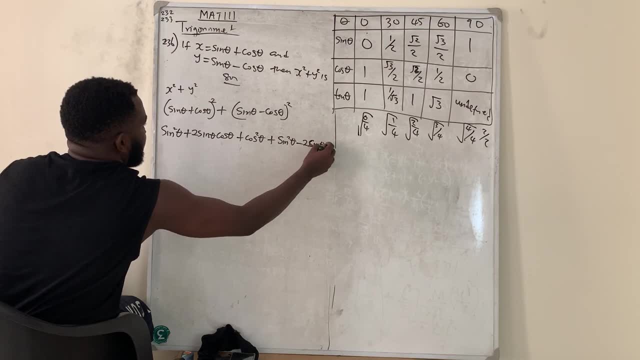 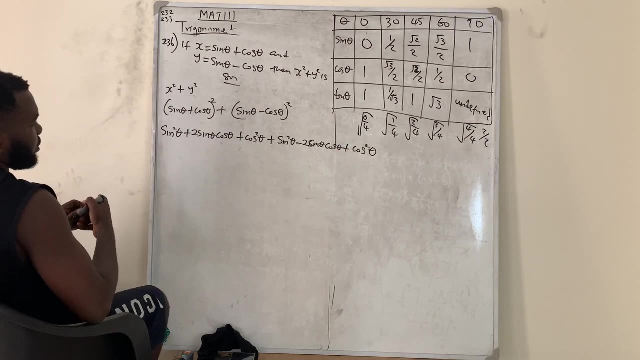 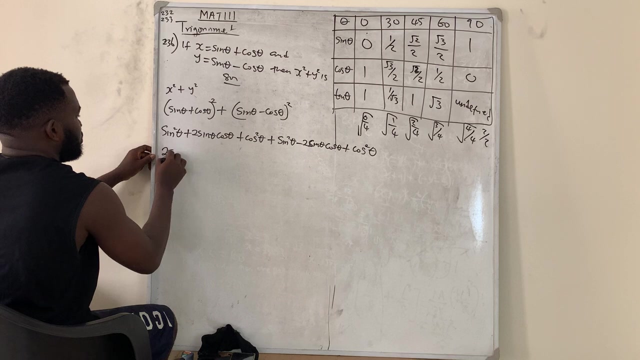 first one and second one. double it minus two sine theta cos theta. then square the last one, you have a plus cos squared theta. so if you look at this, you're going to see that this and this is opposite each other. they are gone, so i'm left with this plus. this will give you two sine squared theta. 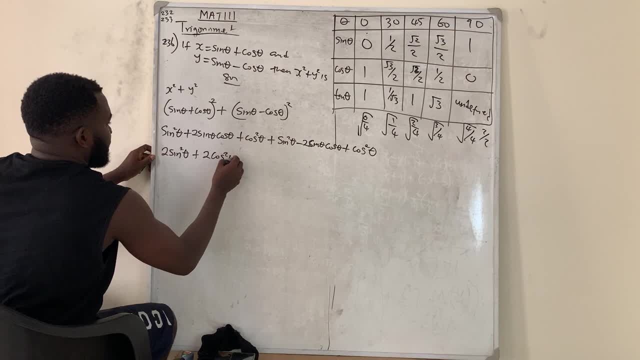 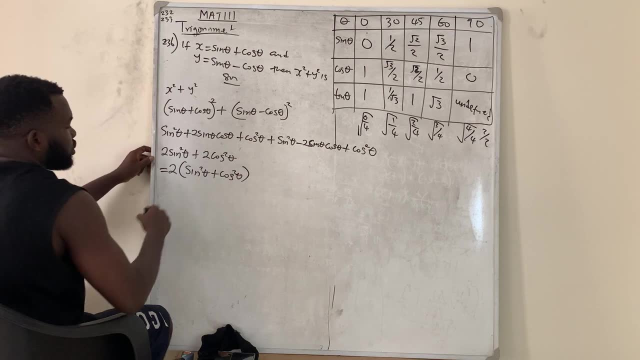 plus this, plus this will give you two cos squared theta. so if you look at this, you're going to see two in bracket of sine squared theta plus cos squared theta and according to three volumetric sine squared theta plus cos squared is equal to one. so this is two in bracket of one. 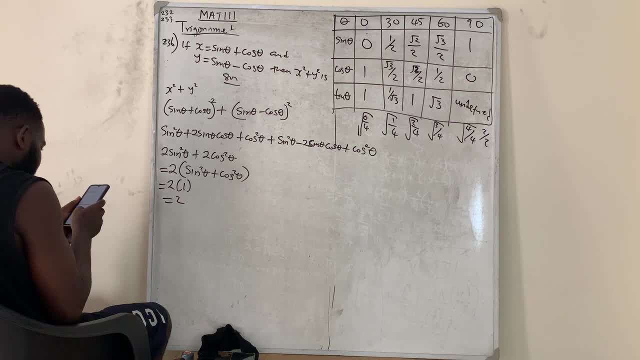 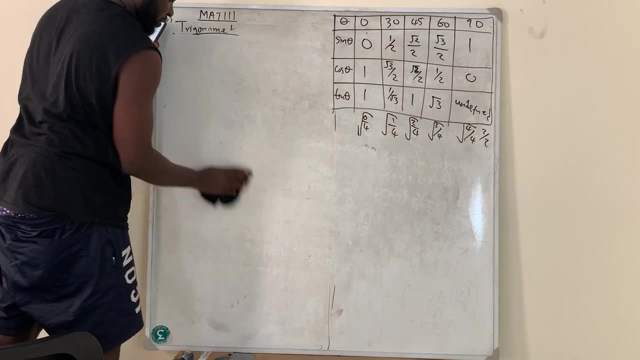 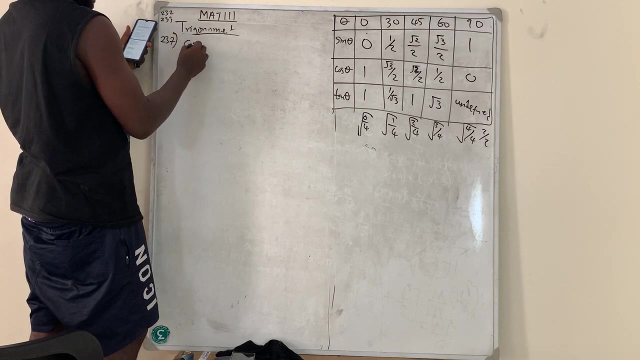 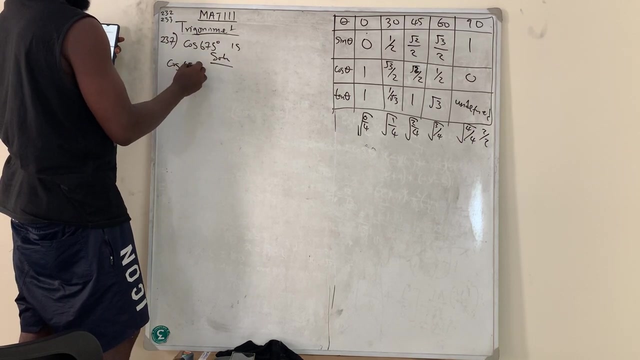 which is two. so my answer here is two right. we move to the next question, question number two: three, seven right. question number two: three, seven. question number two: three, seven said that cos six, seven, five degrees is solution now, whenever you have cos six, seven, five degrees now. 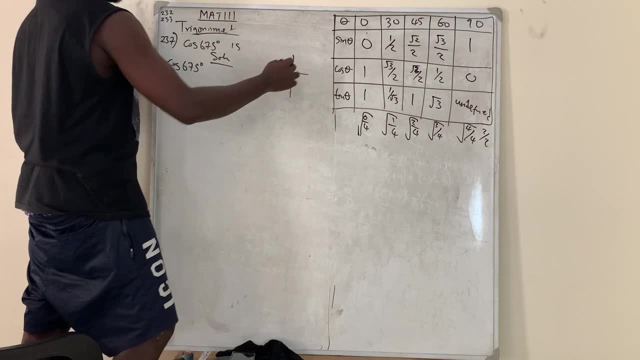 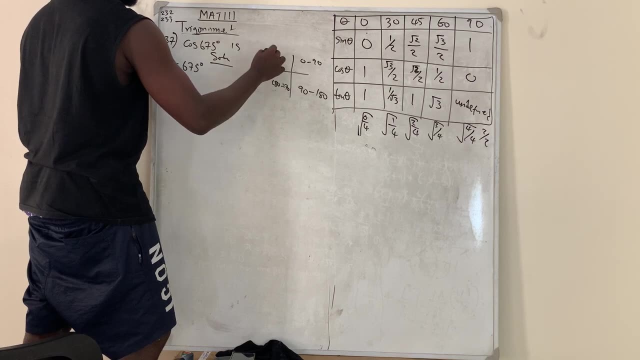 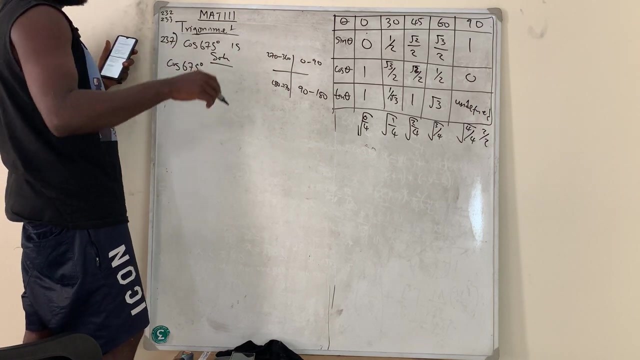 the only thing. we have four quadrants. and my fourth quadrant is what? from zero to ninety, from ninety to one eighty, from one eighty to two seventy, then 270 to 360.. now, anytime they give you an angle that is bigger than the quadrant, just keep subtracting 360 until it will naturally fall into a quadrant. so i'm going to say that. 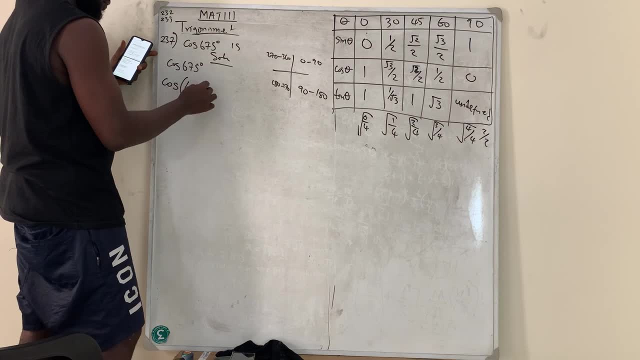 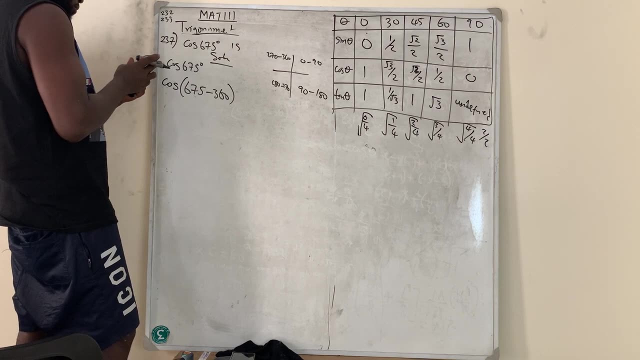 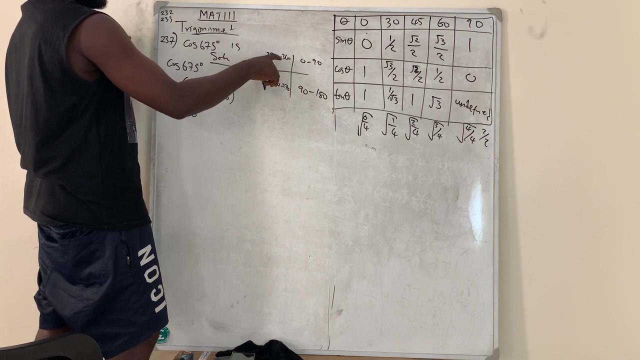 cos, because this is definitely saying cos six, seven, five minus 360.. so what do we have? because subtracting 360 does not change anything at all. okay, so you have them. six, seven, five. okay, minus 360. so i have cos: three, one, five. now, if you look at three, one five has fell in what? in the fourth quadrant? 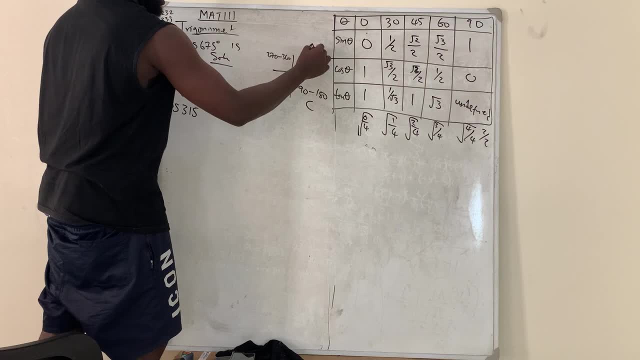 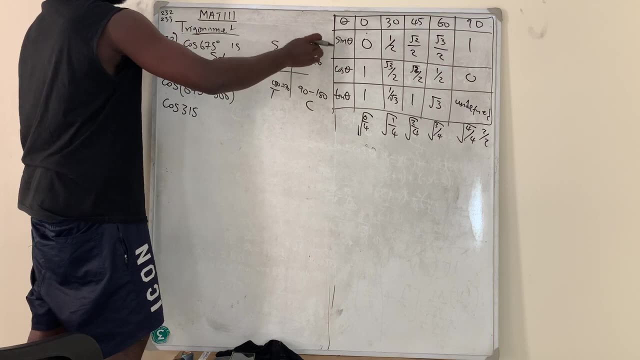 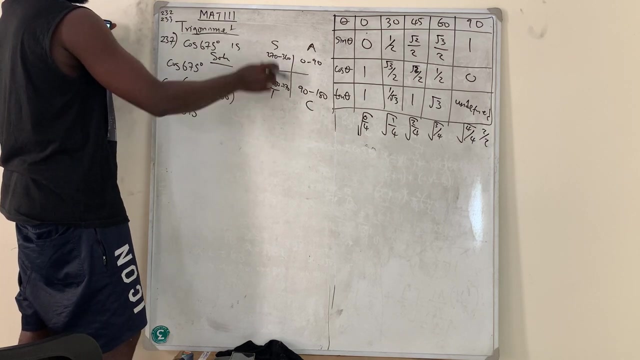 three, one, five is in the fourth quarter. so do your cast. c, a, s, t. so don't forget that why i'm doing the cast. cast means that in the first quadrant only everybody is positive, all it is, all. all is positive. in the second quadrant, only cost is positive. in the third quadrant, only time and 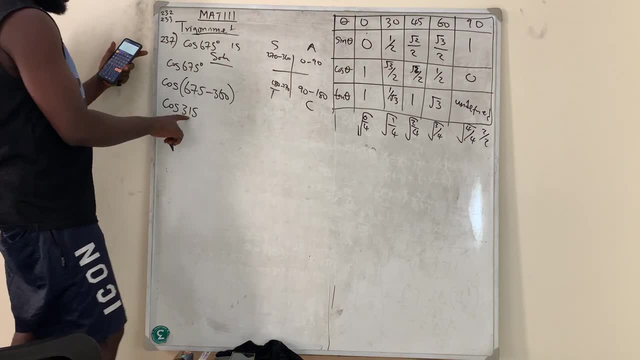 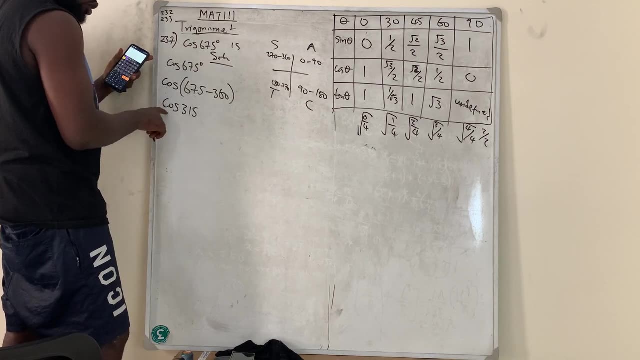 then in the fourth quadrant only uh cost. so if you come to this place now, only sign. so if you know that since cost is in the distance, in the angle, is in the fourth quadrant, so cost is going to be negative, so it's going to be. this is equal to negative cost. in the fourth quadrant we do 360. 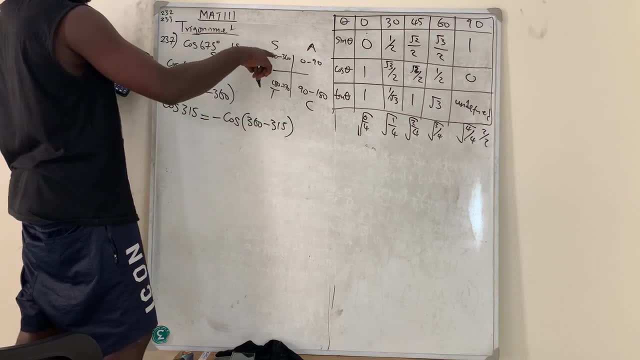 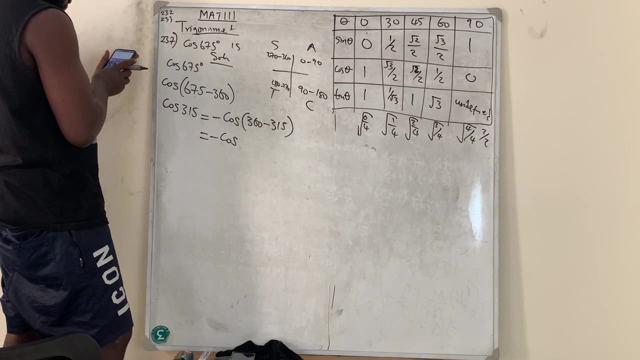 minus that, theta 315.. so this negative is because it's in the fourth quadrant, so i'm having minus cost. so you have them. so plus 45. so which is what? don't forget that plus 45 is a root, 2 over 2, which. 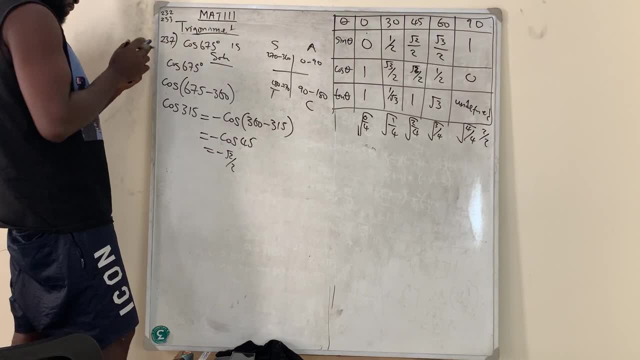 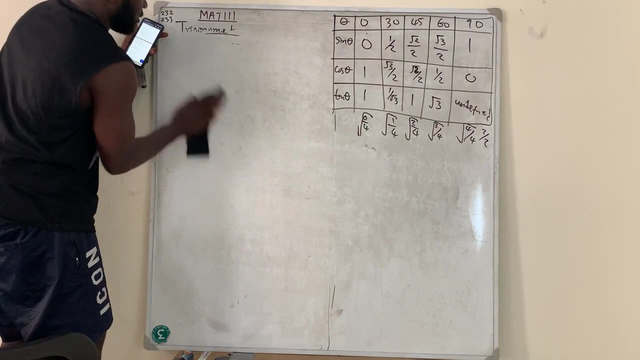 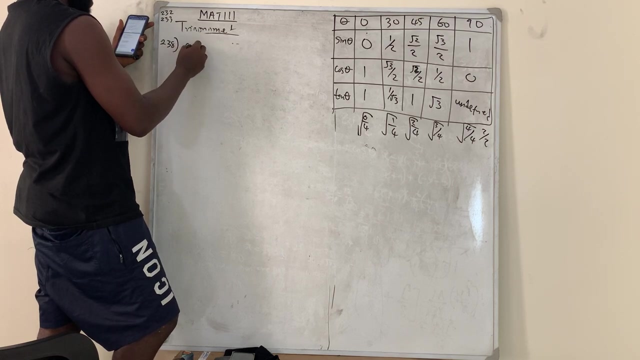 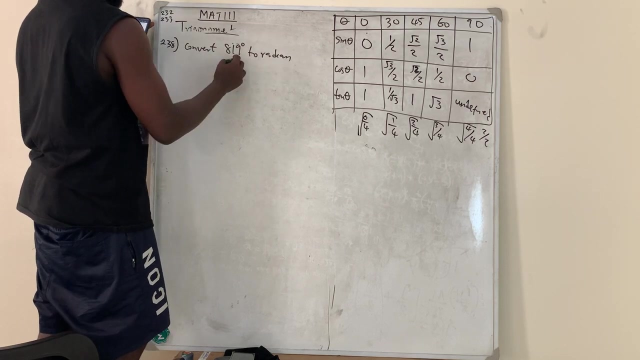 root 2 over 2. so that is the answer there, minus root 2 over 2. okay, so we move to the next question. so from the next question, the next question here said two, three, eight. then i say: convert, convert eight, one, nine degrees to radian. okay solution. so you: 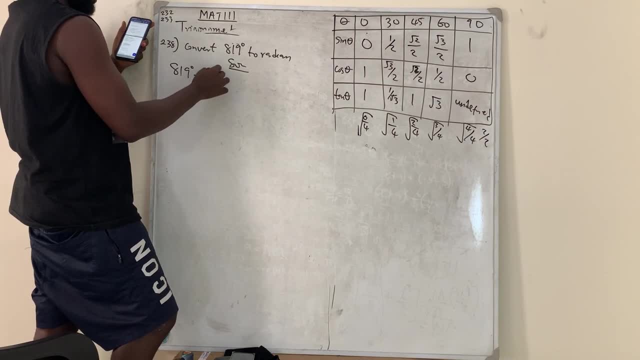 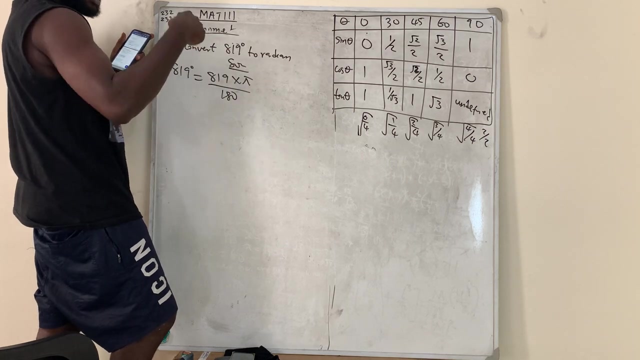 are going to say eight, one nine degrees, the same thing as saying eight one nine times pi divided by one, eight. very simple radian means it must carry pi. so since i'm timesing with pi, i'm going to divide by 180, because pi means 180. so 180, 180 has cancelled out, but since my answer must carry pi, 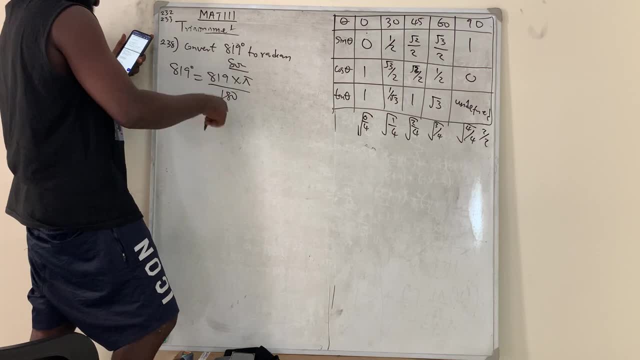 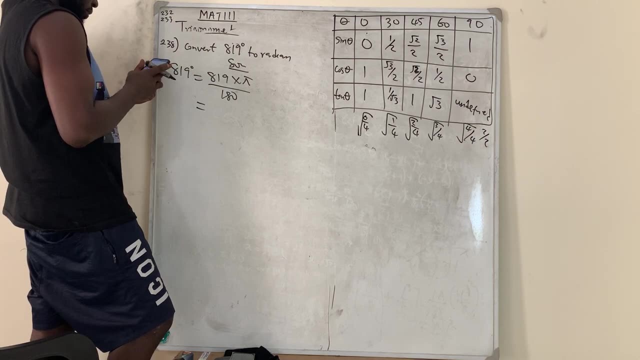 that's why i'm dividing with one eight. so what do you do? just keep reducing these two to the lowest. then you have gotten your answer very simple. so eight one nine divided by one eight. so how do i put my answer in fraction um eight one nine, one eight. 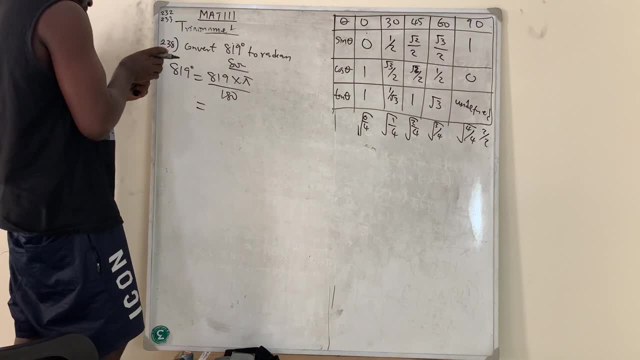 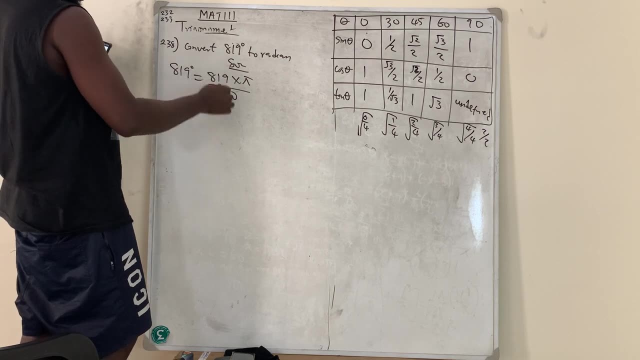 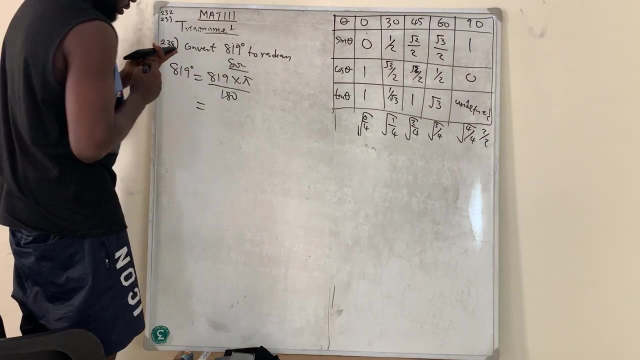 okay, i'm thinking of how to convert. i don't know how this calculator works, so do it yourself. just reduce these two to the lowest. okay, you can find something that can divide them and reduce it to the lowest. then you are done with that particular and then put your. 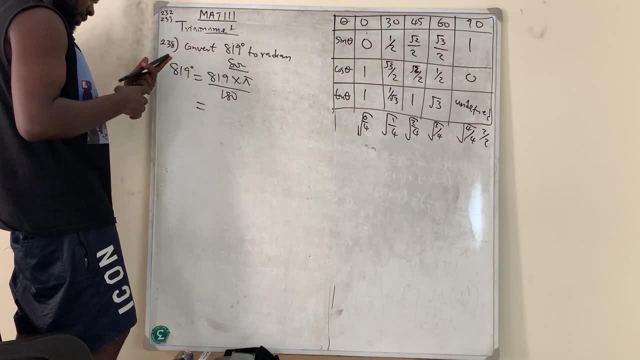 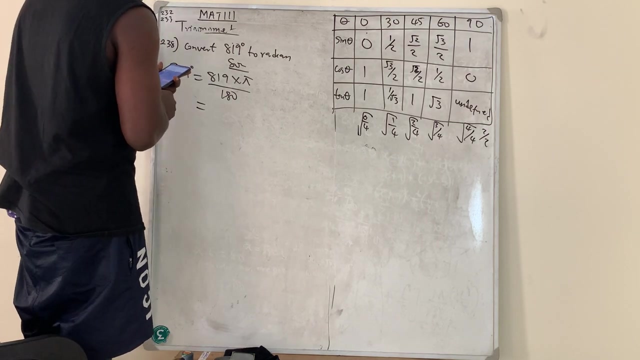 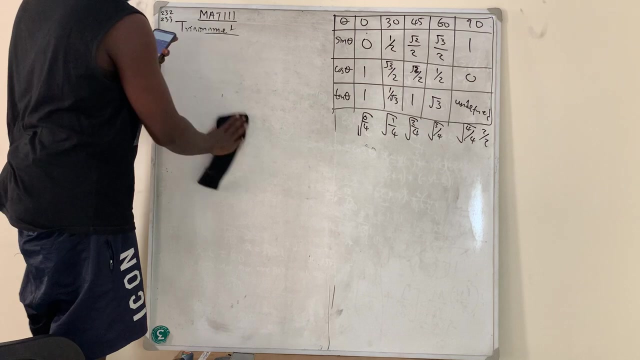 pie, all right. so i can't find where to convert this to: okay, i think i've seen it. this sorry one eight shift. okay, it's not working, so let's leave it. so what do you do? just reduce it to the lowest. so that is that. so we'll go to the next question, question number um. 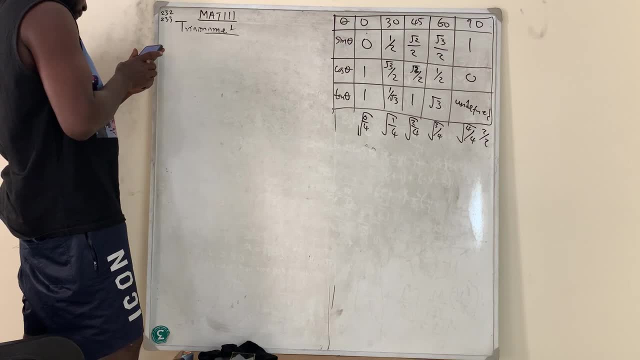 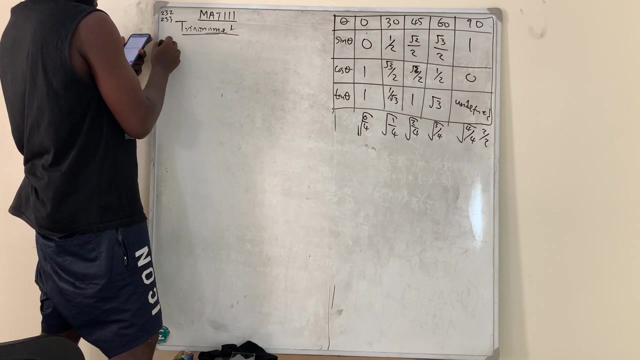 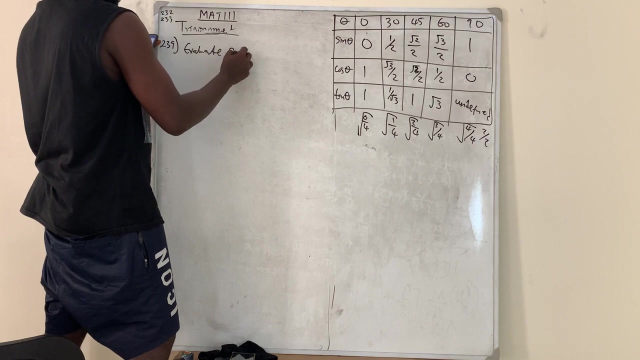 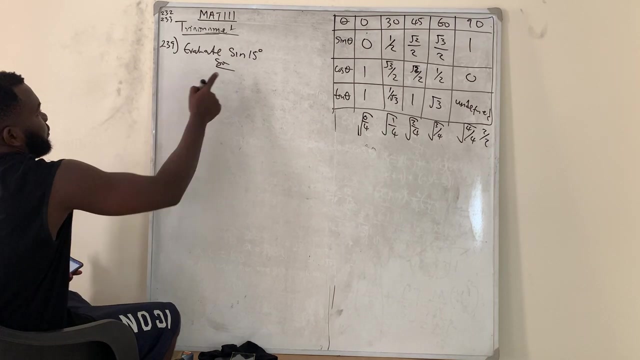 okay, questioniam. sorry about that. this calculator is just making me confused. so question number two, three nine: question number two three nine said evaluateoloIDS sine 15 degrees. all right, solution. this is very, very simple. now the two trigonometric function that will give you 15 is 45 minus 30. so sine 15. 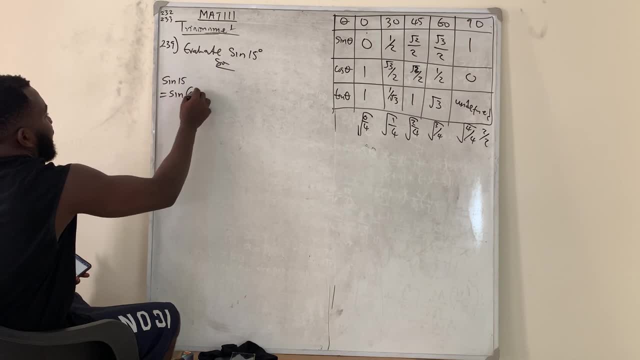 is the same thing as saying sine 45 minus 30. so which is what sine 45 cos 30 minus sine 30 cos 45? so, according to my trigonometric ratio, sine 45 is root 2 over 2 times sine 30 is root 3 over 2. 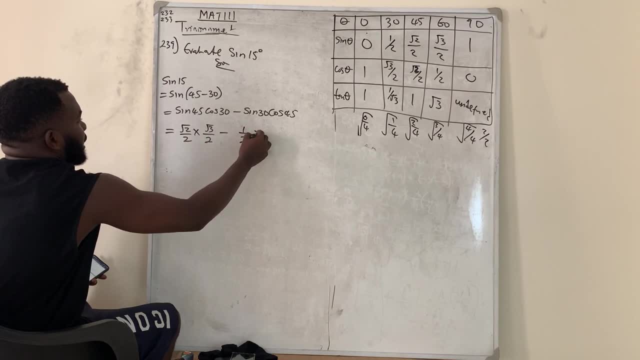 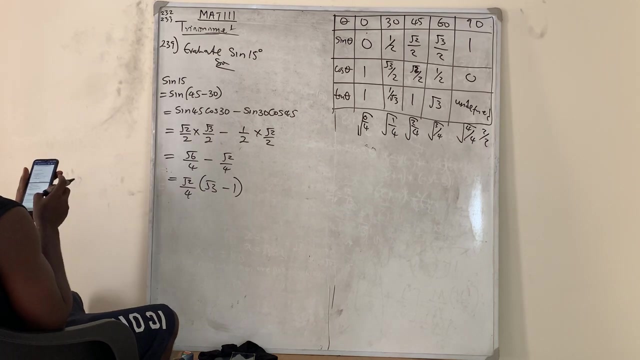 minus this one is 1 over 2, then times root 2 over 2, so i'm having a root 6 over 4 minus root 2 over 4, which will give you root 2 over 4 into root 3 minus 1. so that is the answer for that. so we move. 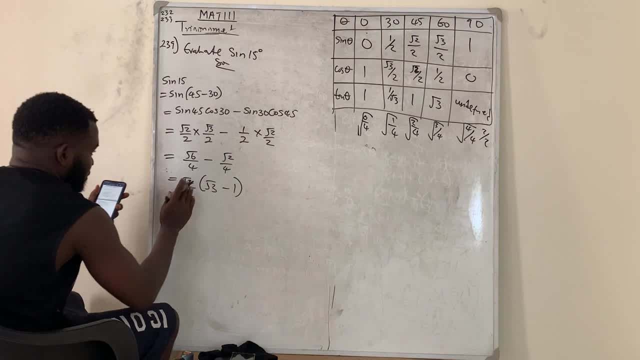 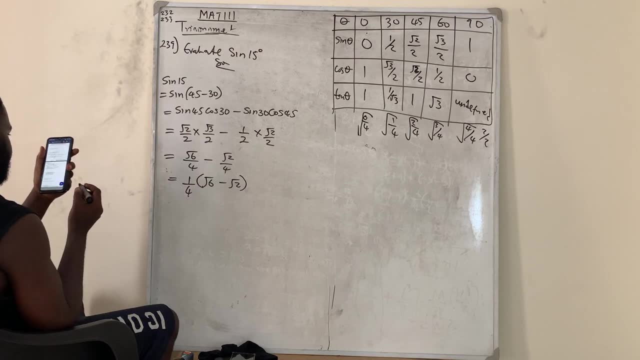 to the next question, which is question or. okay, this one is not there. what is there is that 1 over 4 is what they decided to bring out with 6 minus root 2, so this particular one is the option a. so we move to the next question, question number 240. 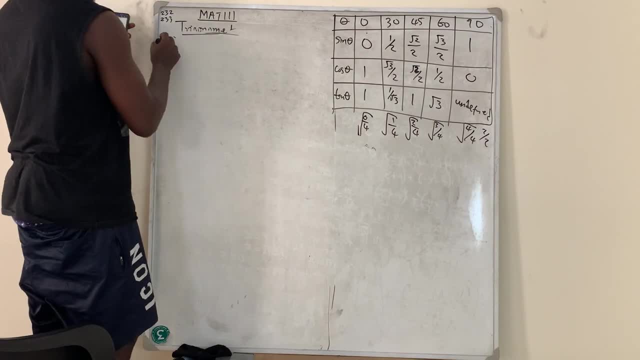 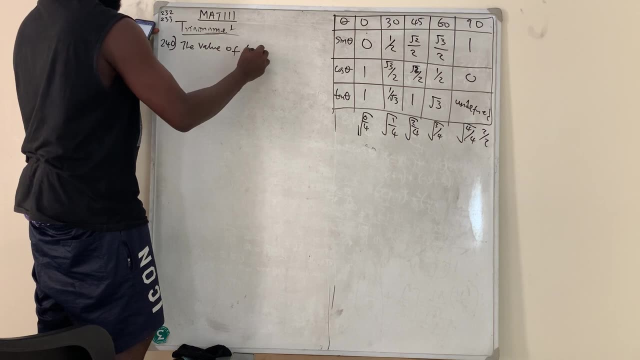 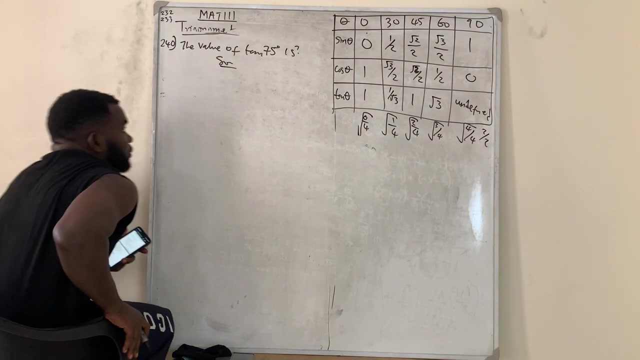 and question number 240 said um the value. the value of tan 75 is okay. solution now for tan. you should know that tan 75, the two numbers for 75, is a. you should know that tan 75, the two numbers for 75, is a. 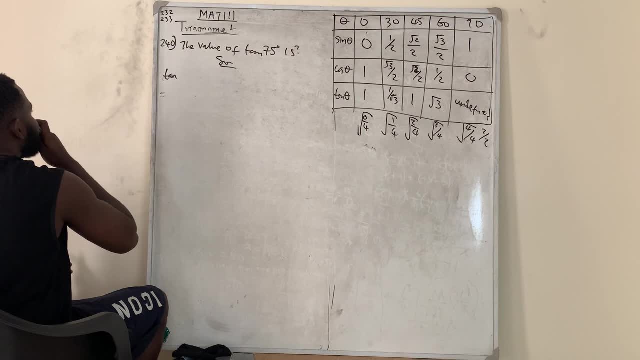 45 and 30 again. okay, so i'm going to have that. this is um 45 and 30 again. okay, so i'm going to have that. this is um 45 and 30 again. okay, so i'm going to have that. this is um sine 45 plus 30. sorry, 45 plus 30. 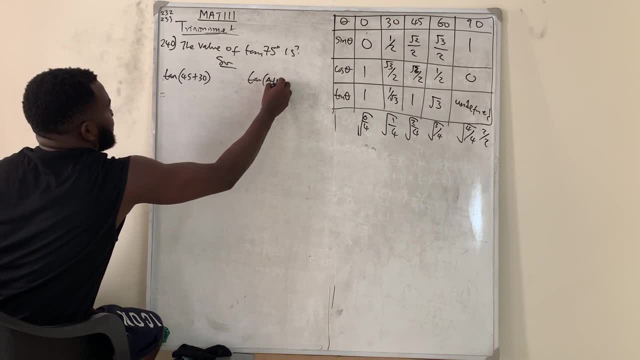 sine 45 plus 30, sorry, 45 plus 30, sorry, 45 plus 30. sine 45 plus 30, sorry, 45 plus 30, so, but don't forget that. tan a plus b: so, but don't forget that. tan a plus b, so, but don't forget that tan a plus b is something that's saying tan a. 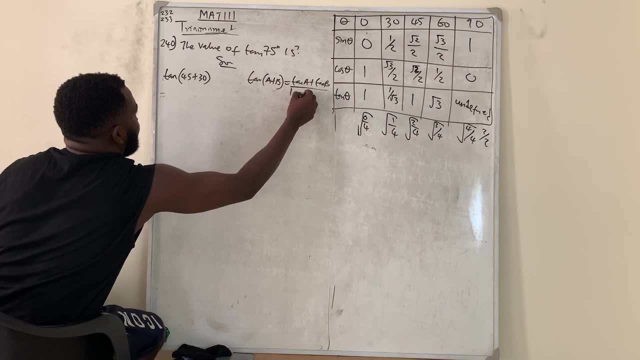 is something that's saying tan a is something that's saying tan a plus tan b. okay, all over one minus tan plus tan b. okay, all over one minus tan plus tan b. okay, all over one minus tan a- tan d- okay. so this is equal to what. 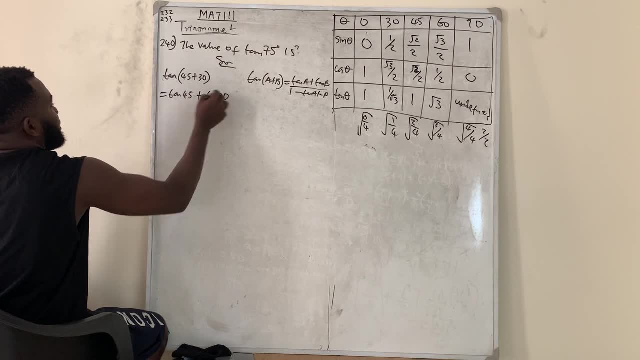 a tan d? okay, so this is equal to what a tan d okay, so this is equal to what tan 45 plus tan 30 all over tan 45 plus tan 30 all over one minus tan 45, one minus tan 45 than 30. so you can watch my video on. 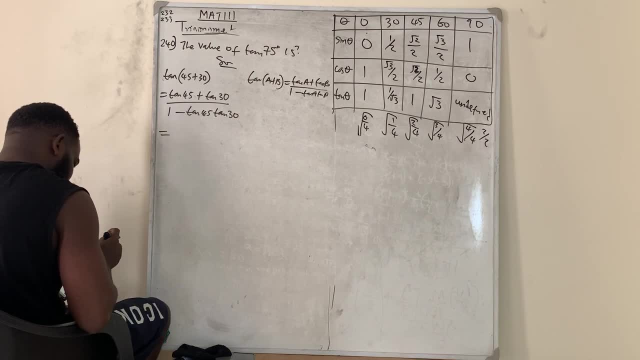 than 30, so you can watch my video on than 30, so you can watch my video on trigonometry. okay, i'll drop the link at trigonometry. okay, i'll drop the link at trigonometry. okay, i'll drop the link at the description. 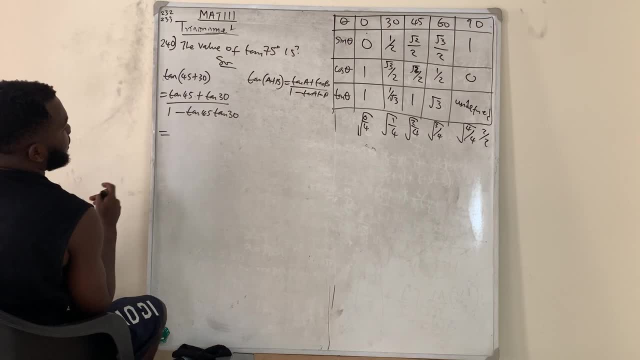 the description, the description, so you understand better. you understand, so you understand better, you understand, so you understand better. you understand that formula, so the next one is that formula, so the next one is that formula, so the next one is now: substitute everybody. tan 45 is one. 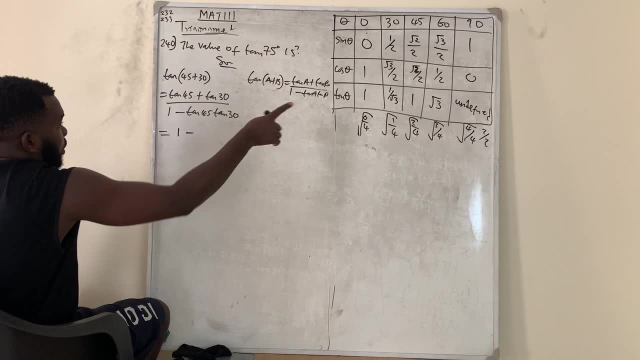 now substitute everybody. tan 45 is one. now substitute everybody. tan 45 is one minus tan 30 is a root three over three minus tan 30 is a root three over three minus tan 30 is a root three over three. one over root three means root three over. 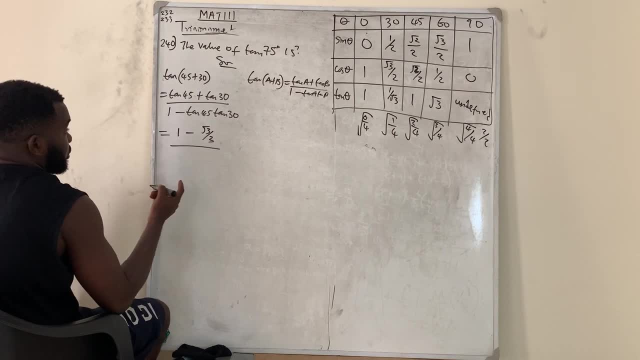 one over root three means root three over one over root three means root three over three. so root three over three all over three. so root three over three all over three. so root three over three all over. according to rationalization. so this is according to rationalization. so this is. 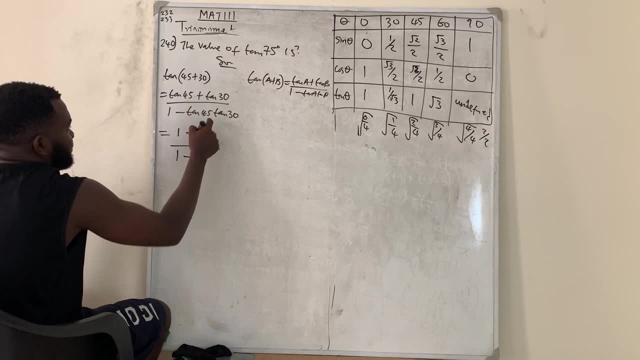 according to rationalization. so this is one. minus tan 45 is one times one. minus tan 45 is one times one. minus tan 45 is one times uh. tan 30 is a root three over three. uh. tan 30 is a root three over three. 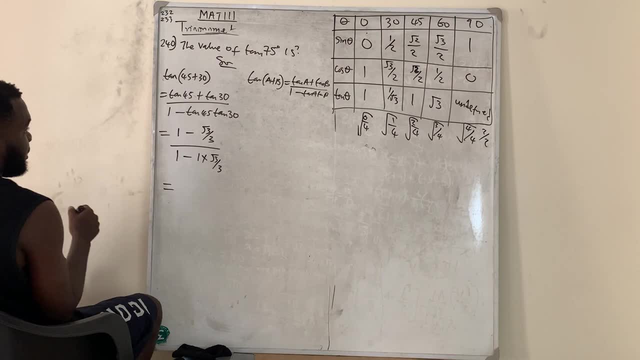 uh, tan 30 is a root three over three. okay, so i'm left with um. okay, so i'm left with um. okay, so i'm left with um. so this is plus. i'm left with lcm, lcm. so this is plus. i'm left with lcm, lcm. 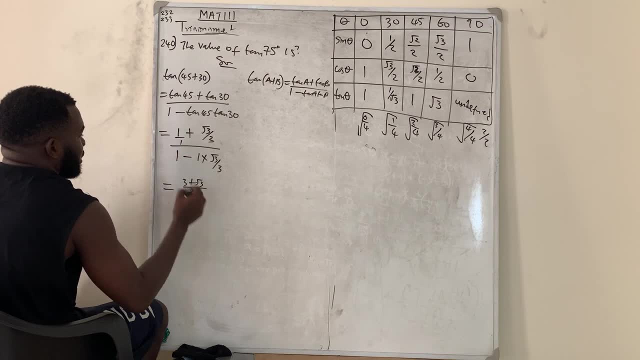 so this is plus. i'm left with lcm. lcm- there is three, so i have them three plus there is three, so i have them three plus there is three, so i have them three plus root three, okay, divided by do this one: root three: okay, divided by do this one. 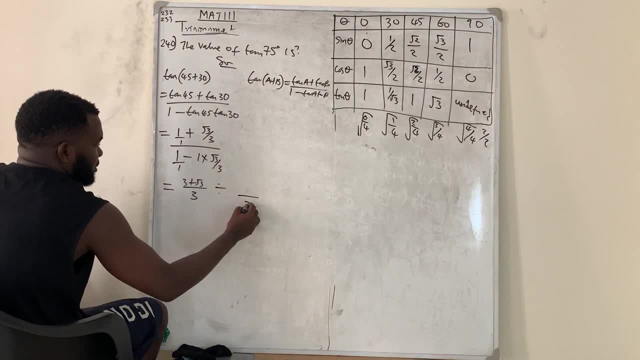 root three. okay, divided by: do this one again by lcm- lcm- anything times one again by lcm- lcm- anything times one again by lcm- lcm- anything times one sentence. so lcm is three. so i have three sentence. so lcm is three. so i have three sentence. so lcm is three. so i have three minus root three. so you are having that. 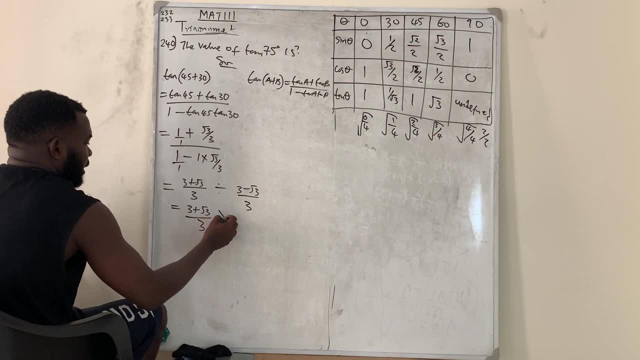 minus root three. so you are having that minus root three. so you are having that three plus root three, three plus root three. three plus root three over three times three over three minus over three times three over three minus over three times three over three minus root three. so if this comes to this, i am 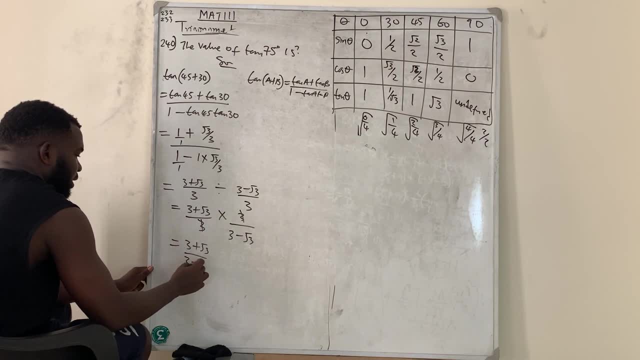 root three. so if this comes to this, i am root three. so if this comes to this, i am left with three plus root three all over left with three plus root three, all over left with three plus root three all over three minus root three. so if the answer 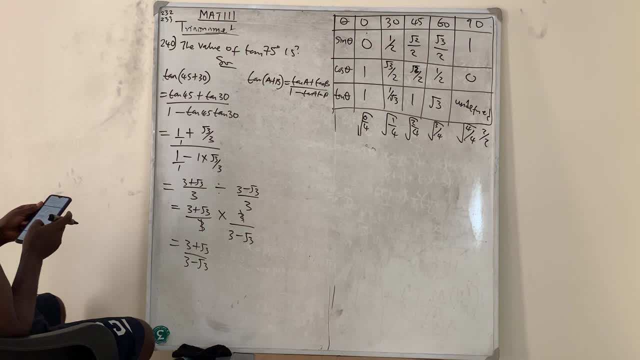 three minus root three. so if the answer three minus root three. so if the answer is not there, then we need to rationalize. is not there, then we need to rationalize. is not there, then we need to rationalize. if this answer is not there, then we need. 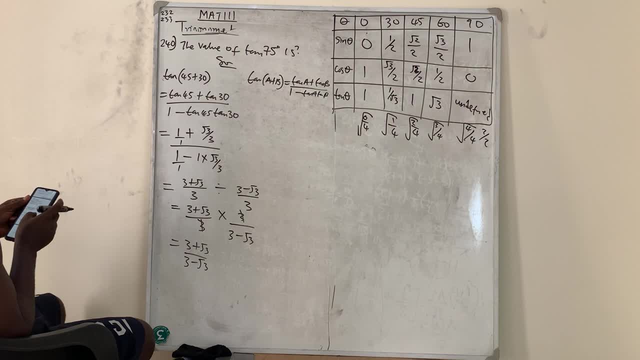 if this answer is not there, then we need- if this answer is not there, then we need to rationalize, to rationalize, to rationalize. okay, so, let us rationalize that. okay, so, let us rationalize that. okay, so, let us rationalize that. if you rationalize this, you're going to 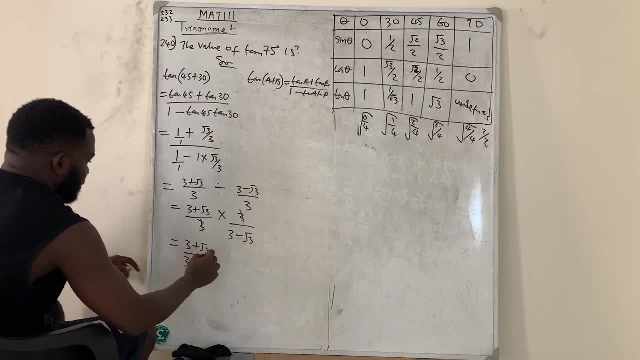 if you rationalize this, you're going to. if you rationalize this, you're going to have have have. if you rationalize this, you're going to. if you rationalize this, you're going to. if you rationalize this, you're going to have times three minus root three. 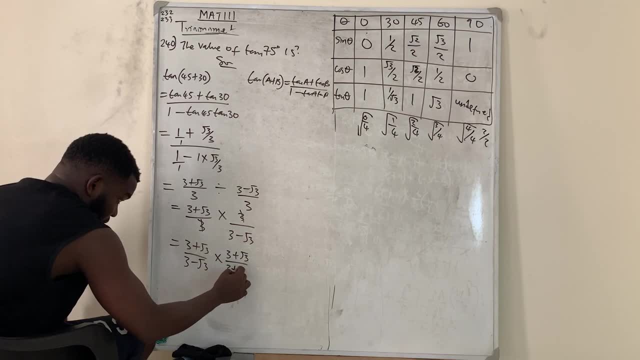 have times three minus root three. have times three minus root three all over sorry three my three plus root all over sorry three my three plus root all over sorry three my three plus root three all over three. three all over three. three all over three plus root three. 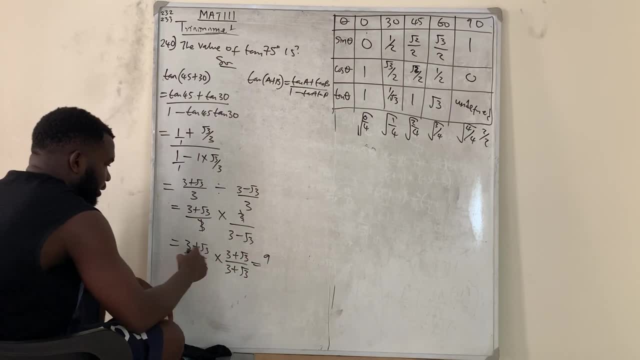 plus root three plus root three. okay, so this is equal to three times okay, so this is equal to three times okay, so this is equal to three times three, three, three, nine, three times. this will give you nine three times. this will give you nine three times. this will give you three roots three with three times this. 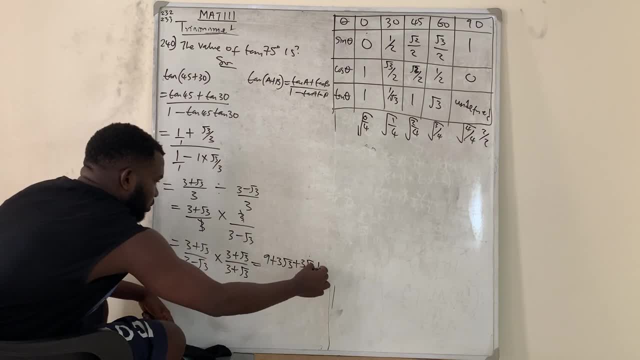 three roots, three with three times this, three roots, three with three times this will give you, will give you will give you three roots, three with three times root, three roots, three with three times root, three roots, three with three times root, three will give you ordinary three, three roots, three with three times root, all over three times three, nine minus. 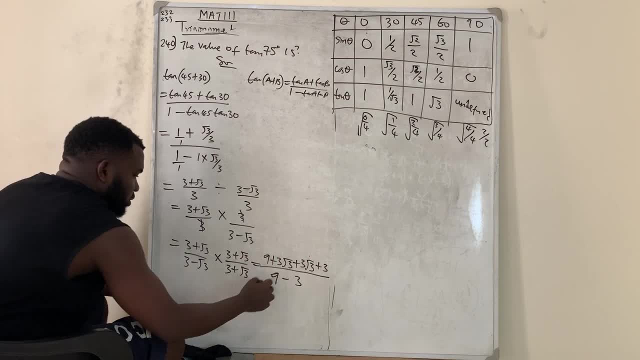 all over three times three, nine minus all over three times three, nine minus root three times three ordinary three. so root three times three ordinary three. so root three times three ordinary three. so i'm left with this plus this will give. i'm left with this plus this will give. 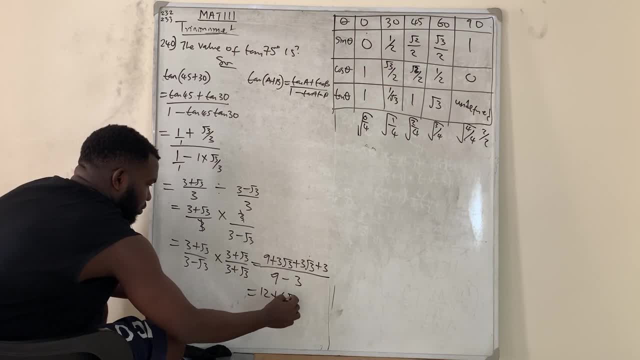 i'm left with this. plus, this will give you twelve this, and this will give you me you twelve this, and this will give you me you twelve this, and this will give you me plus six roots three all over this minus. plus six roots three all over this minus. 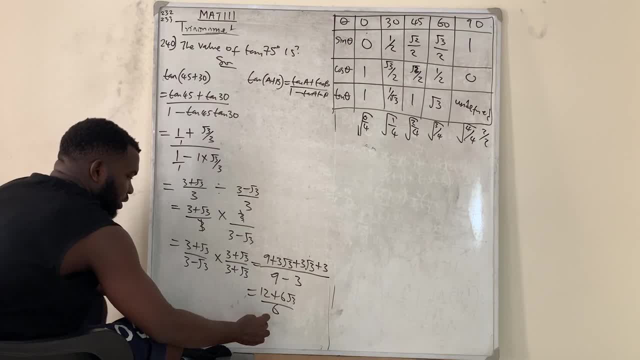 plus six roots three. all over this. minus this is giving me six, so divide. this is giving me six, so divide. this is giving me six, so divide everybody. twelve divided by six will everybody. twelve divided by six, will everybody. twelve divided by six will give you two plus six divided by six. 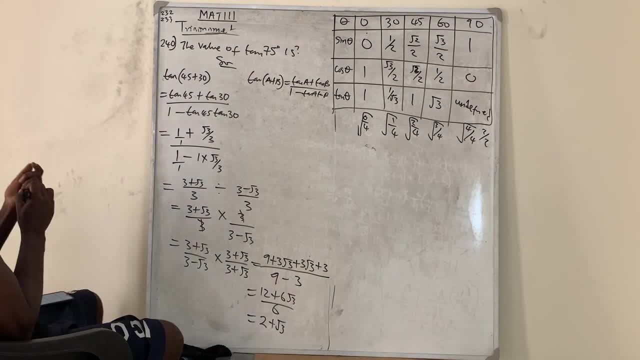 give you two plus six divided by six. give you two plus six divided by six. this will give you one. so i'm left with. this will give you one. so i'm left with. this will give you one. so i'm left with three. so my answer is what? two plus root. 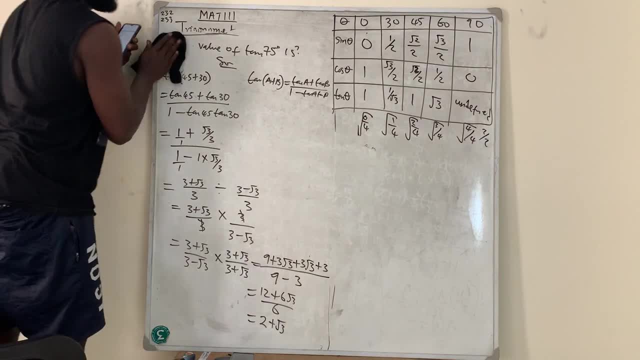 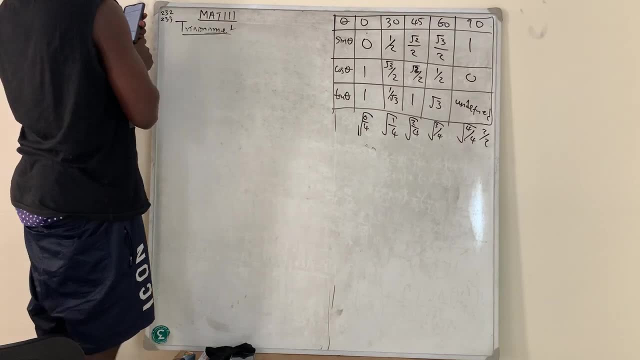 three. so my answer is what two plus root three. so my answer is what two plus root three. so that is the answer there. so we three. so that is the answer there. so we three. so that is the answer there. so we move to the next question. so the next question here said question. 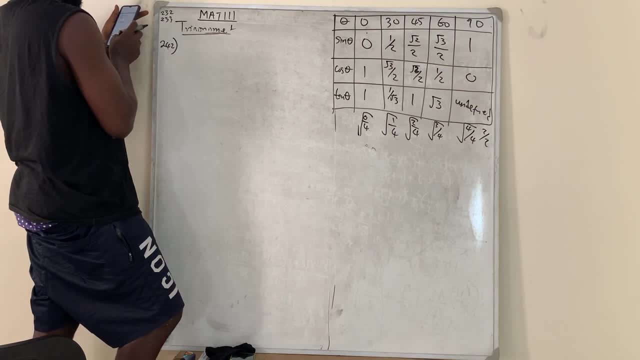 so the next question here said question. so the next question here said question, number, number, number 242. there is no 241, so i have 242, 242, 242. there is no 241, so i have 242, 242, 242. there is no 241, so i have 242, 242, said simplify. 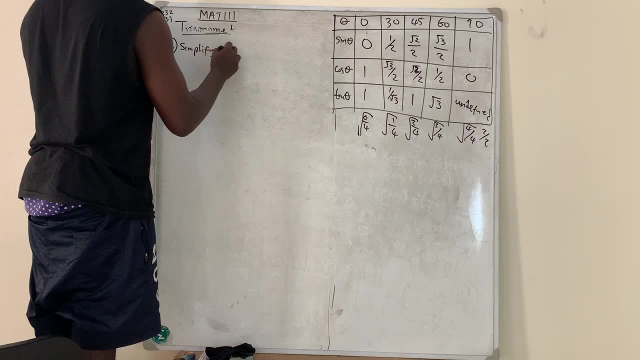 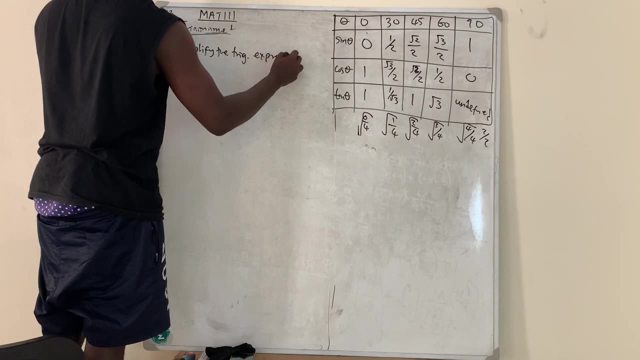 said simplify, said simplify, simplify, simplify said simplify, simplify, simplify the simplify, simplify the simplify, simplify the trigonometry, trigonometry, trigonometry expression, trigonometry expression, tan trigonometry expression, tan, trigonometry expression tan, tan x plus tan x, plus tan x plus cos x. 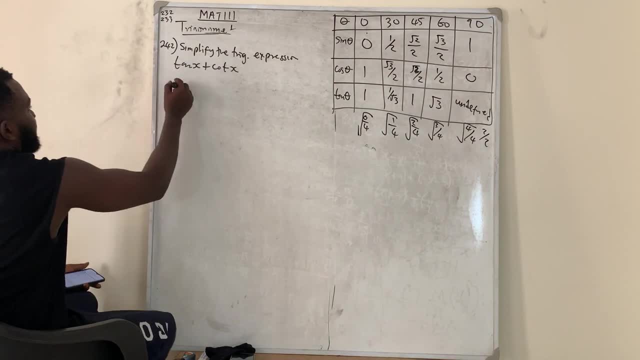 cos x, cos x. okay now, this is very, very simple. what is okay now. this is very, very simple. what is okay now? this is very, very simple. what is tan tan means sine x over what cos x tan tan means sine x over what cos x tan tan means sine x over what cos x plus cot means one, two, three, uh, inverse. plus cot means one, two, three, uh. inverse plus cot means one, two, three, uh. inverse of this one. so inverse of this one, just of this one, so inverse of this one, just of this one, so inverse of this one, just to turn this one around, which is what? 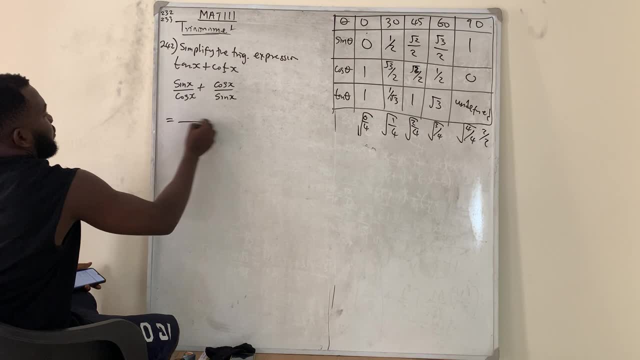 to turn this one around? which is what to turn this one around? which is what cos x over what sine x? so now, if you cos x over what sine x, so now, if you cos x over what sine x, so now, if you find the lcm of this and this, you're. 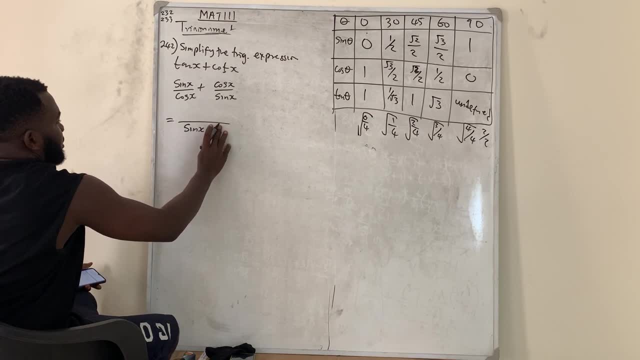 find the lcm of this and this. you're find the lcm of this and this. you're going to have sine x, cos x. going to have sine x, cos x. going to have sine x, cos x, cos x. when these two divide, is you have cos x. when these two divide, is you have. 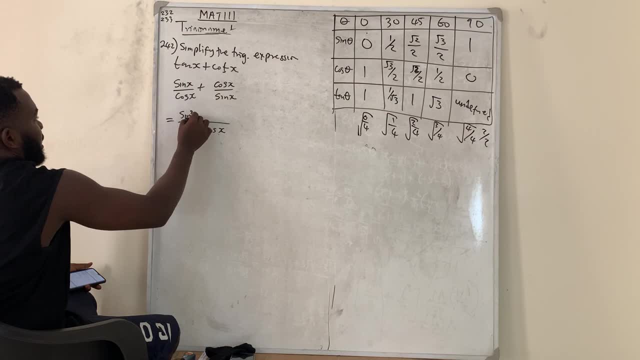 cos x when these two divide is: you have sine s sine s times. so i have what sine sine s sine s times. so i have what sine sine s sine s times. so i have what sine squared x plus when the divide is you squared x plus when the divide is you. 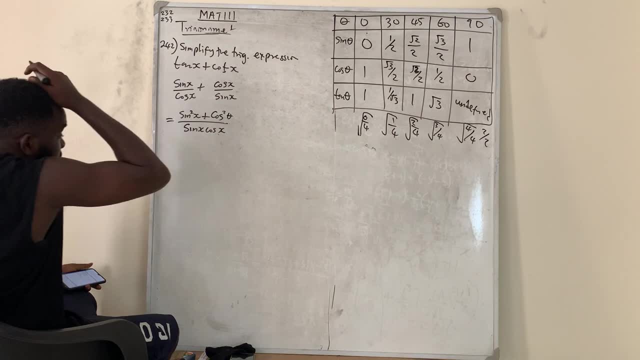 squared x plus when the divide is, you have cos x cos s times. so i have what have cos x cos s times. so i have what have cos x cos s times. so i have what? cos x cos s according to trigonometry. cos x cos s according to trigonometry. 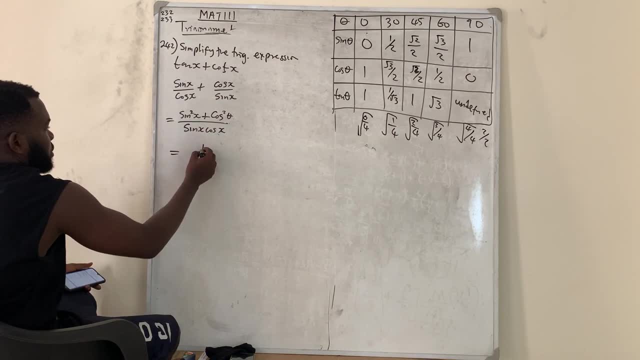 cos x, cos s. according to trigonometry, sine squared s plus cos square s is one. sine squared s plus cos square s is one. sine squared s plus cos square s is one. so my answer is: what one over sine x? so my answer is: what one over sine x? 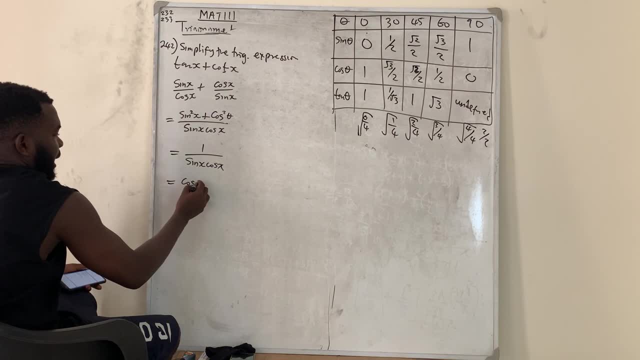 so my answer is what? one over sine x cos x and one over sine means cosec cos x and one over sine means cosec cos x and one over sine means cosec. one over cos means sec, so cosec x, sec x. one over cos means sec, so cosec x, sec x. 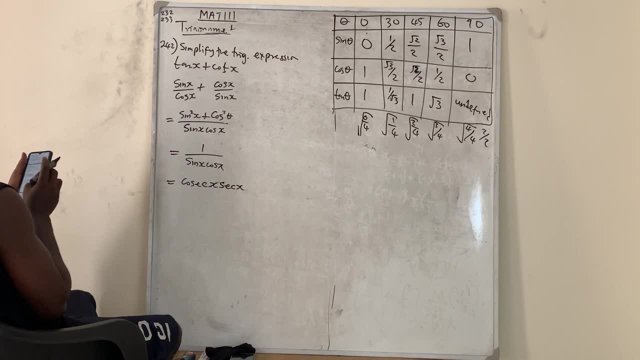 one over. cos means sec? so cosec x, sec x. okay, so that is that cosec x, sec x. okay. so that is that cosec x, sec x. okay, so that is that cosec x, sec x. okay, but this one is not there. okay, but this one is not there. 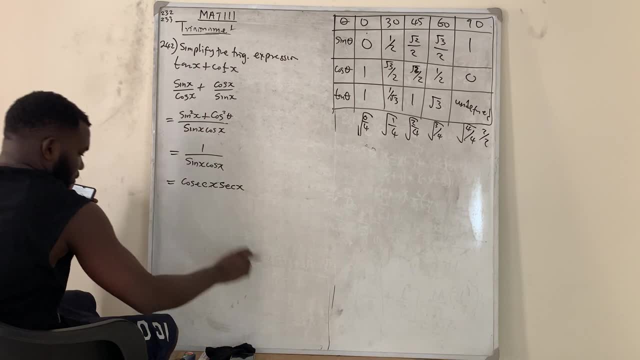 okay, but this one is not there, okay, so they decided to leave this one. so okay, so they decided to leave this one. so okay, so they decided to leave this one. so look at what they did. look at what they did. look at what they did. they want to confuse you. look at what they. 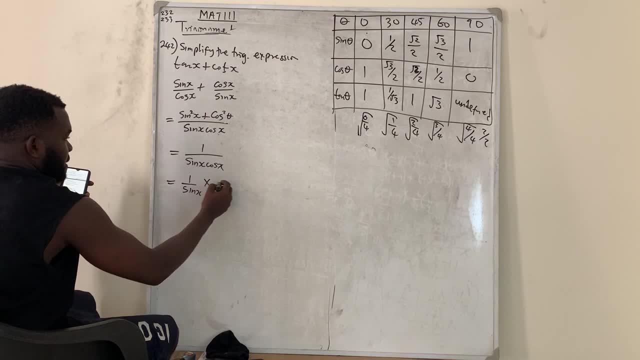 they want to confuse. you look at what they they want to confuse. you look at what they did: one over sine x. you know that did one over sine x. you know that did one over sine x. you know that this is one over sine s all over one over. 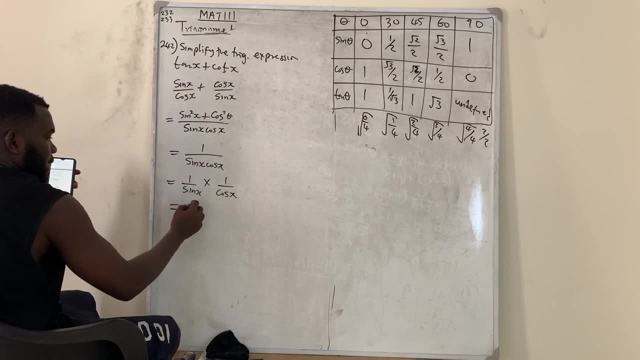 this is one over sine s all over one over. this is one over sine s all over one over cos x all right and one over. they, cos x all right and one over they. cos x, all right and one over. they decided to leave this one the way it is. 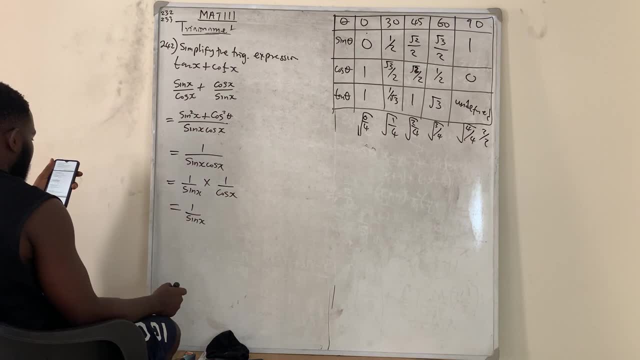 decided to leave this one the way it is, decided to leave this one the way it is. and then one of our course means cosec, and then one of our course means cosec, and then one of our course means cosec and cosec and cosec. 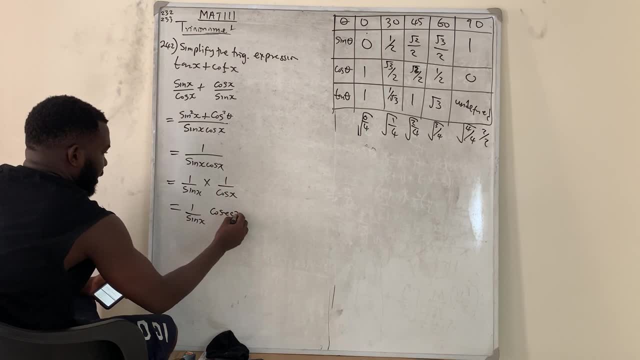 and cosec. we call it csc. so this is what cosec x. we call it csc, so this is what cosec x. we call it csc, so this is what cosec x. so which is what one time this will give. so which is what one time this will give. 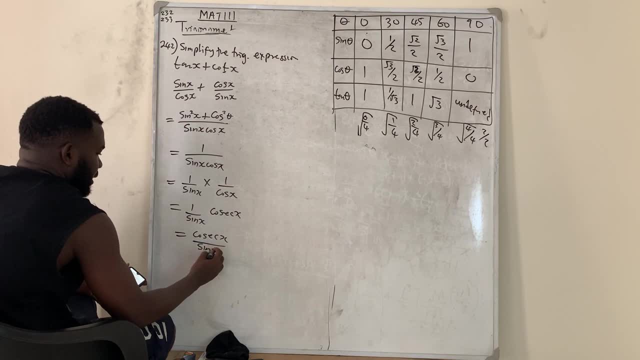 so, which is what one time this will give you cosec x over you, cosec x over you, cosec x over sine x and short form for cosets: we sine x and short form for cosets: we sine x and short form for cosets, we call it csc. 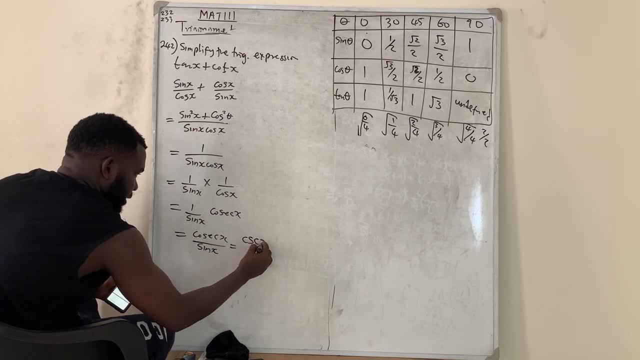 call it csc. call it csc, csc. sorry c, csc, sorry c csc, sorry c. sc x all over what sine x. so this is sc x all over what sine x. so this is sc x all over what sine x. so this is what is in the option there. so option c: 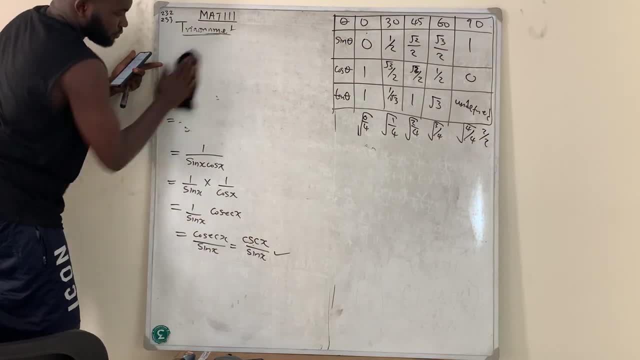 what is in the option there, so option c. what is in the option there, so option c is very, very correct. so go to the next is very, very correct. so go to the next is very, very correct. so go to the next question. so the next question here said question. 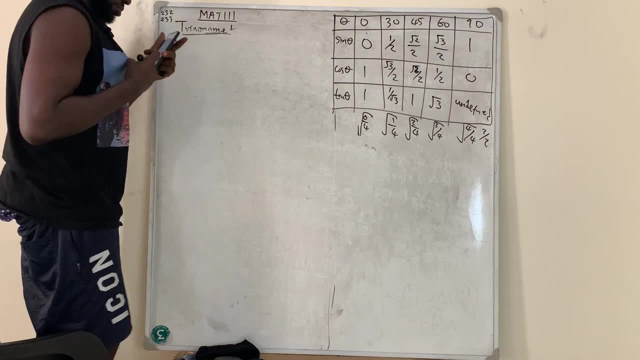 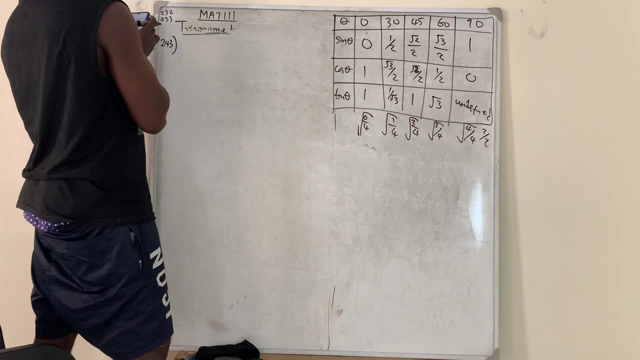 so the next question here said question. so the next question here said question: 243, 243, 243, which said: let me check my video- okay, still moving. let me check my video- okay, still moving. let me check my video- okay, still moving. ah, 30 minutes is gone, all right, okay, so 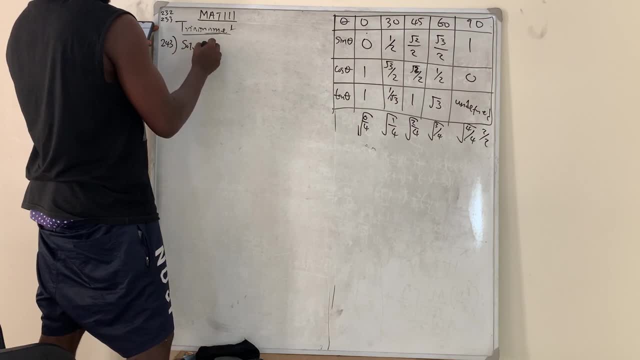 ah, 30 minutes is gone, all right, okay, so, ah, 30 minutes is gone, all right, okay, so i have that, i have that, i have that. uh, they say solve, uh, they say solve. uh, they say solve, solve, solve, solve. sine x minus two sine x, sine x minus two sine x. 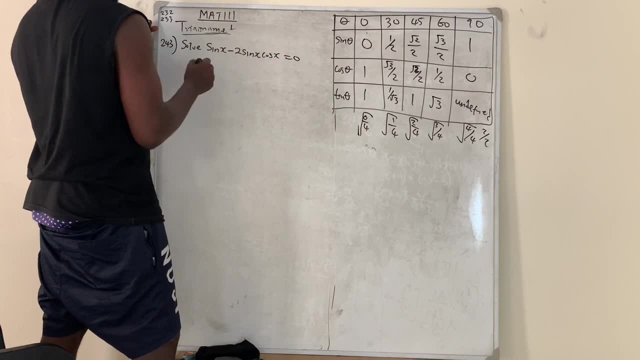 sine x minus two, sine x cos x cos x cos x is equal to zero, and they say that x lies is equal to zero, and they say that x lies is equal to zero and they say that x lies between between between. uh, pi over two, uh, pi over two. 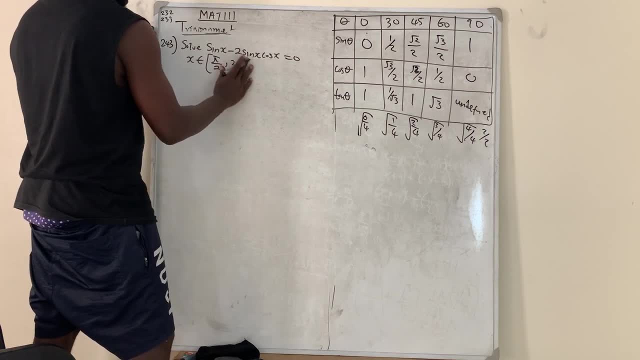 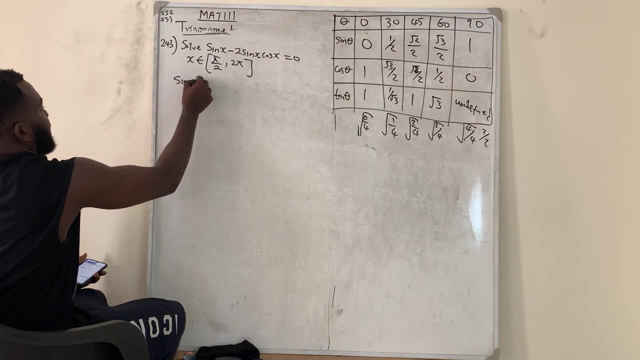 uh pi over two and the two pi okay and two pi all right and two pi all right and two pi all right. so this is a very simple question. so so, this is a very simple question. so so, this is a very simple question. so they gave us sine x minus two. 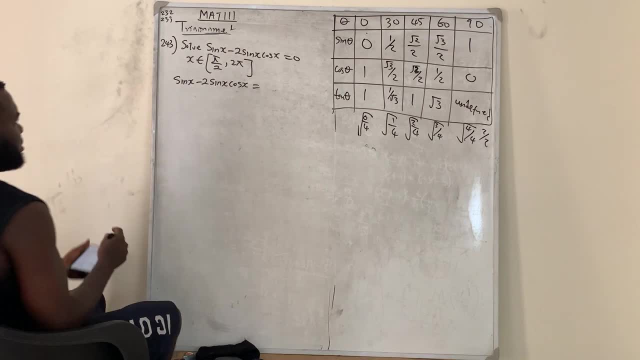 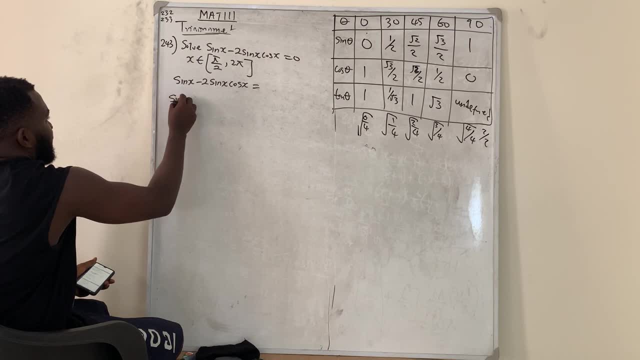 what do we do in this case? well, uh, let. what do we do in this case? well, uh, let me try anyways, so let us factorize. if me try, anyways, so let us factorize. if me try anyways, so let us factorize. if you factorize, i have sine x. 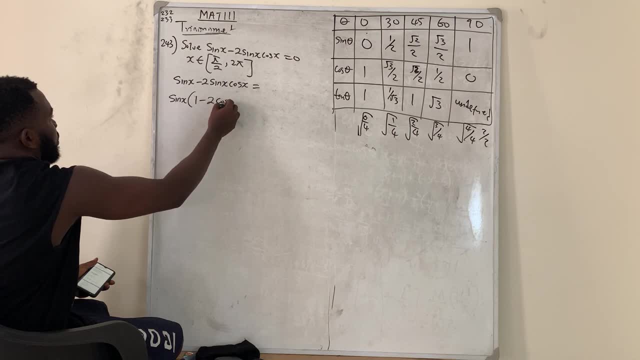 you factorize, i have sine x. you factorize, i have sine x. in bracket of one minus two. in bracket of one minus two, in bracket of one minus two. cos x, cos x, cos x is equal to zero. okay is equal to zero. okay is equal to zero. okay, so, which means um? 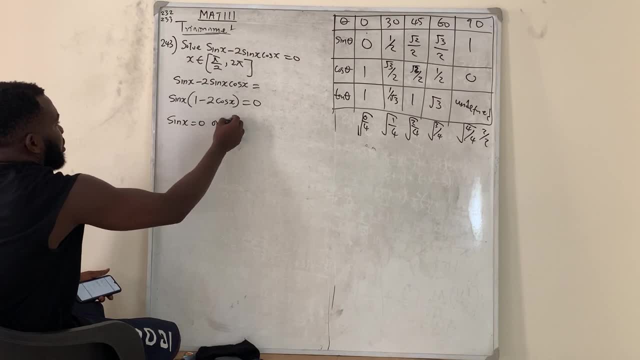 so which means um, so which means um. we now have that that sine x is equal. we now have that that sine x is equal. we now have that that sine x is equal to zero, or one one minus two to zero, or one one minus two to zero, or one one minus two, cos x is equal to zero. so cos x is equal to zero. so cos x is equal to zero. so, sine, what will give you zero if you look sine? what will give you zero if you look sine? what will give you zero if you look at that? you see that, at that, you see that. 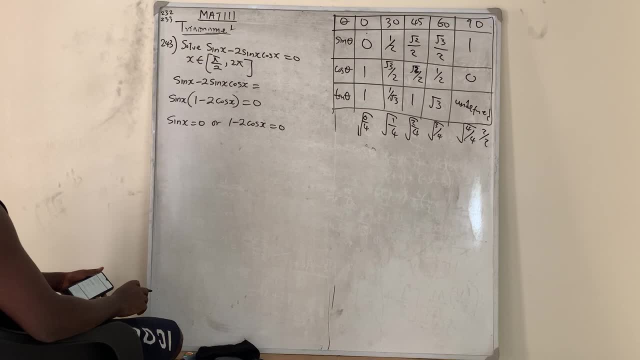 at that. you see that sine um sine um, sine um sine 90, sine 90, sine 90, sine zero is giving me zero, but they say sine zero is giving me zero. but they say sine zero is giving me zero. but they say that, that, uh, uh. 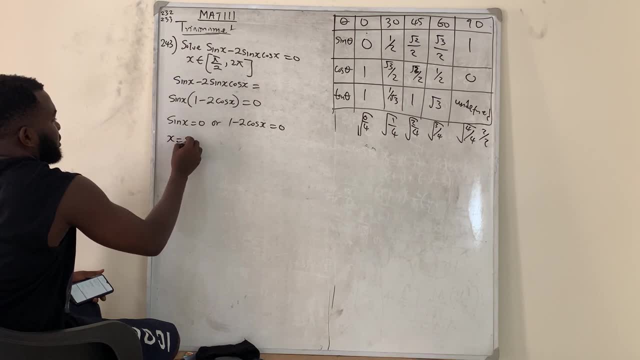 that uh, uh, that uh uh. that x fall between watch your x is equal. that x fall between watch your x is equal. that x fall between watch your x is equal to what the sine inverse of zero and to what the sine inverse of zero and to what the sine inverse of zero and sine inverse of zero is um. 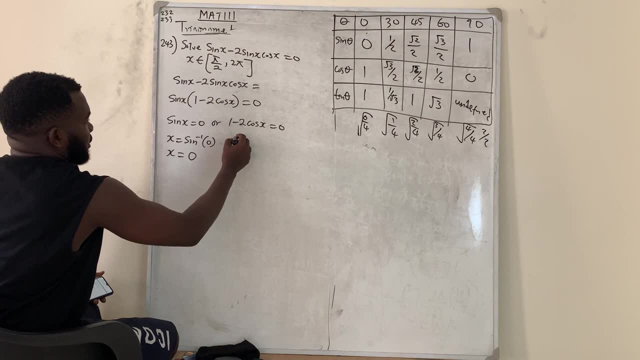 sine inverse of zero is um sine inverse of zero is um. chinese verse of zero is zero, okay, but chinese verse of zero is zero, okay, but chinese verse of zero is zero, okay. but coming to this place, you have that word. coming to this place, you have that word. 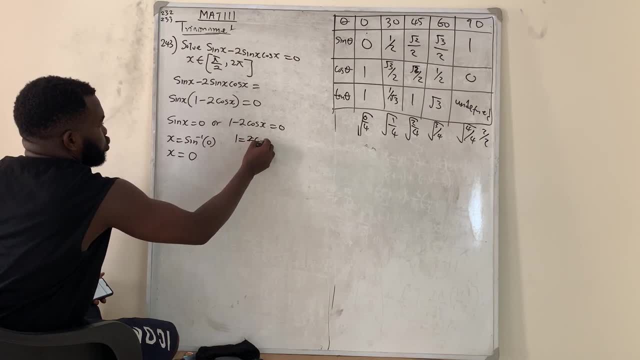 coming to this place, you have that word, that one, my, that one, my that one, my one will be equal to what two cos x. so one will be equal to what two cos x. so one will be equal to what two cos x. so therefore, cos s will not be one over two. 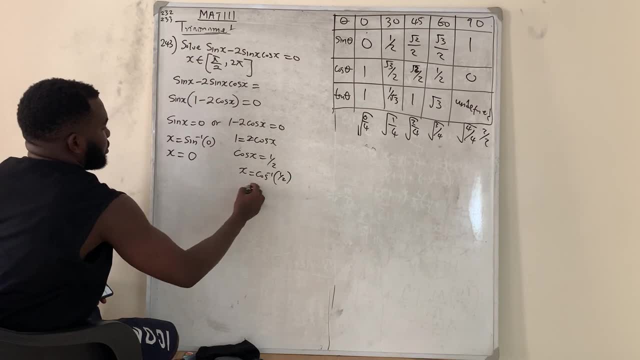 therefore, cos s will not be one over two. therefore, cos s will not be one over two, so x will not be the cos inverse of one, so x will not be the cos inverse of one, so x will not be the cos inverse of one over two. so you are going to have cost. 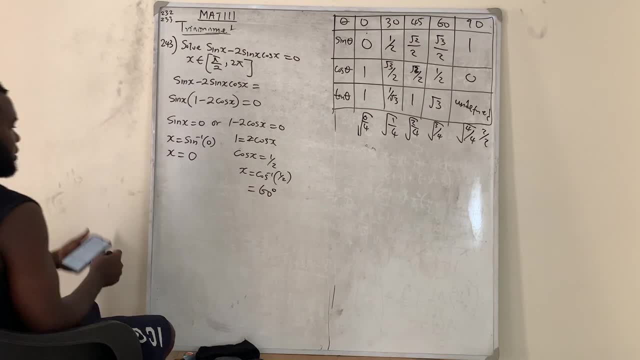 over two. so you are going to have cost over two. so you are going to have cost inverse of one over two will give you 60. inverse of one over two will give you 60. inverse of one over two will give you 60 degrees. all right, so, but if you look at, 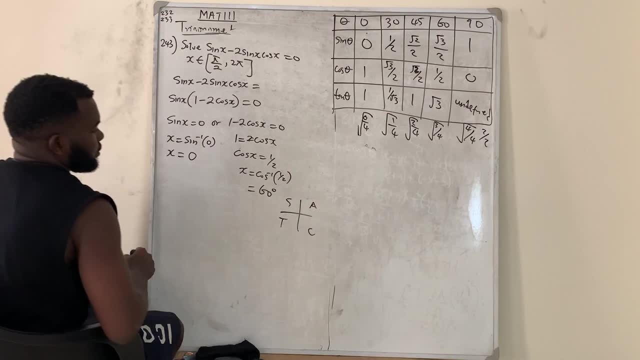 degrees. all right so, but if you look at degrees, all right so, but if you look at cast c a s t, cast c a s t, cast c a s t, so so, so cost is equally positive, cost is equally positive. cost is equally positive in um, in um. 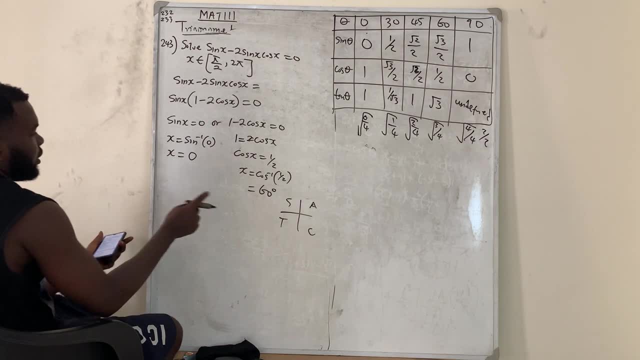 in um, in the, in the, in the second quadrant. so if we say that, where second quadrant, so if we say that, where second quadrant. so if we say that: where do we have zero? where can we have zero? do we have zero? where can we have zero? do we have zero? where can we have zero? so check all deposit, all the possible. 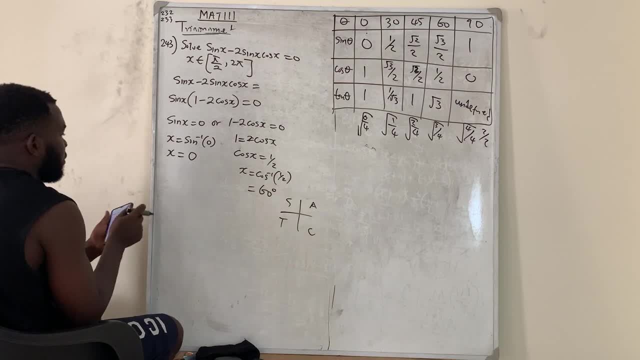 so check all deposit all the possible. so check all deposit all the possible answers, let me see if they okay. so answers, let me see if they okay, so answers, let me see if they okay. so therefore, my x is an element of my x is. therefore, my x is an element of my x is. 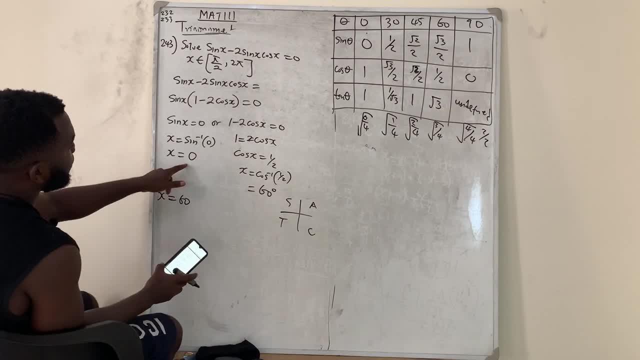 therefore, my x is an element of my x is equal to, equal to, equal to 60.. x cannot be zero, but they say that x 60. x cannot be zero, but they say that x 60. x cannot be zero, but they say that x is from 90. 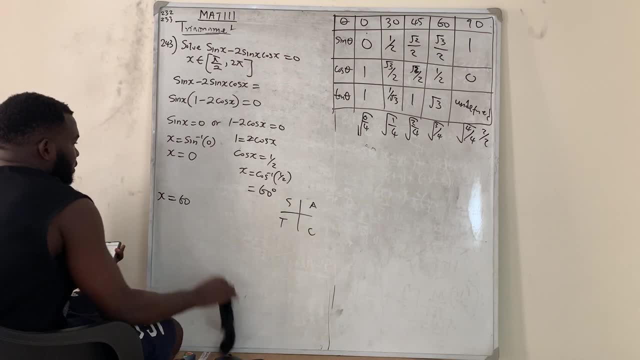 is from 90, is from 90 to 270, so it cannot even be 60. so let to 270, so it cannot even be 60. so let to 270, so it cannot even be 60. so let us say uh, us say uh. 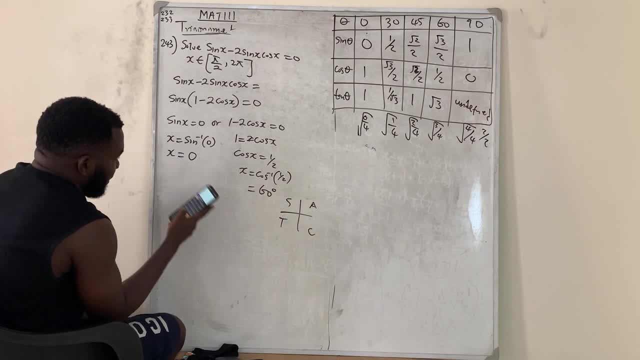 us say: uh, which other one can give us zero sign? which other one can give us zero sign? which other one can give us zero sign? what again can give us that? apart? from what again can give us that? apart, from what again can give us that, apart from zero? let's say: sine 180, let's see what. 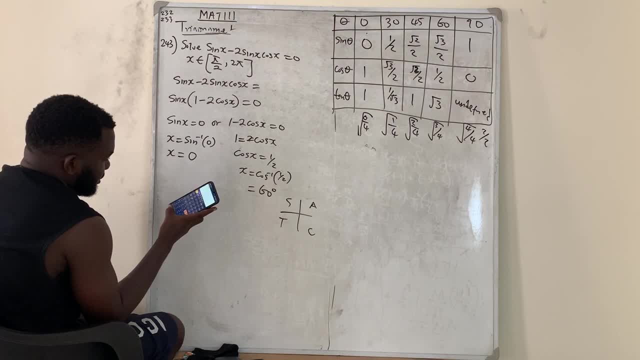 zero, let's say sine 180. let's see what zero, let's say sine 180. let's see what i want it to give us sine. i want it to give us sine. i want it to give us sine 180, 180, 180, oh, zero, so 180. so therefore, 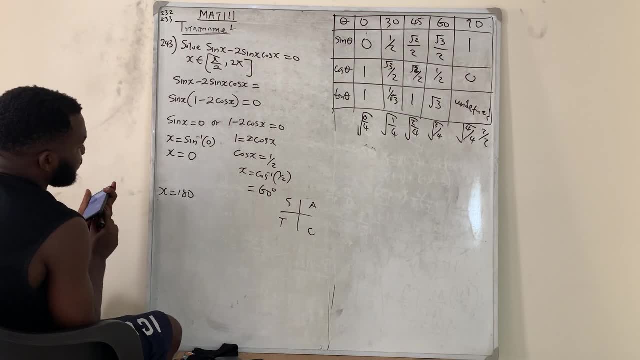 oh zero so 180. so therefore, oh zero so 180. so therefore, my x is equal to 180. so which other one, my x, is equal to 180? so which other one? my x, is equal to 180. so which other one can give us zero? 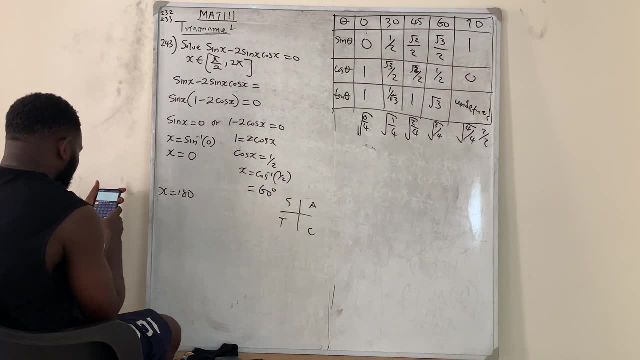 can give us zero, can give us zero or half, or cost anything that can give us or half, or cost anything that can give us or half, or cost anything that can give us up. so let me say cos up, so let me say cos up, so let me say cos, 180 plus 60, 180 plus 60 is giving us 240. 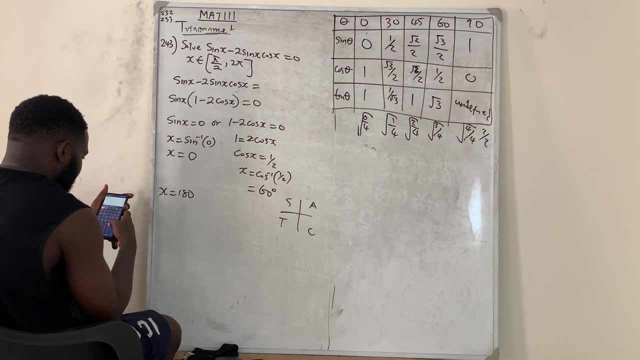 180 plus 60. 180 plus 60 is giving us 240, so let me say cos 240. so let me say cos 240. so let me say cos 240. okay, minus half if i say cos 240. okay minus half if i say cos 240. 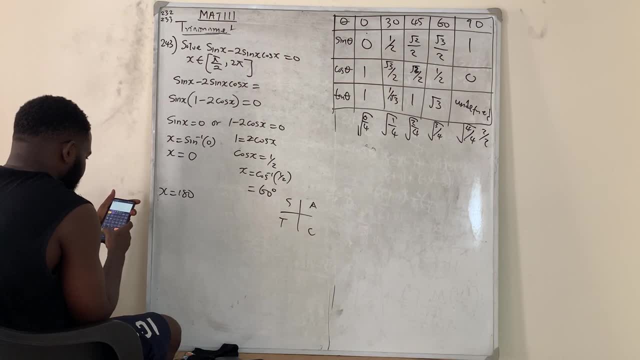 okay, minus half. if i say cos 240 or 240 is now here. so if i say 180 or 240 is now here, so if i say 180 or 240 is now here, so if i say 180 minus 60, that is 120, 120 will be. 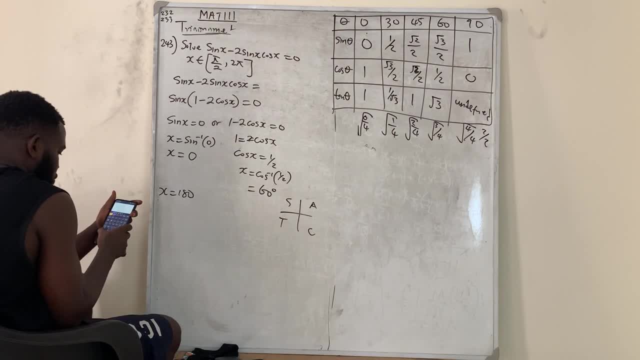 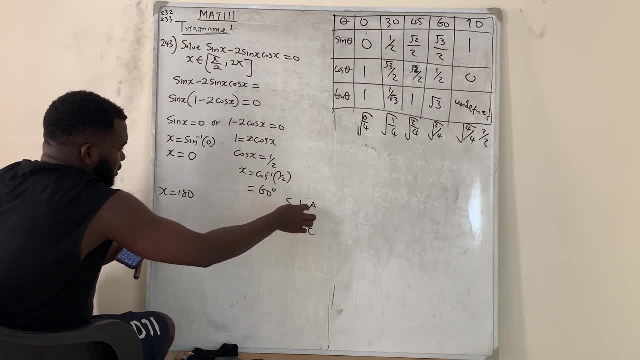 okay, this is according to trigonometry. okay, this is according to trigonometry. okay, this is according to trigonometry. this is first second. this is first second. this is first second cast: cast from the fourth quadrant: okay. cast from the fourth quadrant- okay. cast from the fourth quadrant: okay. sorry, this is the second quadrant. 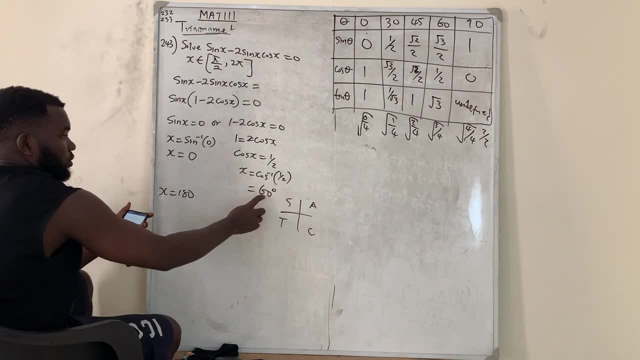 sorry, this is the second quadrant. sorry, this is the second quadrant. third: fourth: okay, fourth quadrant. so third. fourth: okay, fourth quadrant. so third, fourth- okay, fourth quadrant. so we'll be looking for fourth quarter. so we'll be looking for fourth quarter. so we'll be looking for fourth quarter. so if first quarter should be, 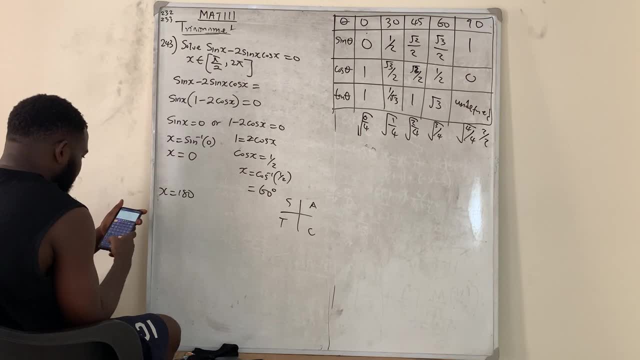 if first quarter should be. if first quarter should be: uh 360 minus this, so that is 300. because uh 360 minus this, so that is 300. because uh 360 minus this, so that is 300, because 300 should give us a hair, 300 should give us a hair. 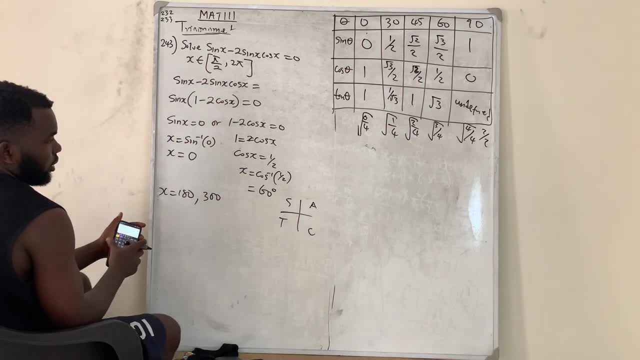 300 should give us a hair half, so i'm having that. 300 is among half, so i'm having that. 300 is among half, so i'm having that. 300 is among. are you getting the one? i'm getting it? are you getting the one? i'm getting it? 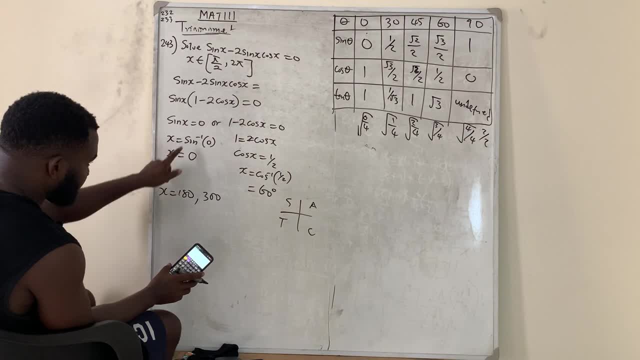 are you getting the one? i'm getting it because just take anything that will give, because just take anything that will give, because just take anything that will give you zero, you, zero, you zero. sign sign one eight is giving me zero. sign sign one eight is giving me zero. 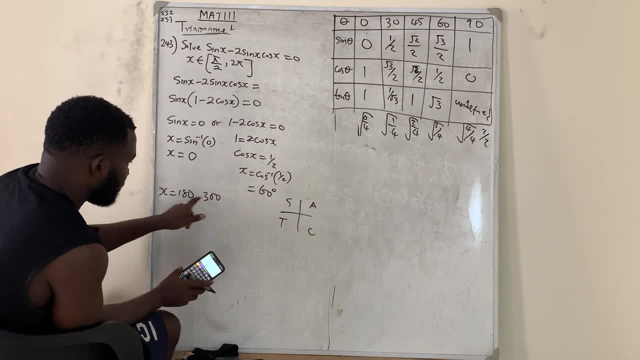 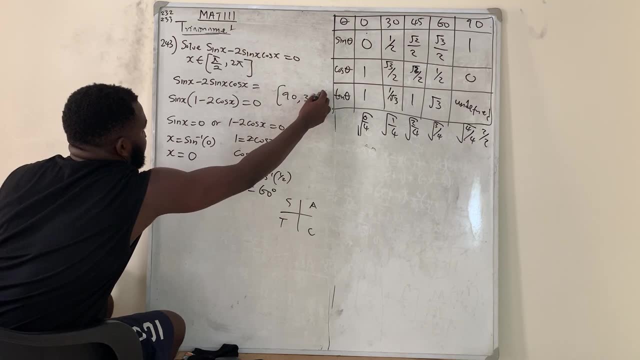 sign, sign. one. eight is giving me zero. okay, okay, okay. cost 300 will give me zero, because we cost 300 will give me zero. because we cost 300 will give me zero, because we need something that will fall between need something that will fall between need something that will fall between anything that will fall between 90 to 360. anything that will fall between 90 to 360.. anything that will fall between 90 to 360.. you get anything that will fall between 90. you get anything that will fall between 90 to 360.. you get anything that will fall between 90 to 360. 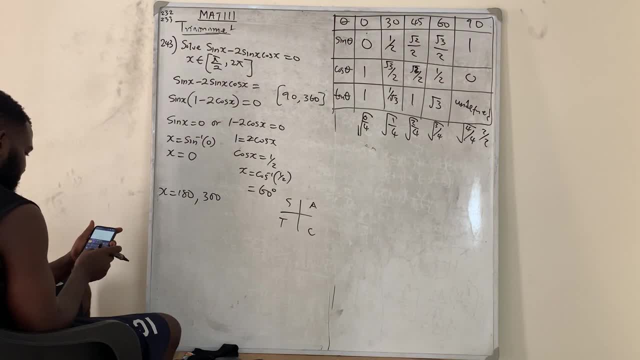 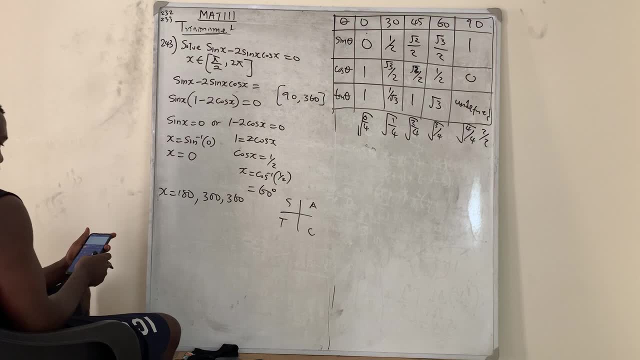 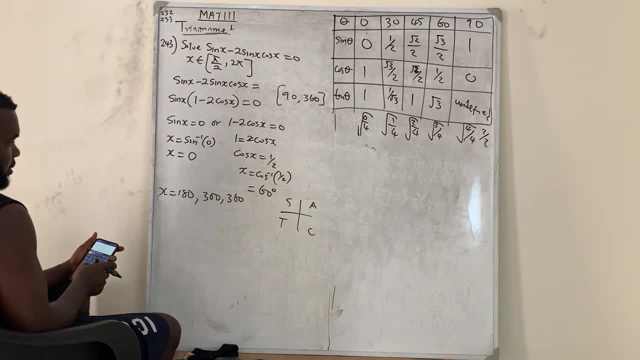 uh, sign. let's say sign 270. can 270 give us sign 360, wow, sign 360, wow, sign 360, wow. so i think 60 is zero. okay, sign 270. so i think 60 is zero. okay, sign 270. so i think 60 is zero, okay, sign 270, sign 270. 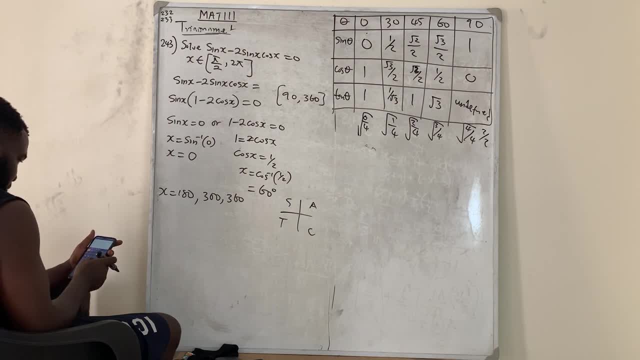 sign: 270 minus one. okay, minus one, okay, minus one, okay, uh cause two, uh cause two, uh cause two. okay, let me check all the special angles. okay, let me check all the special angles. okay, let me check all the special angles. i fall between nine side 90. 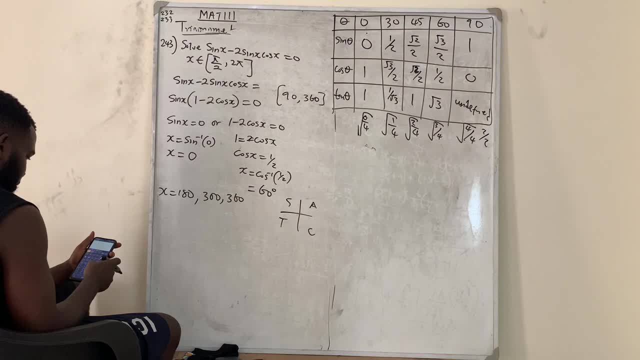 i fall between nine side 90. i fall between nine side 90. sign 90 is one, but this is not one. sign 90 is one, but this is not one. sign 90 is one, but this is not one. okay, sign one eight. sign one eight. 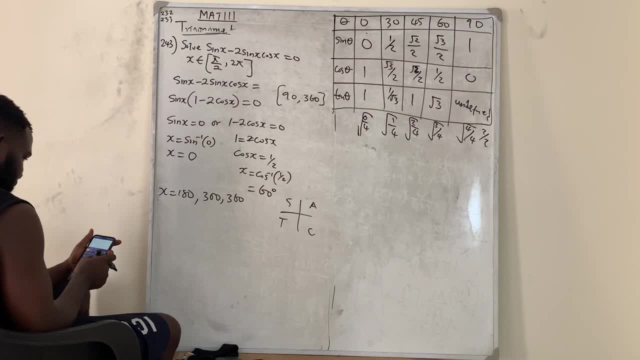 okay, sign one eight. sign one eight. okay, sign one eight. sign one eight zero. so one eight is among uh zero, so one eight is among uh zero, so one eight is among uh sign, sign, sign, okay, i've said 360, so everything about. okay, i've said 360, so everything about. 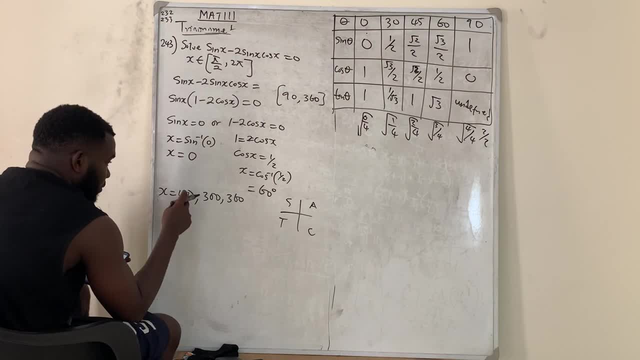 okay, i've said 360, so everything about zero. the only thing that will give us zero, zero, the only thing that will give us zero, zero. the only thing that will give us zero is a 180 and rest. so these are the is a 180 and rest. so these are the. 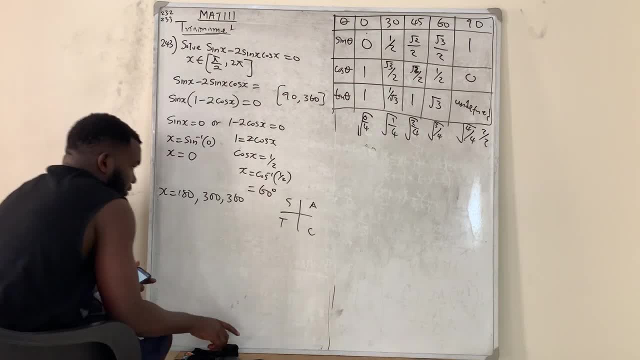 is a 180 and rest. so these are the three answers for this. i don't think three answers for this. i don't think three answers for this. i don't think there's any other one that can give us. there's any other one that can give us? 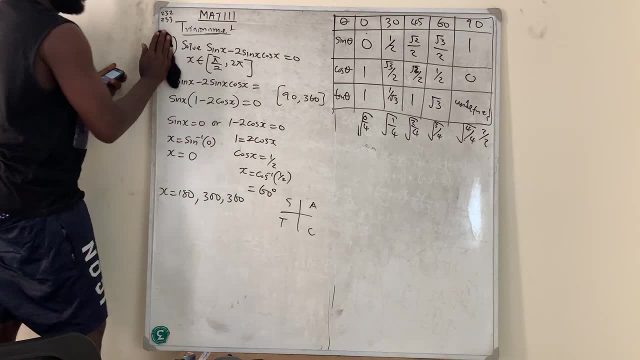 there's any other one that can give us something good, something good, something good. so that is that for that. so move to the. so that is that for that. so move to the. so that is that for that. so move to the next question. next question. next question. we move to the next question, so the next. 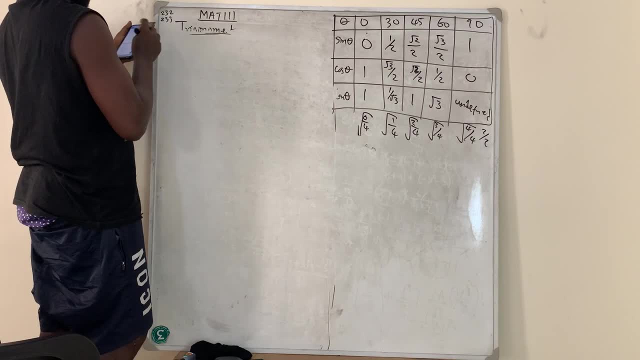 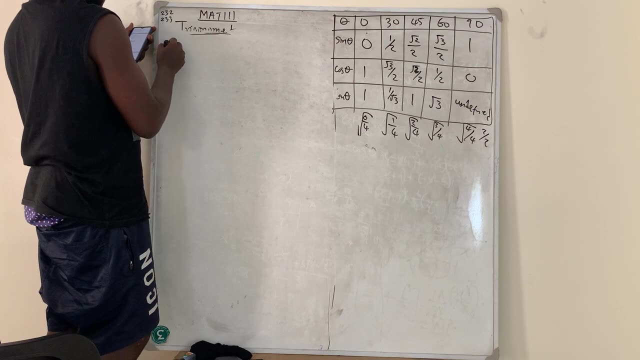 we move to the next question, so the next. we move to the next question. so the next question here said question here said question here said question number, question number two, question number two, question number two. forty four and two forty four said that forty four and two forty four said that. 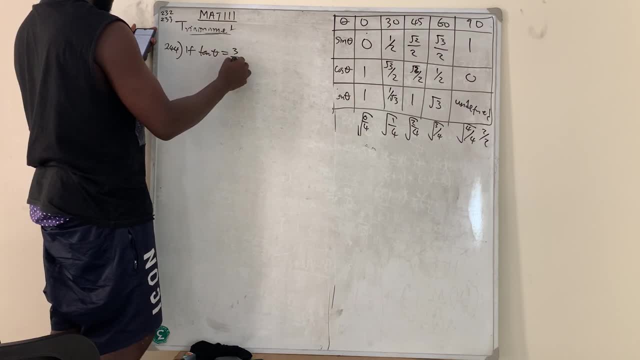 forty four and two forty four said that if, if, if tan theta is equal to three over four, tan theta is equal to three over four, tan theta is equal to three over four, and then three pi over two is less than, and then three pi over two is less than. 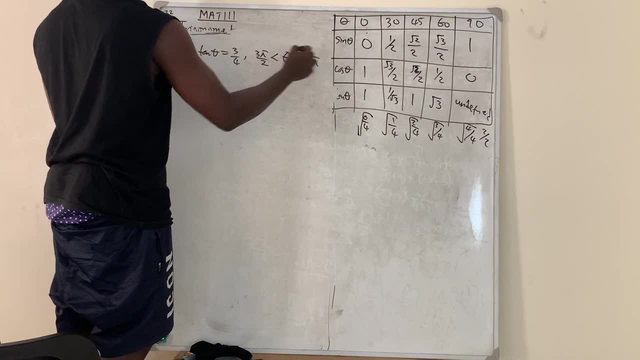 and then three pi over two is less than a, is less than theta, a is less than theta, a is less than theta, which is less than two pi. then i said which is less than two pi. then i said which is less than two pi. then i said then we should find cosec. 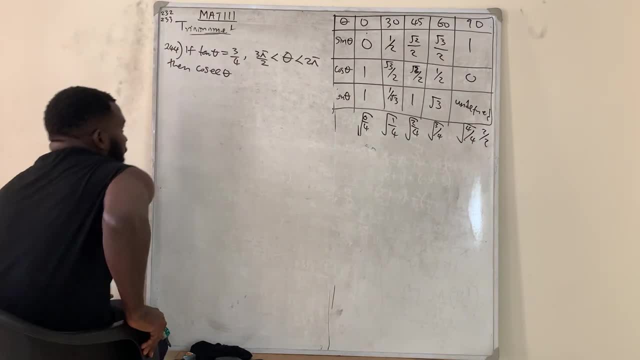 then we should find cosec, then we should find cosec cosec theta. okay, cosec theta, okay, cosec theta. okay, now, what do you do, uh first of all you? now? what do you do uh first of all you now? what do you do uh first of all? you draw it. don't forget that. they say that. 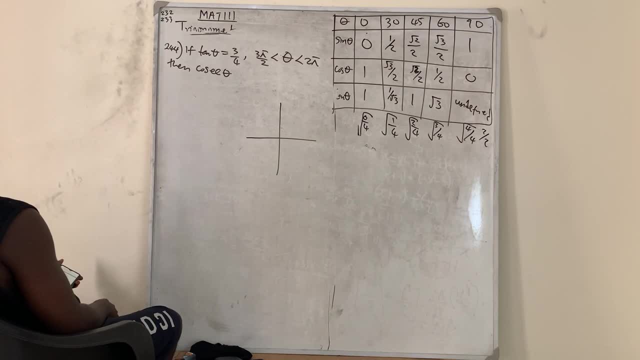 draw it. don't forget that they say that, draw it. don't forget that they say that, that this thing is in the third quadrant, that this thing is in the third quadrant, that this thing is in the third quadrant in trigonometry, are we moving clockwise in trigonometry, are we moving clockwise? 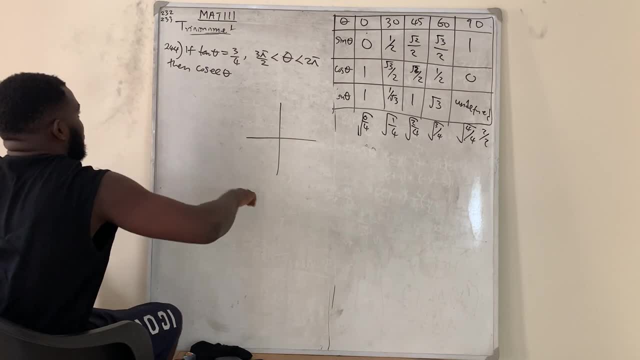 in trigonometry. are we moving clockwise, anti-clockwise? i made mistake. we are anti-clockwise. i made mistake. we are anti-clockwise. i made mistake. we are supposed to move anti-clockwise, supposed to move anti-clockwise. supposed to move anti-clockwise. so in the other, in the other question. 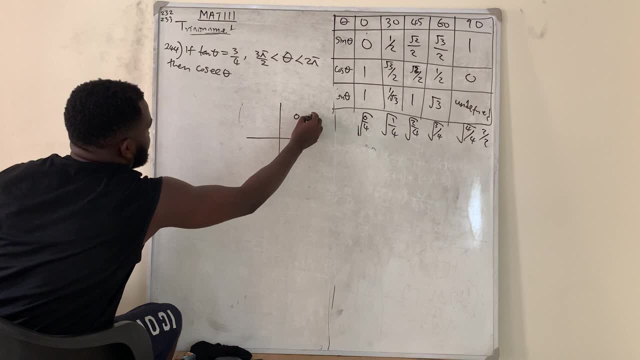 so in the other, in the other question, so in the other, in the other question. please resolve it. we're supposed to move, please resolve it. we're supposed to move, please resolve it. we're supposed to move anti-clockwise. so this is from 0 to 90. 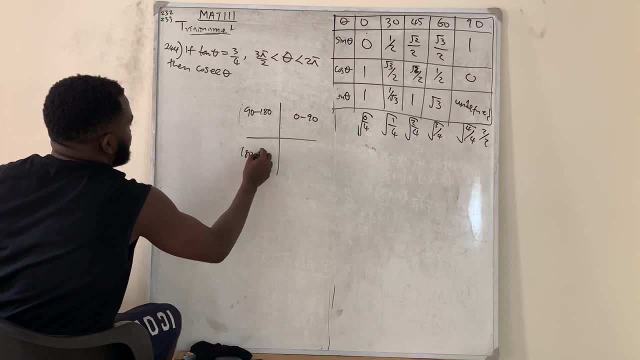 anti-clockwise. so this is from 0 to 90 anti-clockwise. so this is from 0 to 90, 90 to 180, so 180 to 270, then 90 to 180, so 180 to 270, then 90 to 180, so 180 to 270, then 270 to 360.. so please resolve that in. 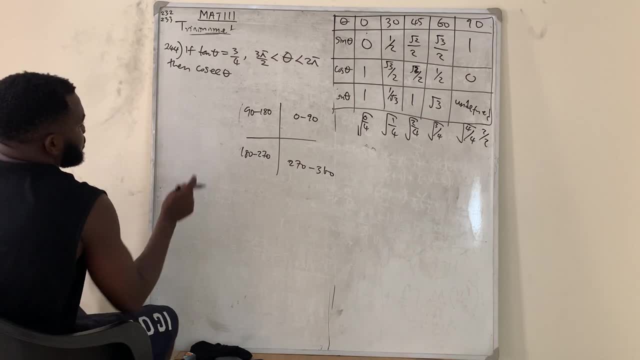 270 to 360.. so please resolve that in 270 to 360.. so please resolve that in the other question. so so this is um the other question. so so, this is um the other question. so so, this is um from 270 to 360. so it fell at the fourth. 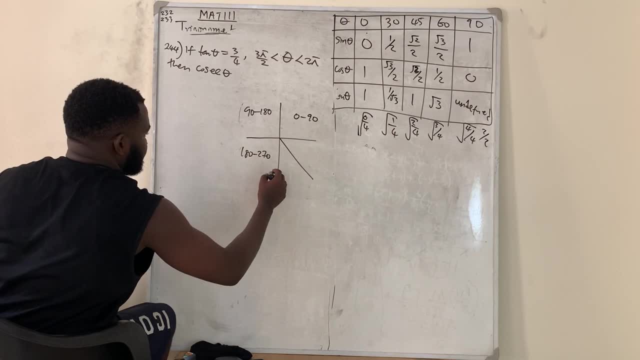 from 270 to 360, so it fell at the fourth. from 270 to 360, so it fell at the fourth quadrant. so at the fourth quadrant i'm quadrant. so at the fourth quadrant i'm quadrant. so at the fourth quadrant i'm going to have something like this: 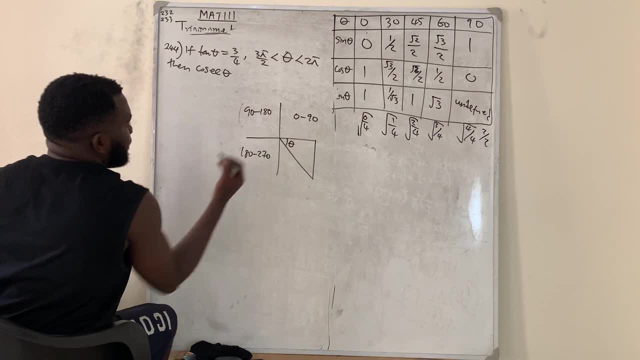 going to have something like this, going to have something like this. if i have something like this, so this is. if i have something like this, so this is. if i have something like this, so this is my theta, my theta, my theta, this is my theta, my, this is my theta, my. 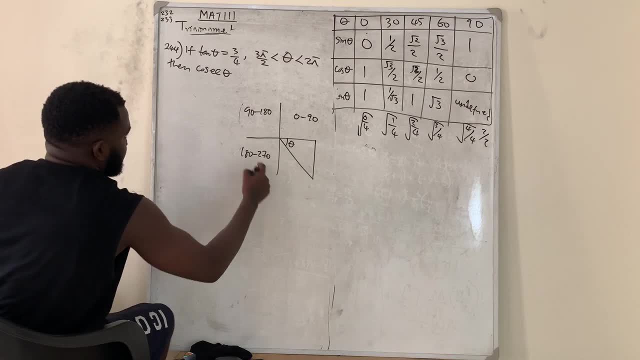 this is my theta. my turn is turn is turn is opposite over adjacent. so my opposite is opposite over adjacent. so my opposite is opposite over adjacent. so my opposite is here. so minus three because it is down here. so minus three because it is down here. so minus three because it is down and my adjacent is in the right hand side. 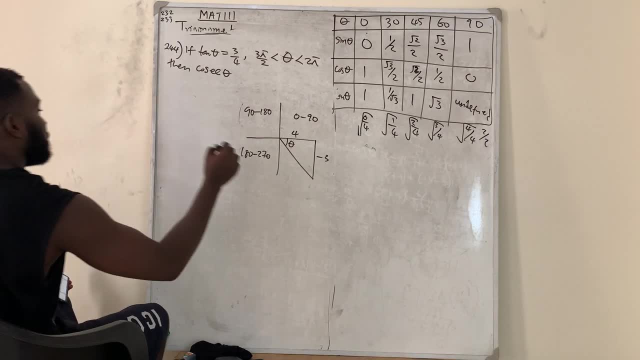 and my adjacent is in the right hand side and my adjacent is in the right hand side, which is four, okay. so that is that so. which is four okay. so that is that, so, which is four okay. so that is that. so, according to pythagoras, triple here is: 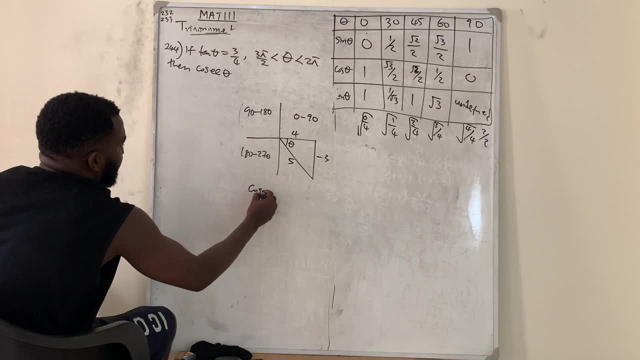 according to pythagoras triple: here is according to pythagoras triple: here is going to be five. so if there is going to going to be five, so if there is going to going to be five, so if there is going to be five, we now have that cosec. 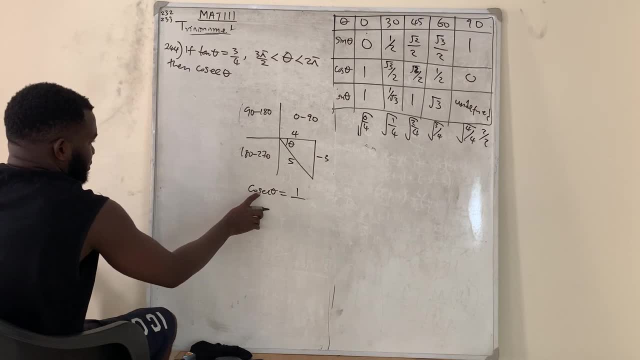 be five. we now have that. cosec be five, we now have that. cosec theta means one over sine theta. one two theta means one over sine theta. one, two theta means one over sine theta. one, two, three. one over sine theta, which is what? three, one over sine theta, which is what. 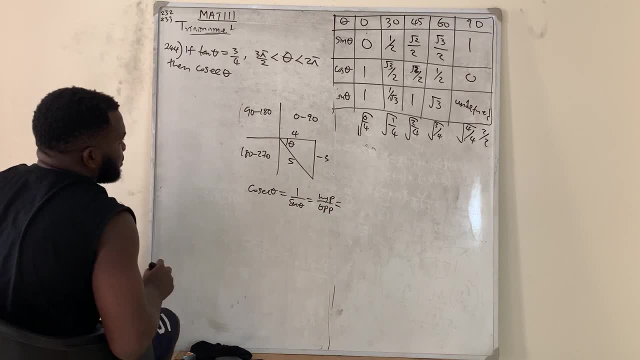 three, one over sine theta, which is what? hypotenuse over opposite. so where is my hypotenuse over opposite? so where is my hypotenuse over opposite? so where is my hypotenuse, hypotenuse, hypotenuse, hypotenuse is five over opposite my. 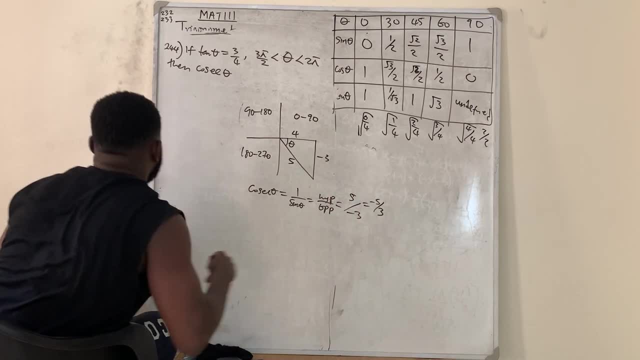 hypotenuse is five over opposite. my hypotenuse is five over opposite. my opposite is minus three. so my answer is opposite is minus three. so my answer is opposite is minus three. so my answer is minus five over three. so minus five over. minus five over three, so minus five over. 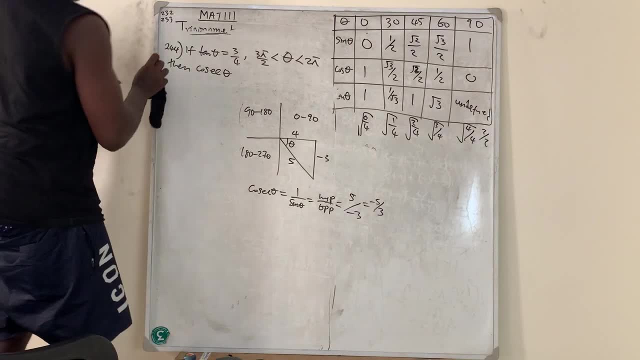 minus five over three. so minus five over three is the answer for that particular three. is the answer for that particular three is the answer for that particular question. so we move to the next question. so we move to the next question. so we move to the next question. 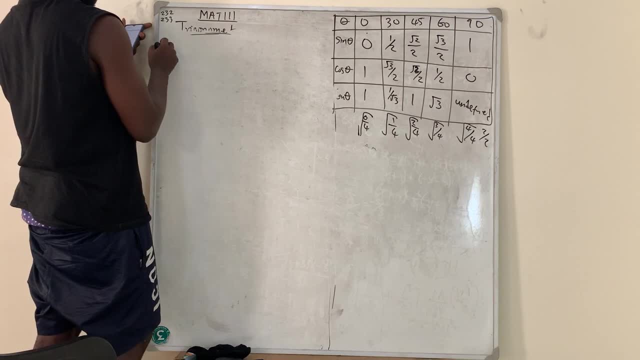 so the next question here say the. so the next question here say the. so the next question here say the question number, question number, question number 245 and question number 245. 245 and question number 245. 245 and question number 245 said that if theta is. 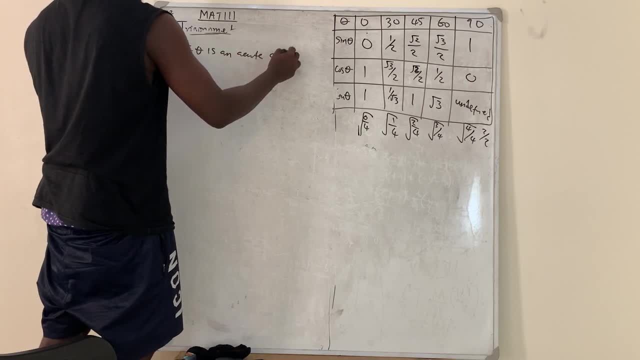 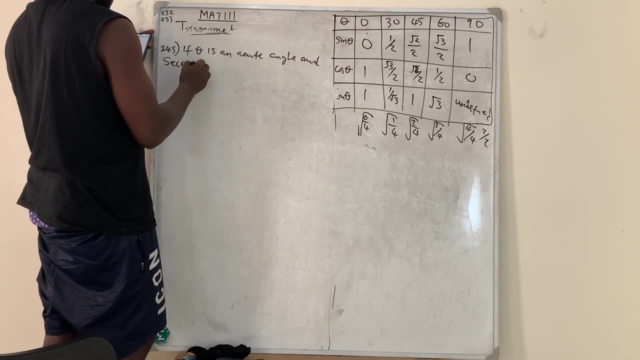 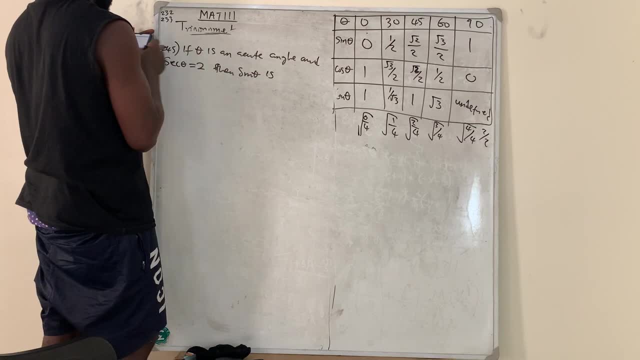 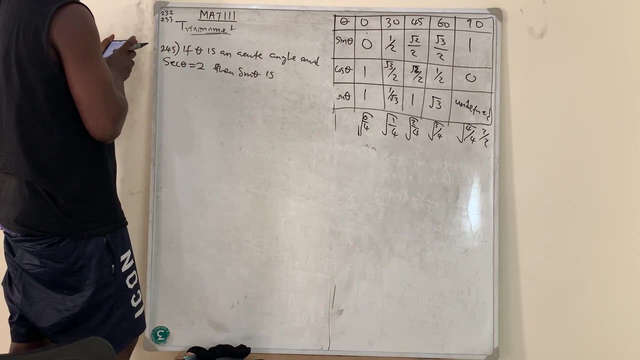 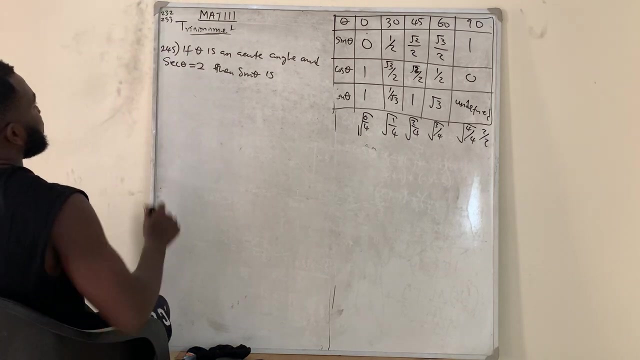 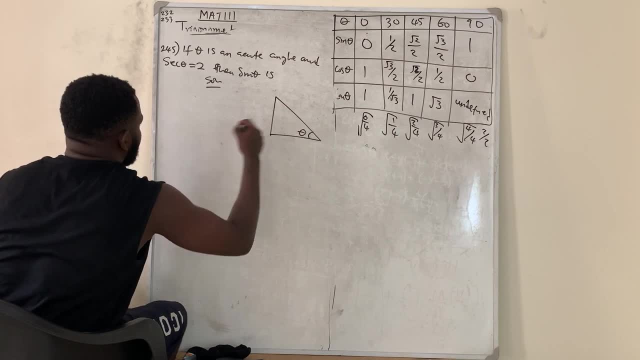 uh, they gave us the same method again. uh, they gave us the same method again. whenever you see acute, just draw your. whenever you see acute, just draw your. whenever you see acute, just draw your. normal triangle, normal triangle, normal triangle. it doesn't affect anything. so sec, sec is. 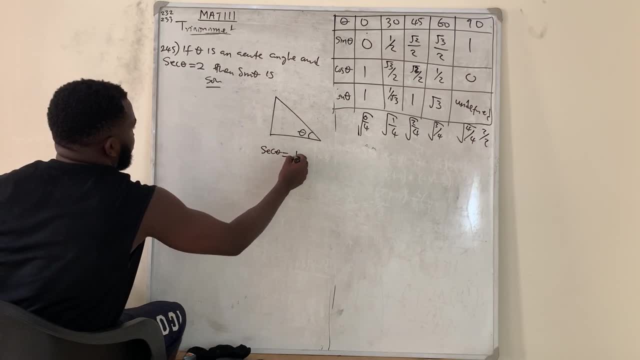 it doesn't affect anything. so sec, sec is: it doesn't affect anything. so sec, sec is one, two, three, one over course. so sec: one, two, three, one over course. so sec: one, two, three, one over course. so sec. theta is equal to one over cost, theta is equal to one over cost. 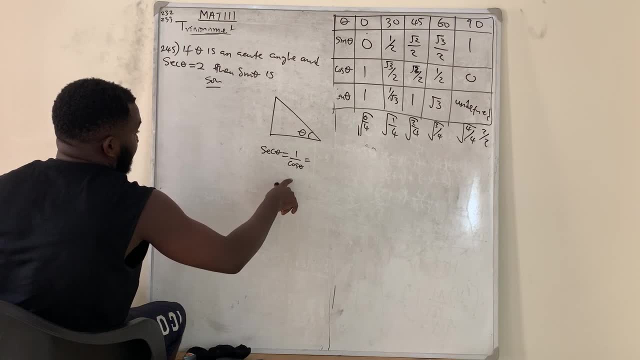 theta is equal to one over cost, theta and cost normally is opposite over theta and cost normally is opposite over theta and cost normally is opposite over adjacent over hypotenuse. so it's going to adjacent over hypotenuse, so it's going to adjacent over hypotenuse, so it's going to be hypotenuse over adjacent, so which is? 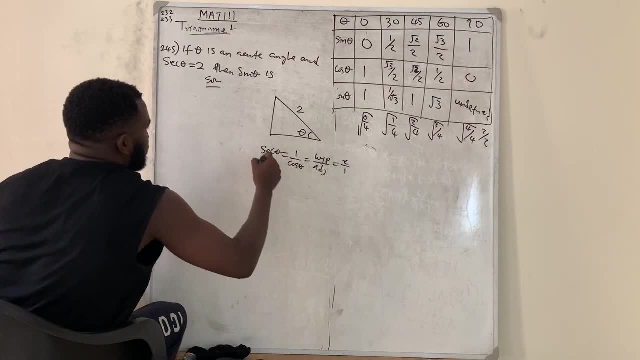 be hypotenuse over adjacent, so which is be hypotenuse over adjacent, so which is what hypotenuse is two, which is they gave. what hypotenuse is two, which is they gave. what hypotenuse is two, which is they gave me two. two is two over one, so over one. 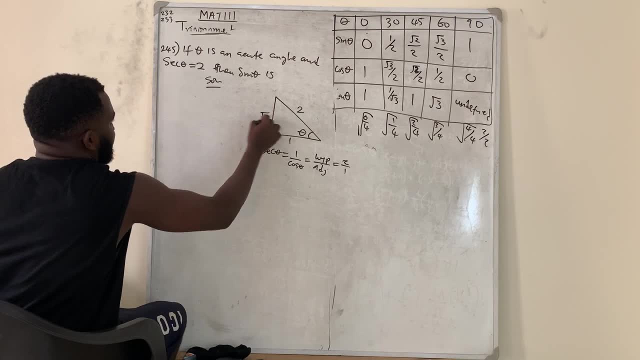 me two. two is two over one, so over one me two. two is two over one, so over one here. so i'm having according to here, so i'm having according to here, so i'm having according to pythagoras crm. here is going to be root. pythagoras crm. here is going to be root. pythagoras crm. here is going to be root three. you have done it before, so this is three. you have done it before, so this is three. you have done it before, so this is going to be root three. 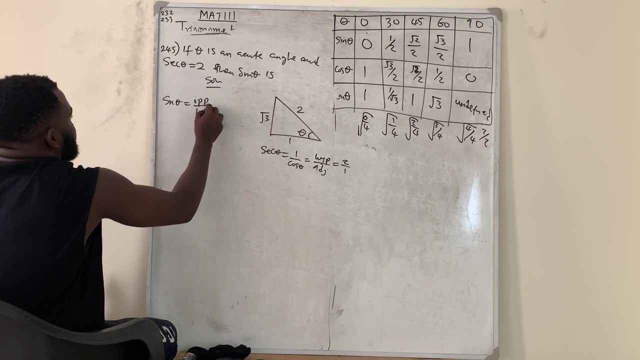 going to be root three. going to be root three sine theta is equal to what opposite over sine theta is equal to what opposite over sine theta is equal to what opposite over hypotenuse, which is equal to what hypotenuse, which is equal to what hypotenuse, which is equal to what root. 3 over 2, so that 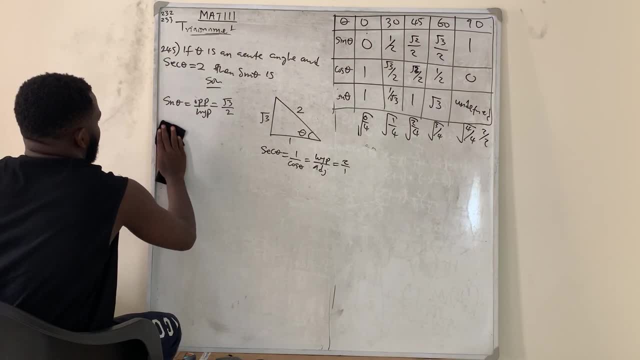 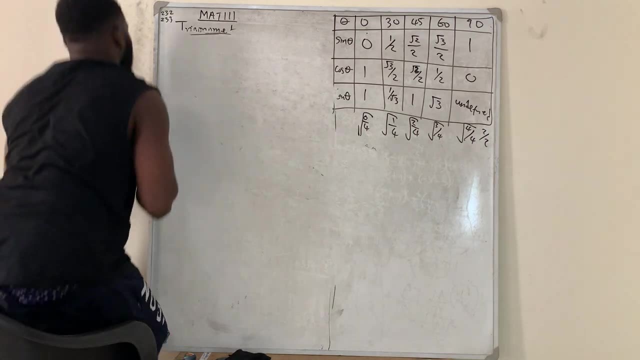 root 3 over 2. so that root 3 over 2. so that is that is. that, is that right, okay, okay, okay. so we move to the next one. so we move to the next one, so we move to the next one. the next one is a question number. 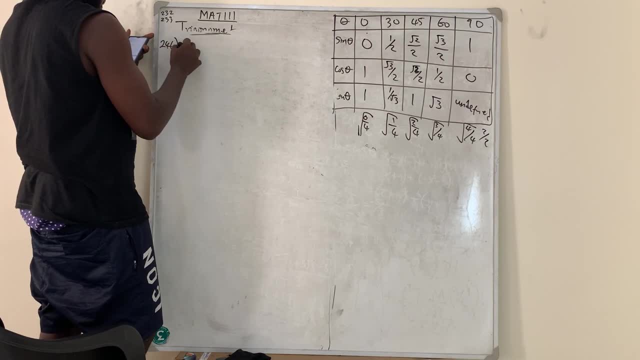 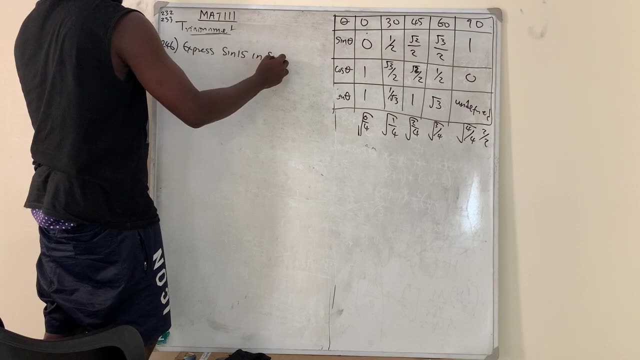 question number 246 and question number. question number 246 and question number. question number 246 and question number 247. express 247, express 247. express express sign 15. express sign 15. express sign 15 in sword, in sword, in sword form, form form express sign 15 in sword form. solution. 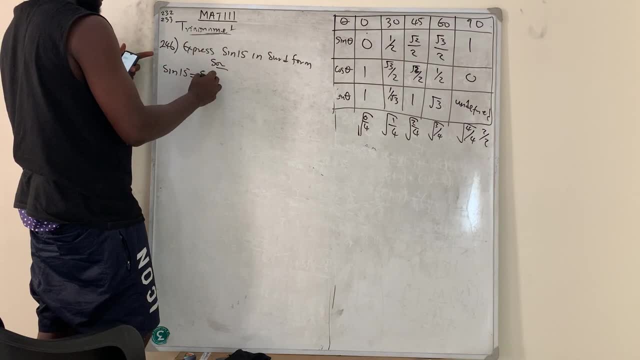 express sign 15 in sword form solution. express sign 15 in sword form solution. you know that sign 15 is same thing. as you know that sign 15 is same thing, as you know that sign 15 is same thing as saying, saying, saying sine 45 minus 30, which is what. 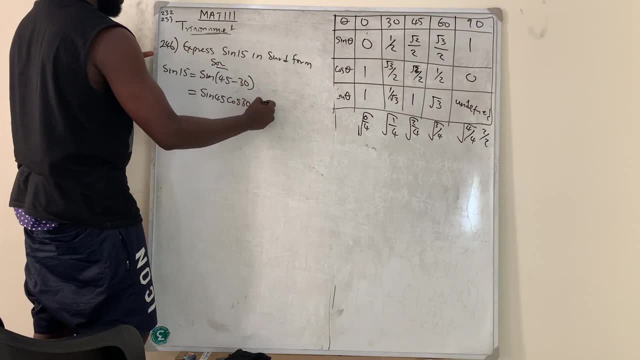 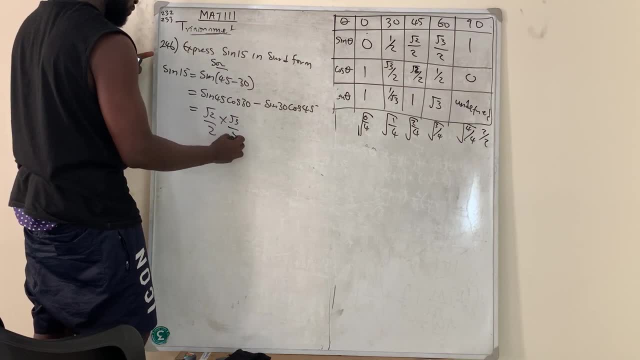 sine 45 cos 30 cos 45, which is what root 2 over 2 times root 3 over 2. root 2 over 2 times root 3 over 2. root 2 over 2 times root 3 over 2 minus. 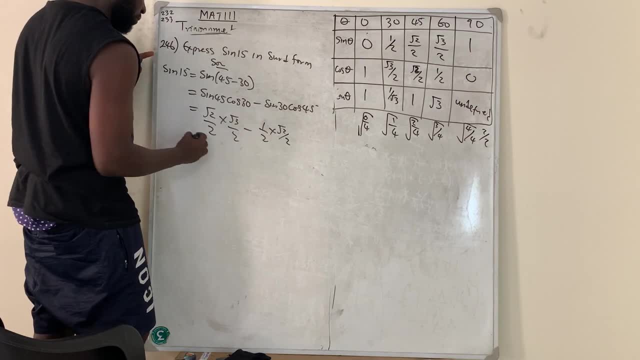 minus, minus minus 1 over 2 times root 2 over 2. so minus 1 over 2 times root 2 over 2. so minus 1 over 2 times root 2 over 2. so i'm left with root 6 over 4. 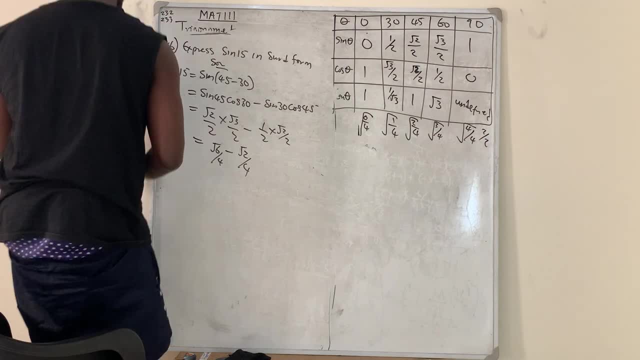 i'm left with root 6 over 4. i'm left with root 6 over 4, minus root 2 over 4. so what do they have? minus root 2 over 4? so what do they have minus root 2 over 4? so what do they have as the option? so in the option they have, 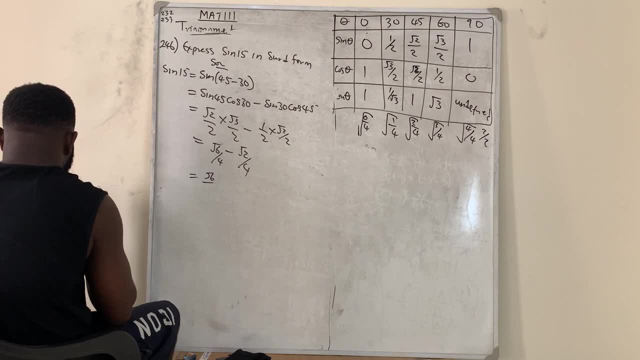 as the option. so in the option they have as the option. so in the option they have root 6 over root 6 over 4.. the option is not correct. supposed to root 6 over 4.. the option is not correct. supposed to root 6 over 4.. the option is not correct. supposed to be root 6 over 4 into root uh. 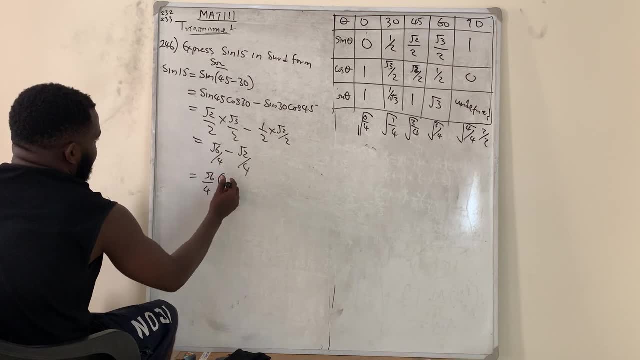 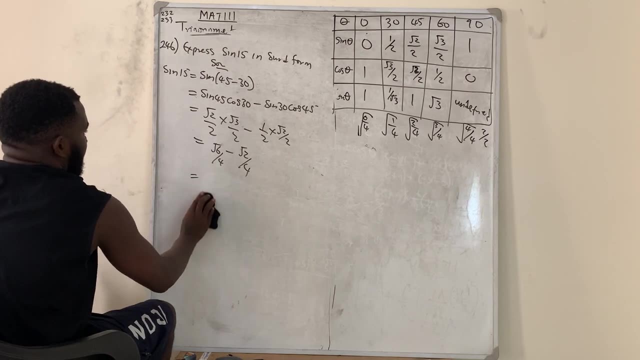 be root 6 over 4 into root. uh, be root 6 over 4 into root. uh, root 3, root 3. root 3. sorry into one, sorry into one, sorry into one minus huh, what am i saying? sorry, it's going to be, sorry, it's going to be. 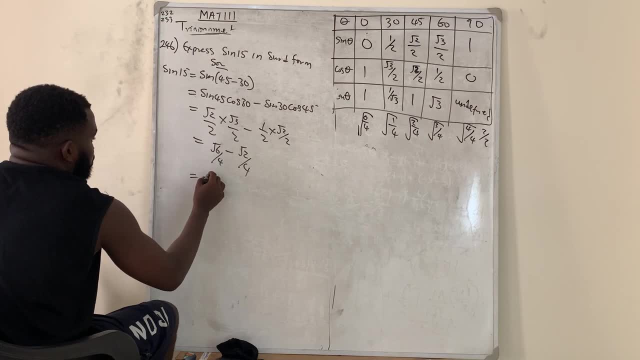 sorry it's going to be, that is, if it's one over four, that is if it's one over four, that is if it's one over four. okay root two. sorry root two. okay root two. sorry root two. okay root two. sorry root two. root two over four into. 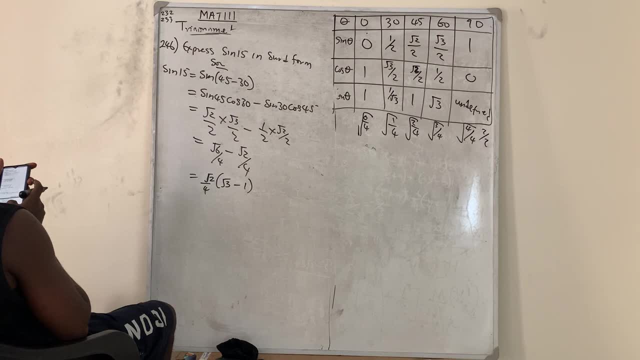 root. two over four into root. two over four into root. three minus one root. two over four root. three minus one root. two over four root. three minus one root. two over four into root. three into root. three into root. three minus one. okay, option a is very, very. 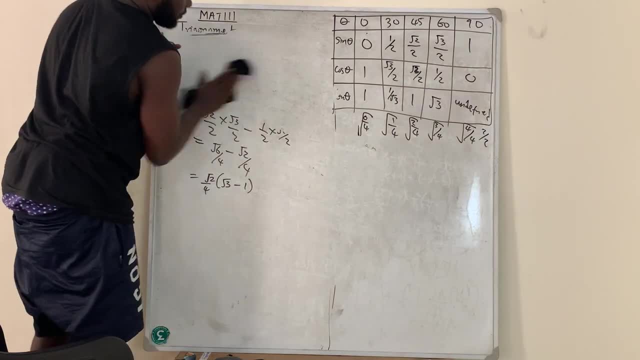 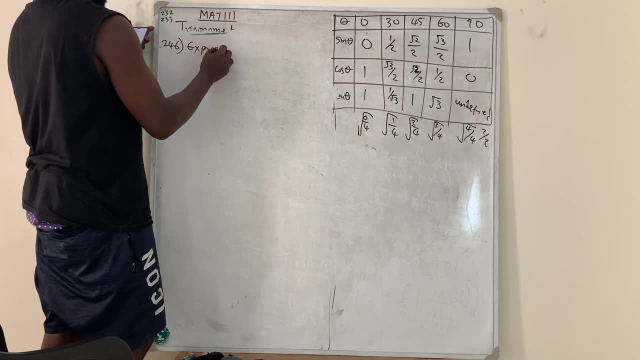 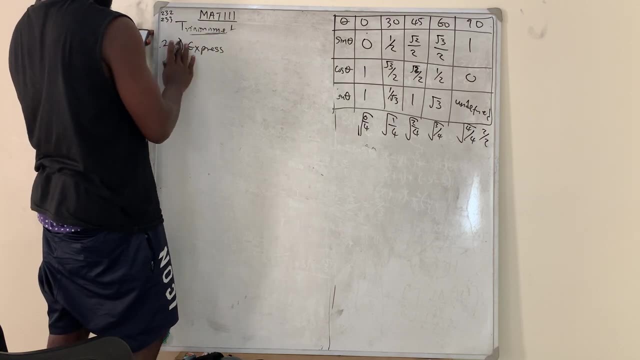 question number 246. question number 246 said express. said express. said express express um sorry. 250. question number 250, sorry. 250. question number 250. sorry. 250. question number 250. question number 250 said question number 250 said question number 250. said convert. convert. 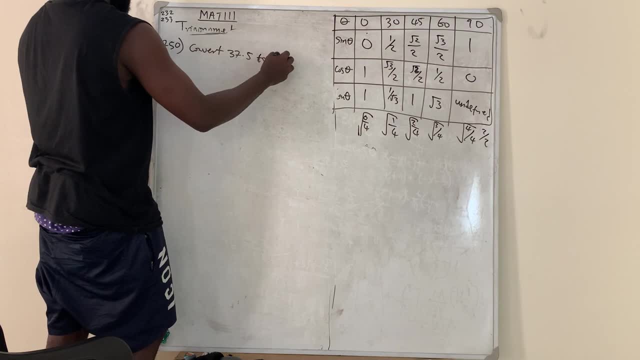 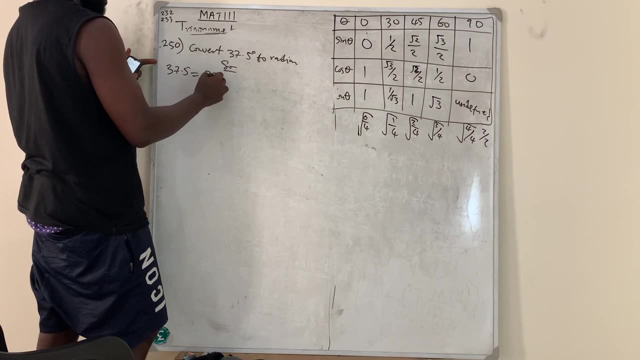 convert, convert, convert, convert. 37.5, 37.5, 37.5 to radian to radian to radian. so what do you do? solution? so what do you do solution? so what do you do? solution: so you have: 37.5 is equal to 37.5. 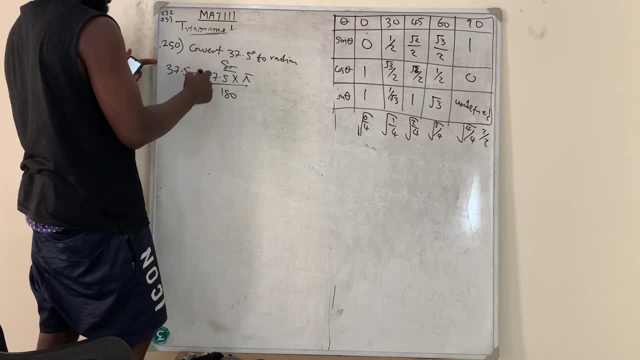 so you have: 37.5 is equal to 37.5. so you have: 37.5 is equal to 37.5 times pi, then divided by 180, so just times pi, then divided by 180, so just times pi, then divided by 180. so just reduce these two to the lowest, okay. 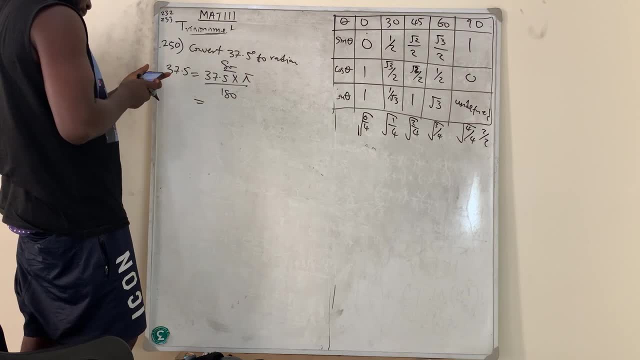 reduce these two to the lowest. okay, reduce these two to the lowest. okay, reduce it to the lowest. so you're going reduce it to the lowest. so you're going reduce it to the lowest. so you're going to have 37 to have, 37 to have 37.5 divided by 180. 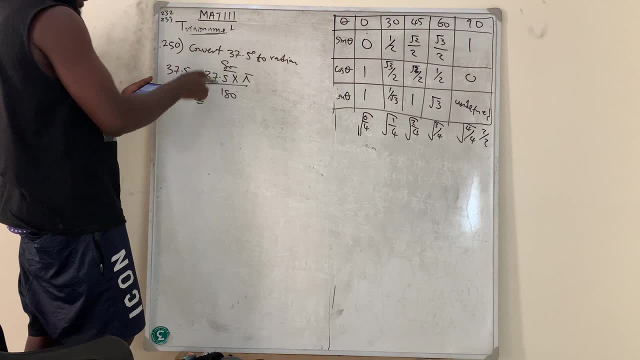 .5 divided by 180, .5 divided by 180, so i have a. if you reduce it to the, so i have a. if you reduce it to the, so i have a. if you reduce it to the lowest, lowest, lowest. so find how to reduce this into the. 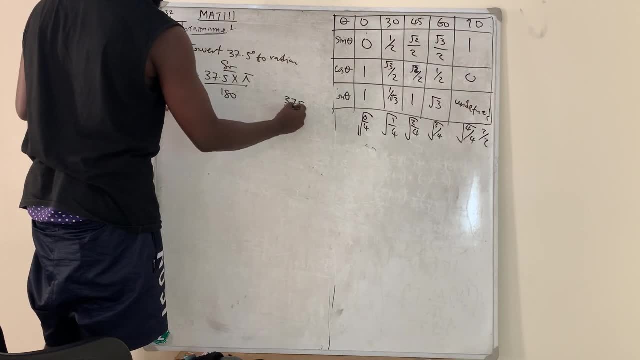 so find how to reduce this into the. so find how to reduce this into the. lowest, that is, you can say 375 divided. lowest, that is, you can say 375 divided. lowest, that is, you can say 375 divided by 1800. so you now be sharing it, see you? 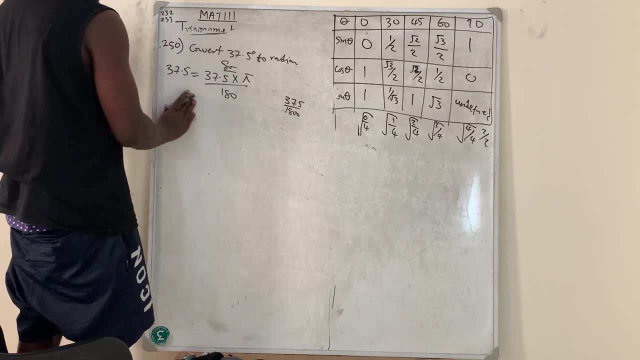 by 1800, so you now be sharing it. see you, by 1800, so you now be sharing it. see, you reduce it to the lowest form. so you now reduce it to the lowest form. so you now reduce it to the lowest form. so you now put your pi. so that is the answer, that 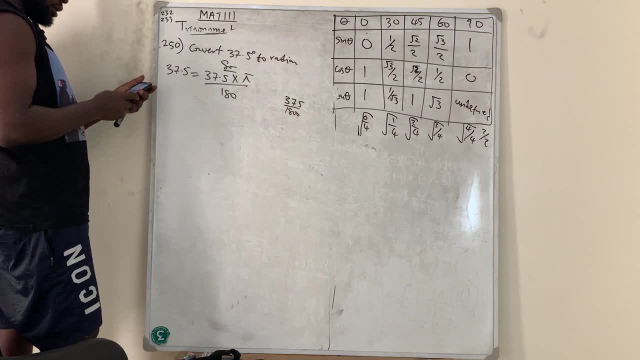 put your pi. so that is the answer. that put your pi, so that is the answer that okay, okay, so, maybe, okay, let me just help five can. so maybe okay, let me just help five can. so maybe okay, let me just help five can divide. so if i divide, let's start with. 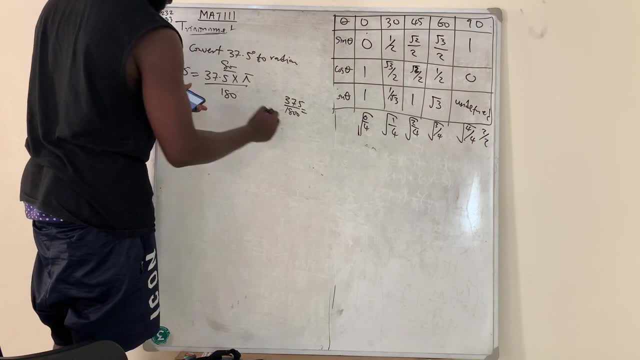 divide. so if i divide, let's start with divide. so if i divide, let's start with five, three, seven, five divided by five. so five, three, seven, five divided by five. so five, three, seven, five divided by five. so i have 75 over. i have 75 over. 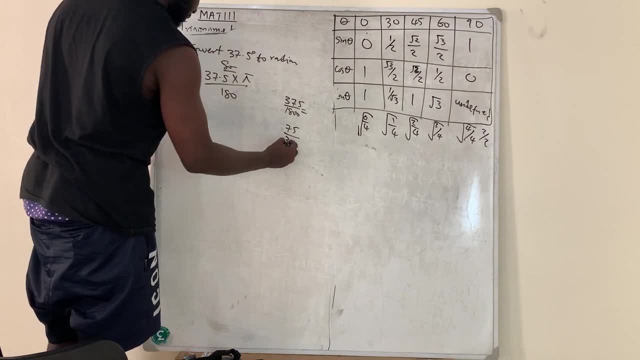 i have 75 over 1 800 divided by five, so i have 360.. 1 800 divided by five, so i have 360.. 1 800 divided by five, so i have 360.. five again can divide divided by five. again can divide divided by. 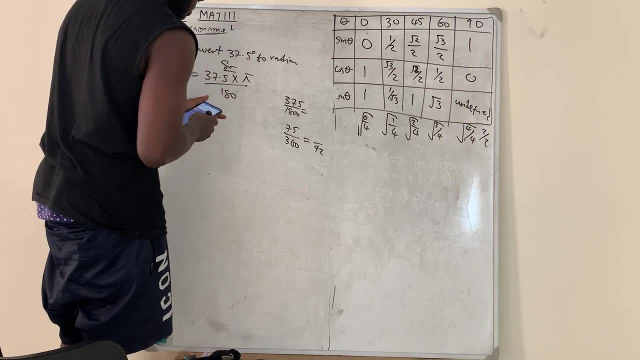 five again can divide divided by five. so i have 72, 72 five. so i have 72, 72 five. so i have 72, 72, 75 divided by five: i have 15.. so three. 75 divided by five: i have 15.. so three. 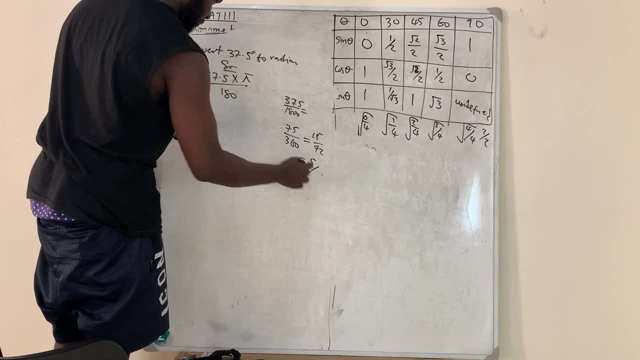 75 divided by five, i have 15.. so three can divide divided by three, i have five. can divide divided by three, i have five. can divide divided by three, i have five. over 72 divided by three, i have 24.. so, over 72 divided by three, i have 24.. so 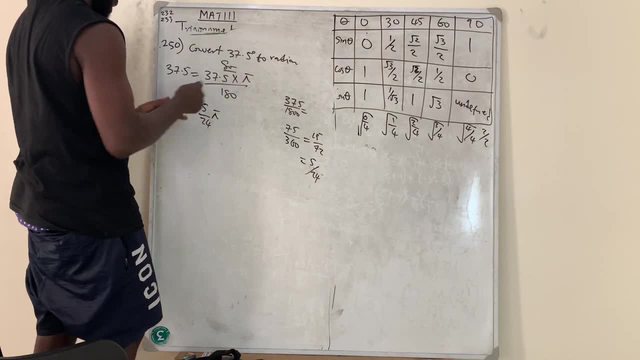 over 72. divided by three, i have 24.. so the answer is now. the answer is now. the answer is now: 5 over 24 pi. so that is what i mean by 5 over 24 pi. so that is what i mean by 5 over 24 pi. so that is what i mean by reducing it to the lowest. 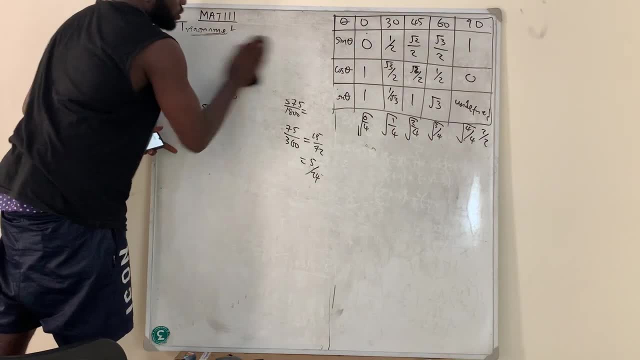 reducing it to the lowest. reducing it to the lowest. or 5 pi over 24- okay, so go to question. or 5 pi over 24- okay, so go to question. or 5 pi over 24- okay, so go to question number two, number two. number two: fifty one. question number two: five one. 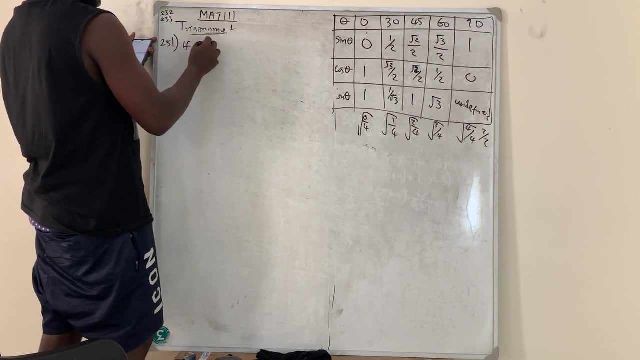 fifty one. question number two: five one. fifty one question number two: five one. question number two: five one. said question number two: if sine squared x, if sine squared x, if sine squared x, plus plus, plus sine x, sine x, sine x minus two is equal to zero. and then i say: 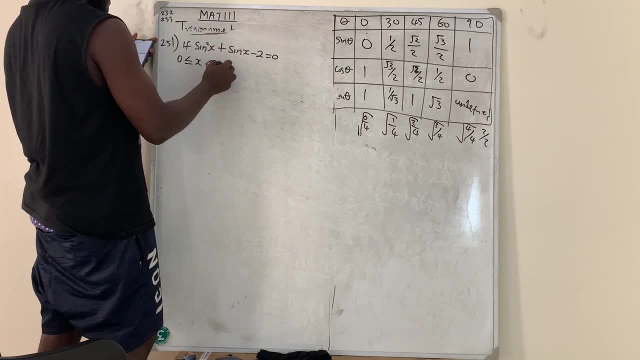 minus two is equal to zero. and then i say: minus two is equal to zero, and then i say: that that zero is less than or equal to x, that that zero is less than or equal to x, that that zero is less than or equal to x, which is less than or equal to pi, then 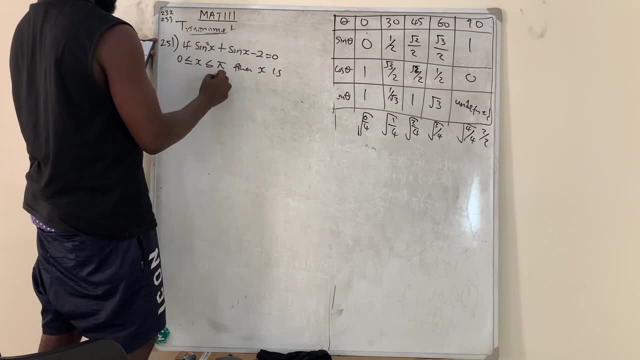 which is less than or equal to pi, then which is less than or equal to pi, then they now say: then they now say: then they now say: then x is, x is x is. solution. now, this is the pythagoras solution. now, this is the pythagoras. 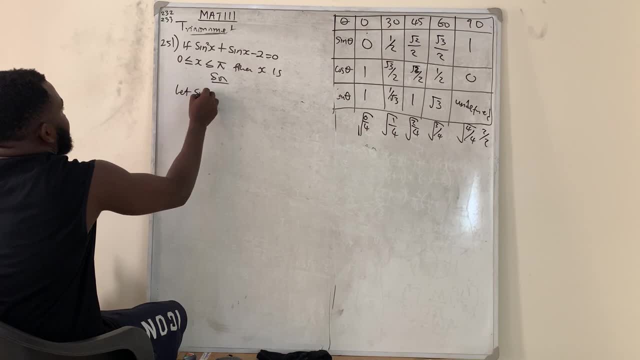 solution. now, this is the pythagoras, this is quadratic equation. so first, this is quadratic equation. so first, this is quadratic equation. so first thing you say is that let that sine x thing you say is that, let that sine x thing you say is that let that sine x equal to y. so anyway, you see, sine x. 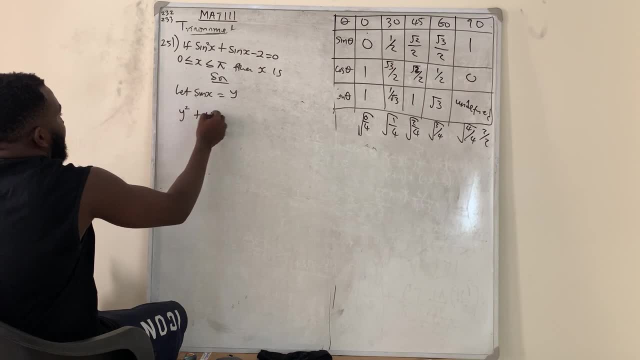 equal to y. so anyway, you see sine x equal to y. so anyway, you see sine x pitch y. so this will not be y squared pitch y. so this will not be y squared pitch y. so this will not be y squared plus y minus two is equal to zero. so if 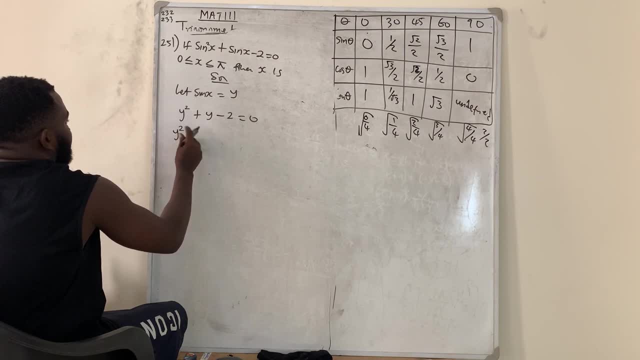 plus y minus two is equal to zero. so if plus y minus two is equal to zero. so if you factorize, i'm going to have y. you factorize, i'm going to have y. you factorize, i'm going to have y squared, squared, squared, uh. 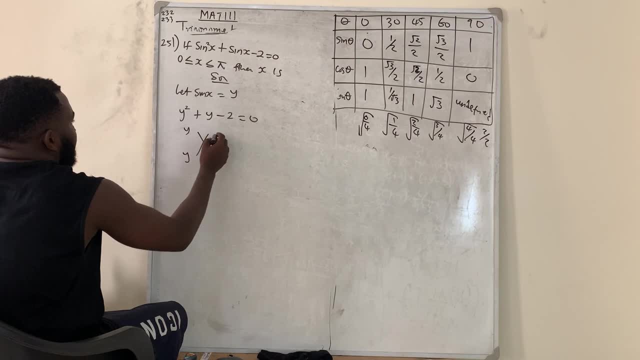 uh, uh. let me use this method so that it is y. let me use this method so that it is y. let me use this method so that it is y and y and y and y. minus two, sorry two and minus one. and if minus two, sorry two and minus one. and if 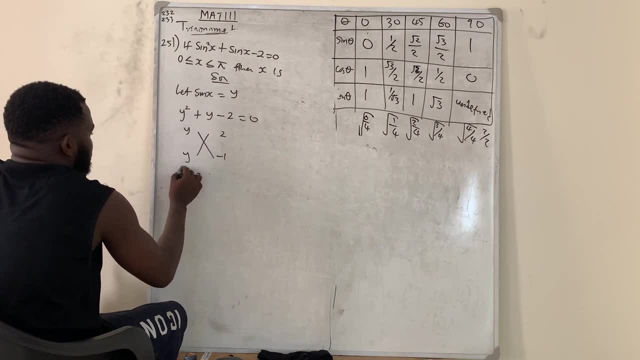 minus two, sorry, two and minus one. and if you check, you check, you check, we're going to get this. so i have that we're going to get this. so i have that we're going to get this. so i have that. y plus two, y plus two. 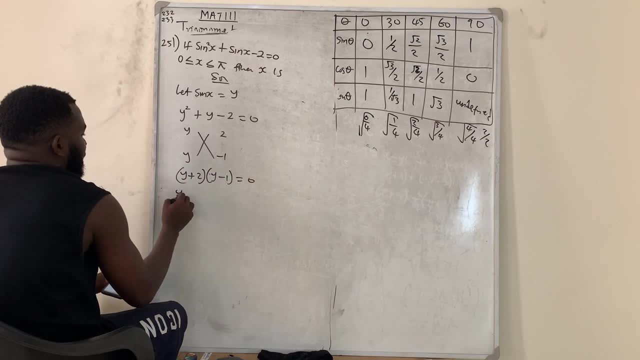 y plus two and y minus one is equal to zero. so i'm and y minus one is equal to zero, so i'm, and y minus one is equal to zero, so i'm, having that y minus having that y minus, having that y minus y is equal to, so you have the y plus two. 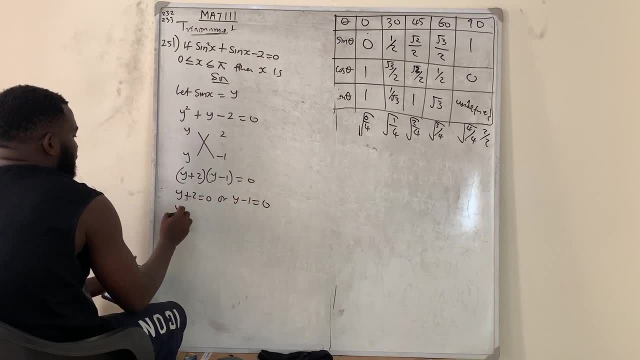 y is equal to, so you have the y plus two. y is equal to, so you have the y plus two. zero or zero, or zero or y minus one zero, so therefore y is equal y minus one zero. so therefore y is equal y minus one zero. so therefore y is equal to minus two or y is equal to one. but 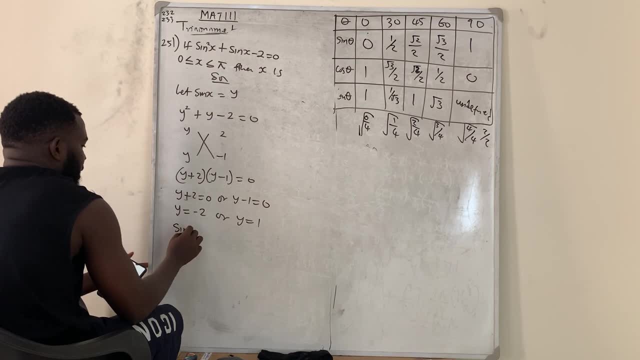 to minus two or y is equal to one, but to minus two or y is equal to one. but i'm not looking for y, i'm looking for x, i'm not looking for y, i'm looking for x, i'm not looking for y, i'm looking for x. so i'll say that sine x is equal to. 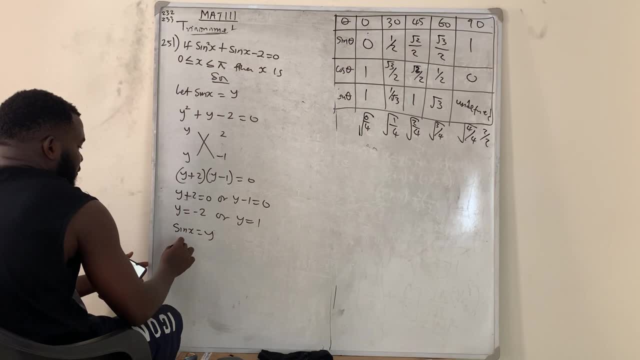 so i'll say that sine x is equal to. so i'll say that sine x is equal to minus two, minus two. minus two, so it's equal to y. so therefore, sine x, so it's equal to y. so therefore, sine x, so it's equal to y. so therefore, sine x is equal to minus two, or. 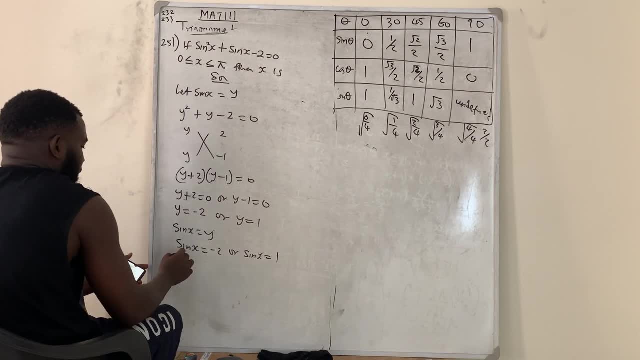 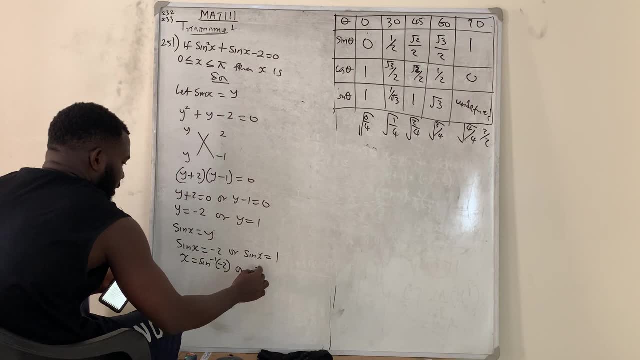 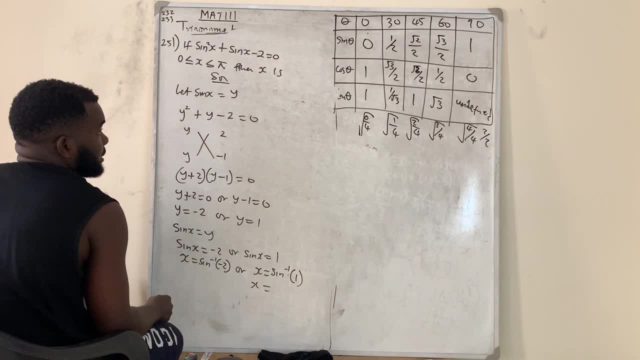 one, okay, one, okay. so sine inverse of one. so sine inverse of one. so sine inverse of one. uh, i'll give you 90 because i need to give. uh, i'll give you 90 because i need to give. uh, i'll give you 90 because i need to give you one. so here is 90 sine inverse of. 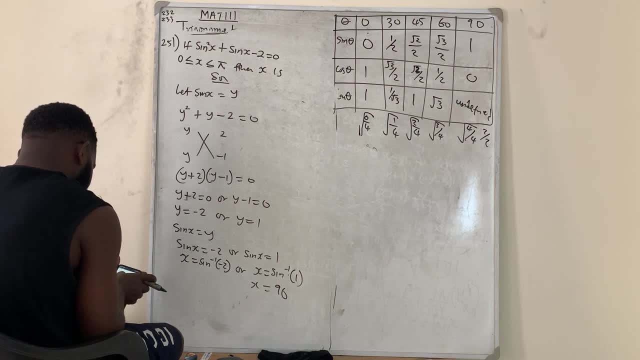 you one, so here is 90 sine inverse of you one, so here is 90 sine inverse of minus two. minus two, minus two: do we have sine inverse of minus two? do we have sine inverse of minus two? do we have sine inverse of minus two? shifts sine minus two. 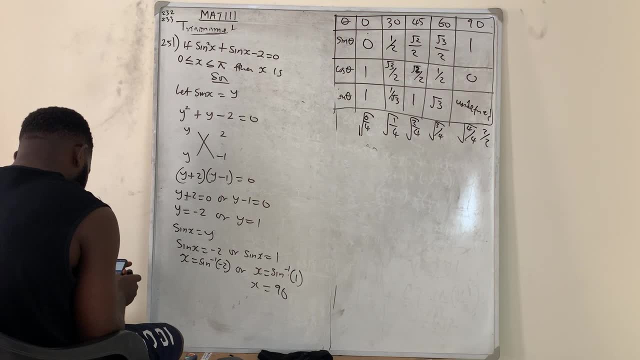 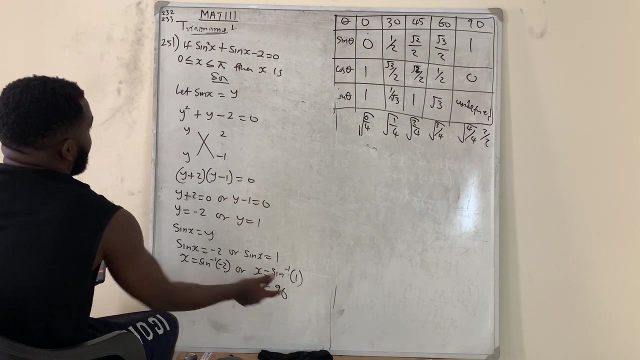 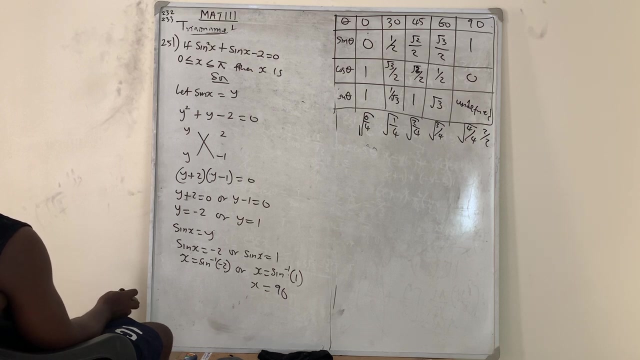 shifts sine minus two, shifts sine minus two. oh problem, okay, so i can't get the sine inverse of minus, so i can't get the sine inverse of minus, so i can't get the sine inverse of minus two. so two, so two. so i have that. this is 90. okay, but they said that theta falls from 0 to 180, so which other one can sign 180? 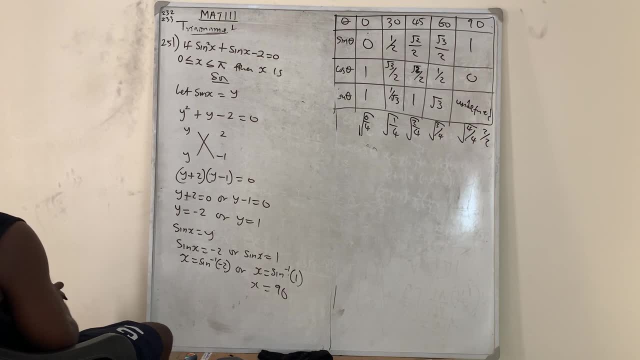 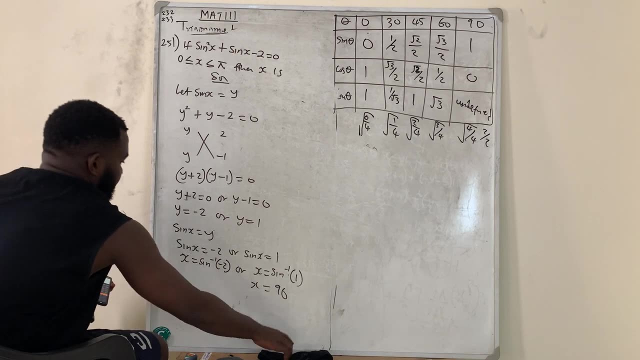 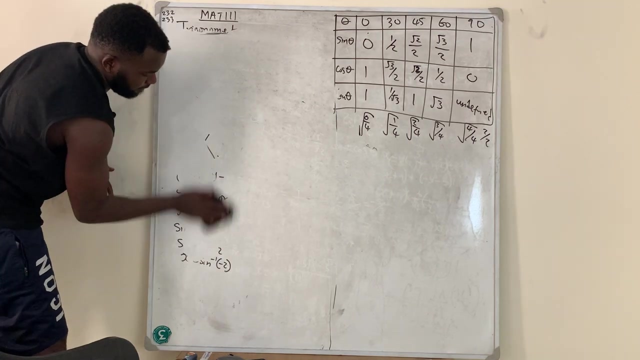 give us 1, let's check- sign 180, so it will not work. so theta and x is equal to what? 90 degrees? okay, so that is that x is equal to 90 degrees. so we move to the next question. so the next question here said question number. 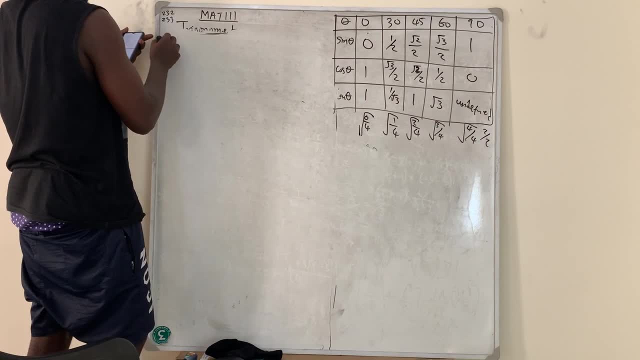 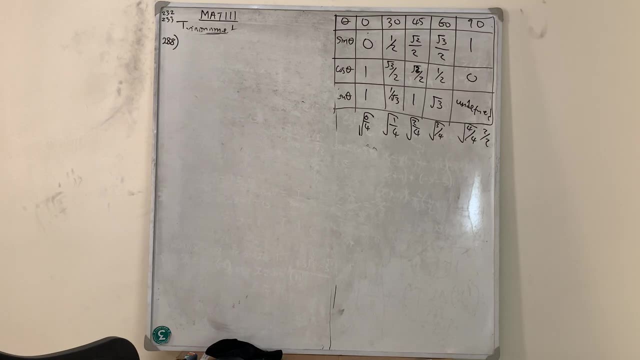 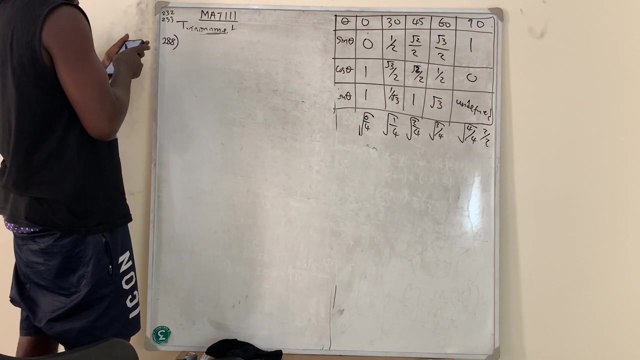 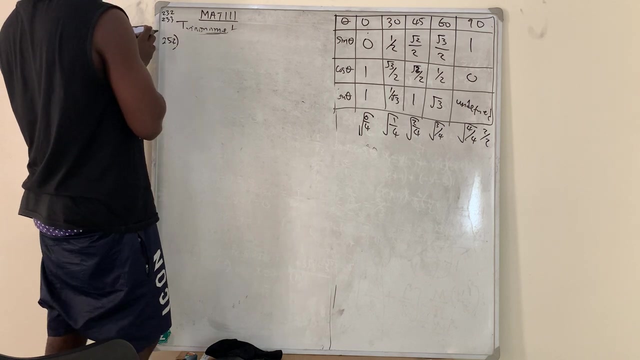 uh, 288, question number 288. let me keep checking. okay, yes, question number 288. this trigonometry is very much sorry, i've gone far. okay, so question number two: what? where am i? okay, 252, question number 252. so question number 252 said that if, if cos theta- sorry, if c. 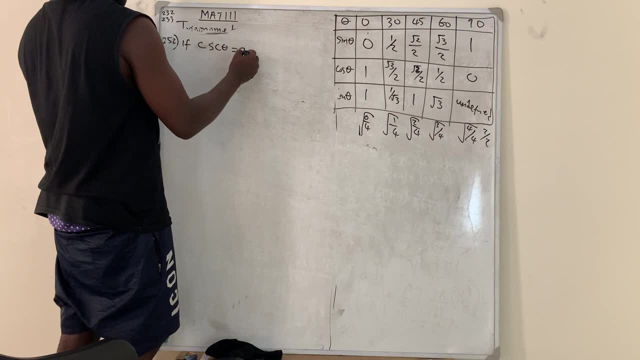 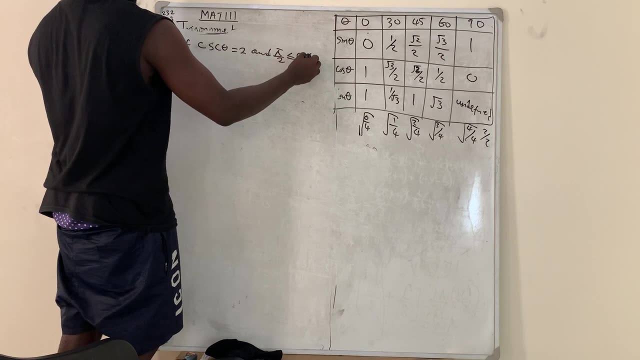 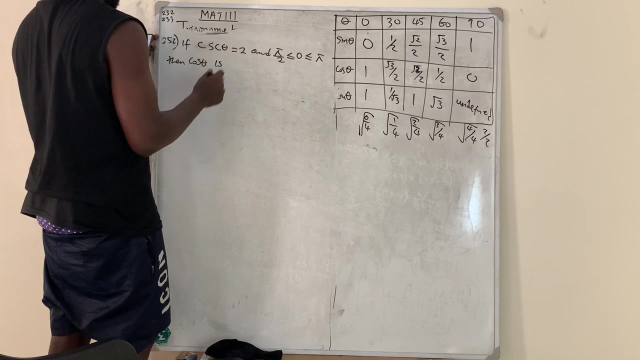 lc, theta is equal to 2 and and pi over 2 is less than or equal to 0, which is less than or equal to pi. then they now say with them: okay, then, cos theta is okay. so this is very, very simple. so first, the only problem is that they say: 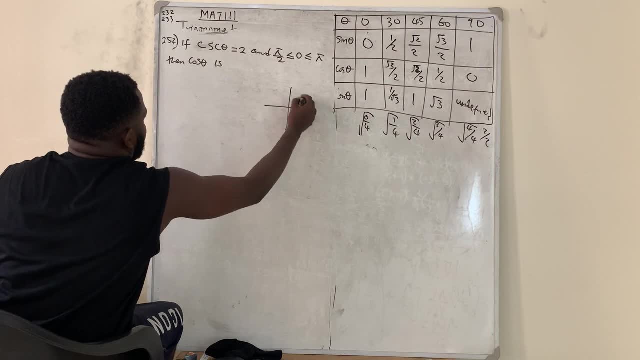 that it are forced between 90 to 180.. so if you draw your quadrant 0 to 90, then 90 to 180, so which means it's in this side. so if i draw this like this and cut this like this, so i have that here. 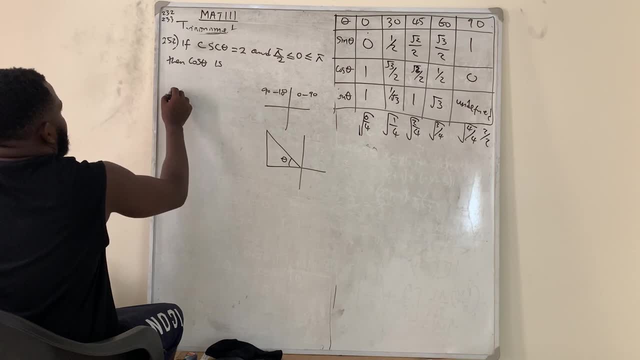 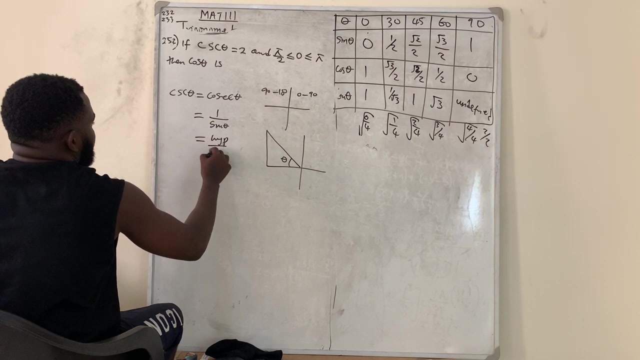 is my tita, so csc means ccc theta, so normally this means cosec theta. okay, and cosec is what one over sine, theta, which is what sine is opposite over hypotenuse, so it's going to be hypotenuse over opposite. okay, so my hypotenuse. 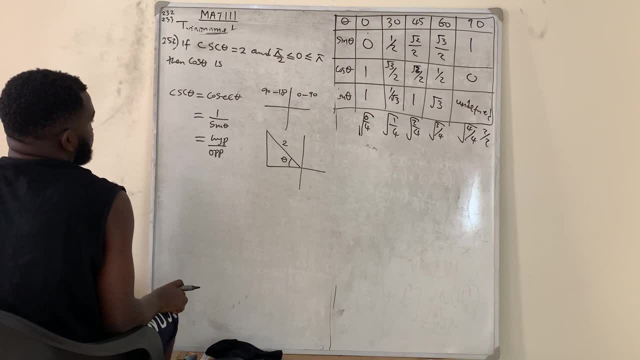 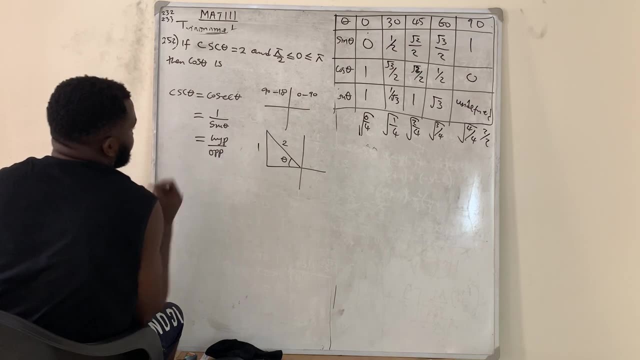 is now my two by my opposite is going to be one, so, but this is in the uh. okay, it's up here. so it's going to be one as well. so it's going to be one, okay. so, if i use my tagora's theory here, it's. 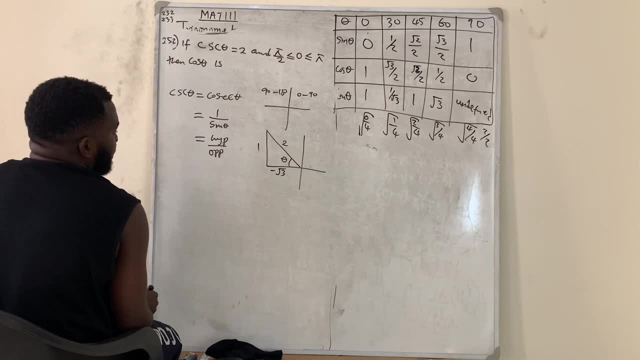 going to be minus root three. okay, so this is going to be minus three because it's in the negative. that's why it's minus three. so the last thing we should find cosec, theta, cosec- is what adjacent over what hypotenuse so adjacent is going to be. my adjacent is minus root three over what hypotenuse. 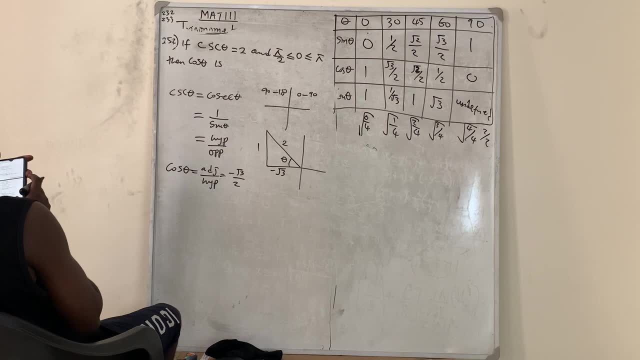 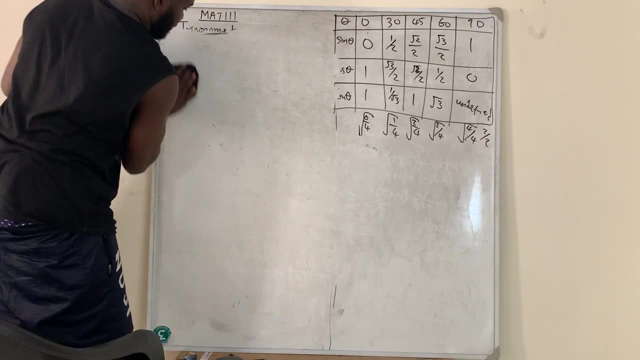 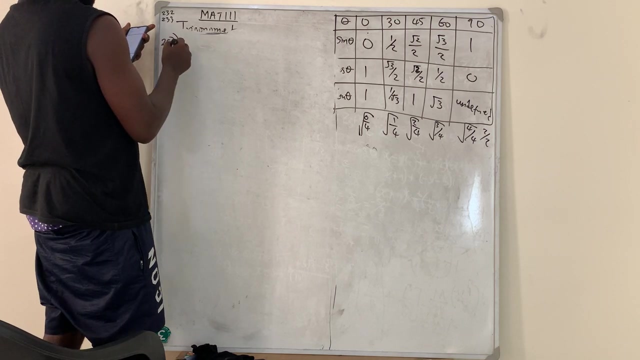 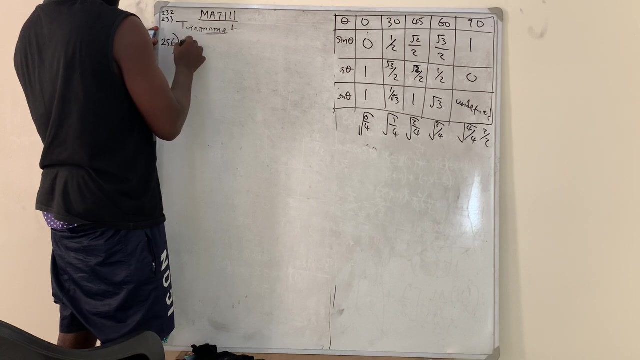 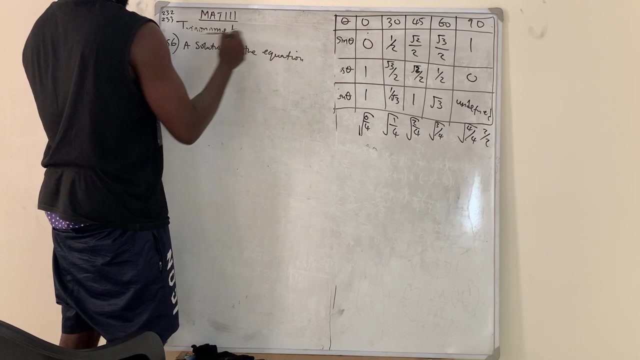 two. so minus root, three over two is my answer. that is option c. so we move to the question number 253. so question number 253, 253. question number 253 said: okay, no 253, so 256. question number 256 said: a solution, a solution to the equation, a solution to the equation sine. 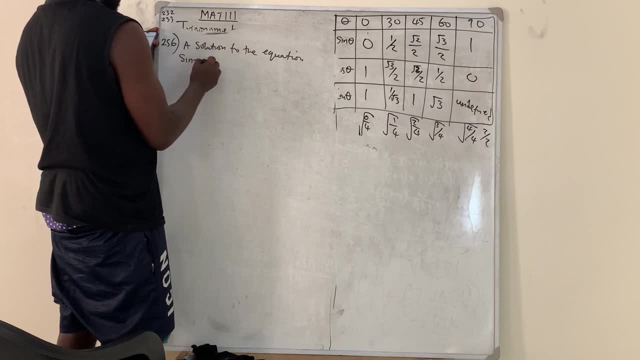 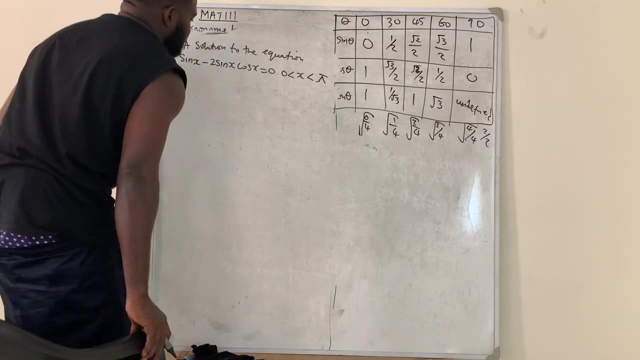 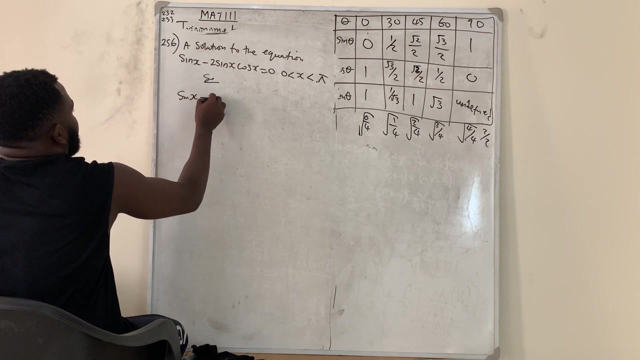 sine x minus two, sine x, cos x is equal to zero, as zero lies between zero and nine and one eight, as s lies between zero and one eight. okay, we have solved this question before, so i've solved this question before. so what did the solution they gave you? that sine x minus two, sine x, cos x is equal to zero. so if you factorize, 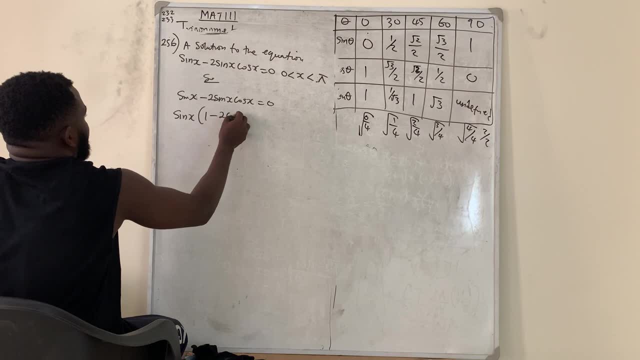 are going to have sine x in bracket of one minus two cos x is equal to zero. so i'm going to say that that's sine x is equal to zero. or one minus two cos x is equal to zero. so therefore, two cos x is equal to. 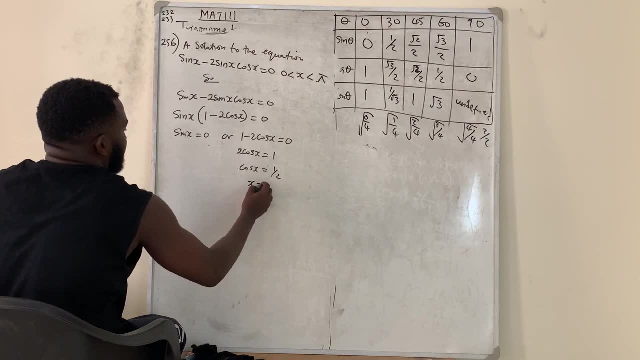 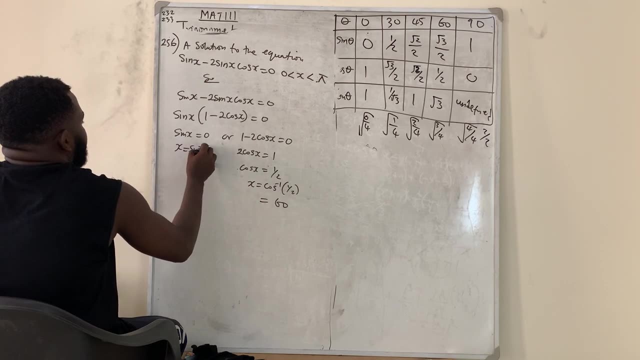 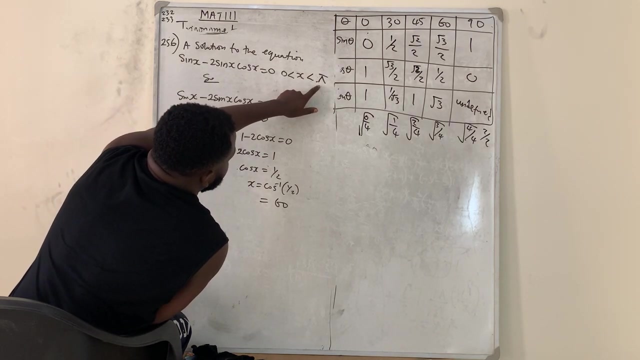 one and the cos x is equal to half, so therefore x will now be the cost inverse of half, so and cost inverse of half is 60, so but here x is equal to what? the sine inverse of zero? sine inverse of zero is zero. but they say that x lie between zero and 180, but zero is not among, because it is less than. 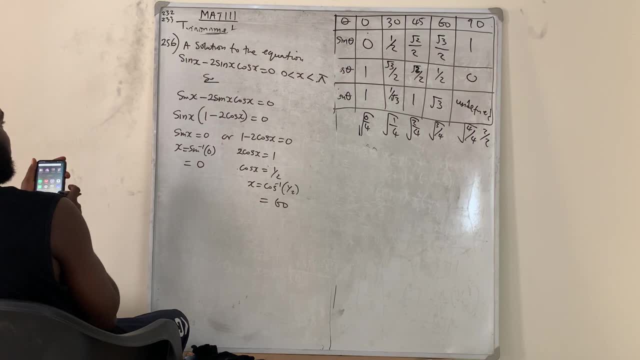 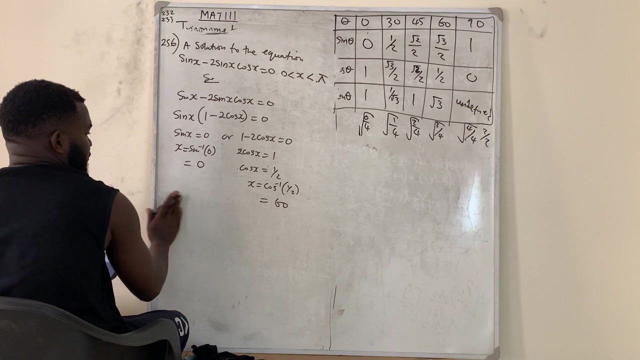 equal to here. so zero is not among. find any other thing that can give you, uh, um, what zero sin 90 is one. sine 270 is minus one. sine sine 180 is zero. so so my x is equal. the first number is one. okay, they say that is less than 180. so 180 is not even among. so the only answer here is just 60. 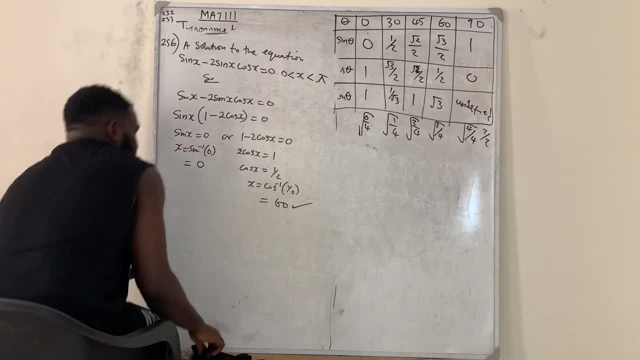 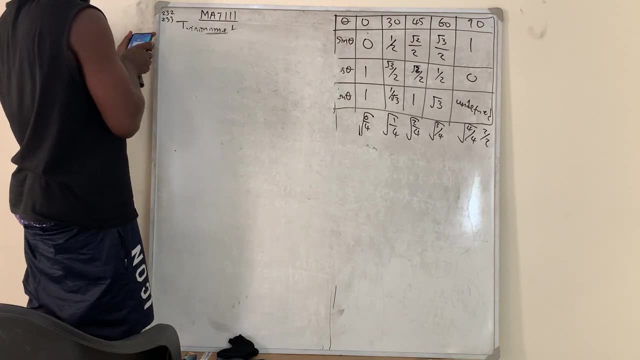 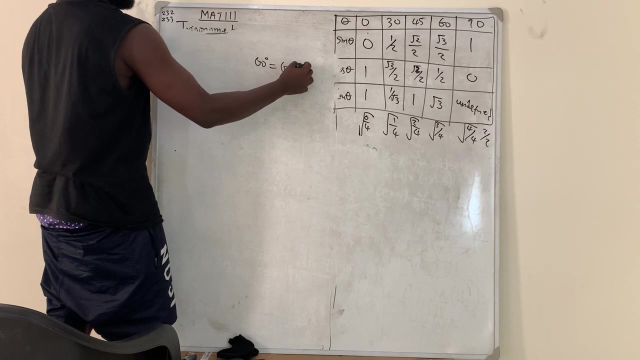 so my x is just 60. so 60 is the only answer for this particular one. okay, so we move to the next question, question number. so and 60? okay, their own is in radian. 60 degrees converted to radian is 60 times times pi divided by 180. so reduce this one to the lowest. so if you say 180 divided by 60, 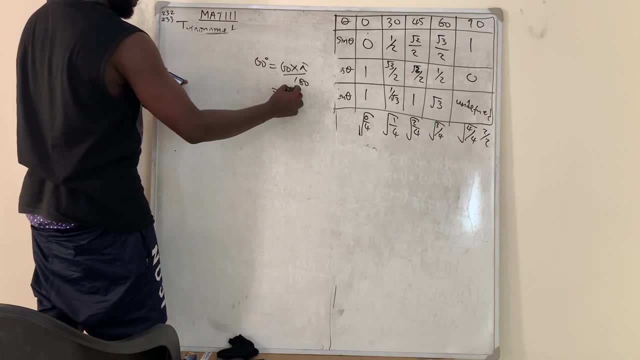 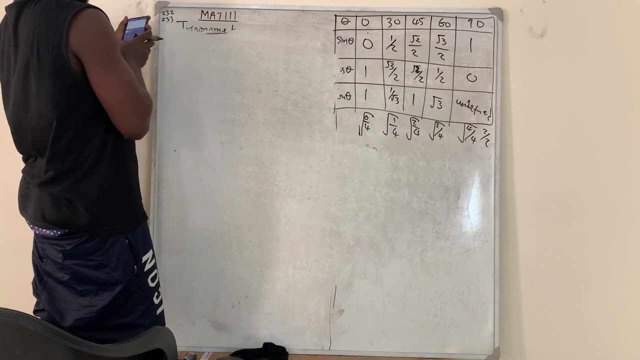 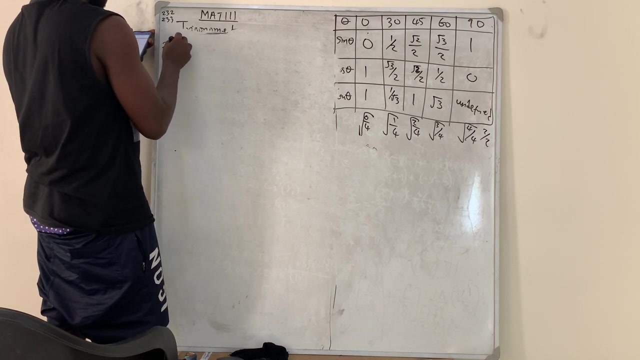 180 divided by 60, so 3, that is pi over 3. so the answer there is pi over 3. pi over 3 is 10 to the 60. all right, so the next question is question number. here is it 2, 5, 8? okay question. 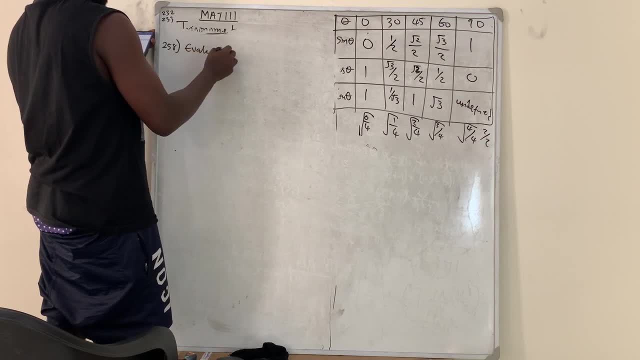 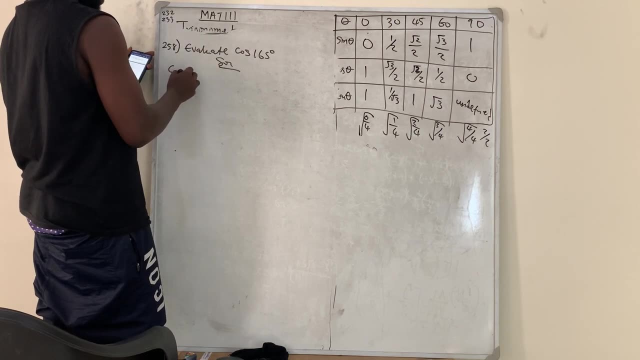 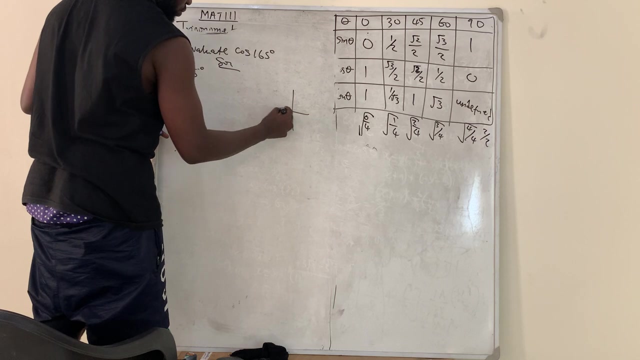 number 2, 5 says: said: evaluate, evaluate cos 165 degrees. all right solution. now cos 165 degrees. 165 is in what quadrant? 165 is in what quadrant? that's what you check, from 0 to 90, 90 to 180, and i have cast so cost is even negative in the second quadrant. so it's negative. so i'm going. 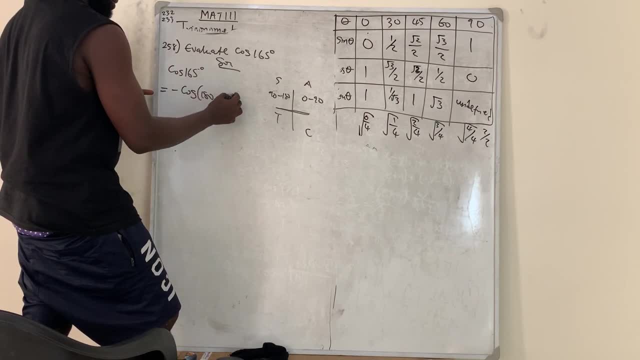 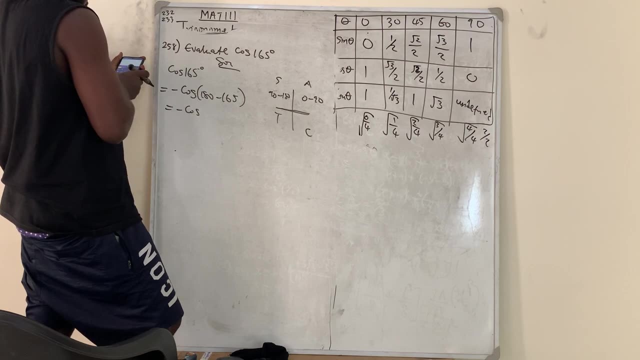 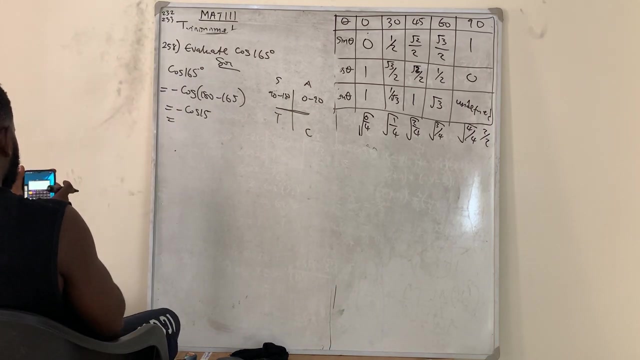 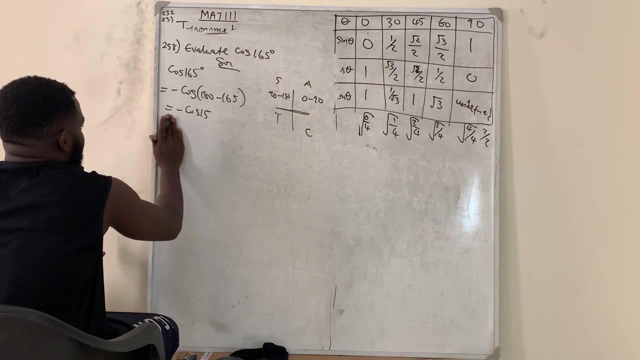 to have negative cos 180 minus 165. so i'm going to have minus cos. check it: 180 minus 165. so i have 15. okay, so, um, let me check if it is um an option question. okay, cos 15. the same thing we did before. let us do it again. so, cos 15, give you minus. cos 15 is. 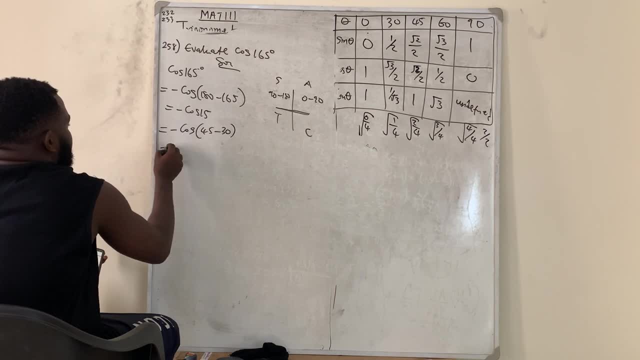 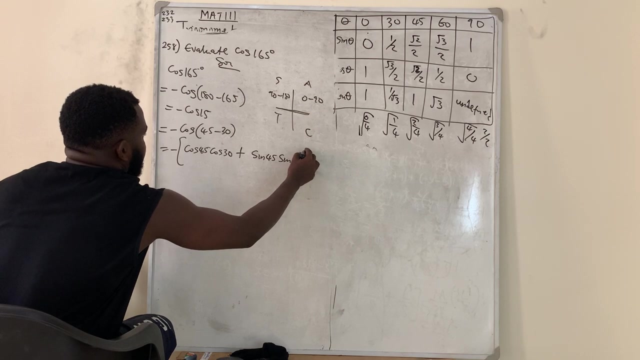 the same as saying 45 minus 30.. all right, which is what? minus into cos 15 means cos 45 cos 30.. if this minus here is going to be plus cos sorry, plus sine 45, sine 30. all right, so i'm going to have that this is minus into, this is root. 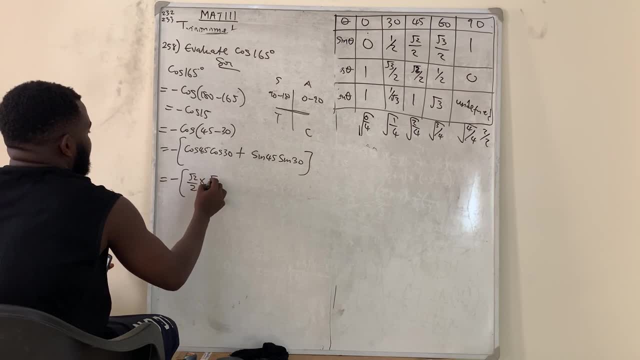 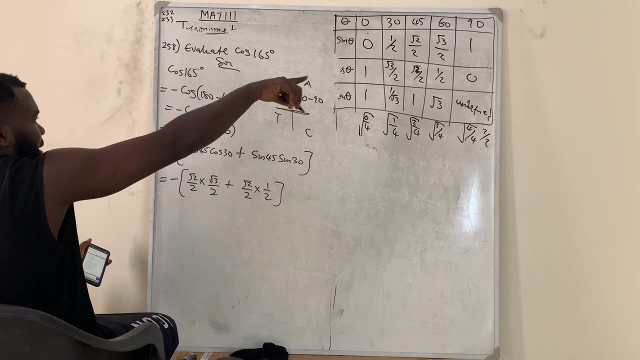 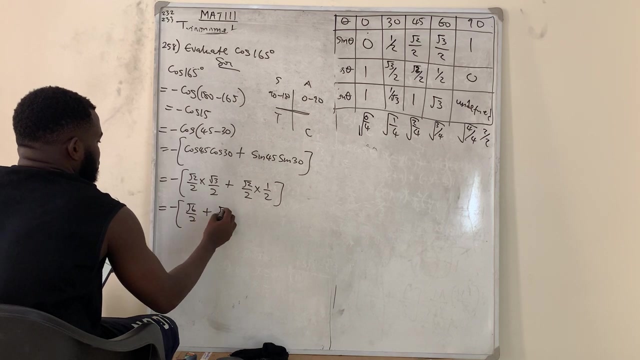 2 over 2 times root 3 over 2 plus root 2 over 2 times 1 over 2. according to that. uh, this, this stuff here, so i'm going to have that. this is what root 6 over 2 plus root 2- sorry, over 4 plus root 2. 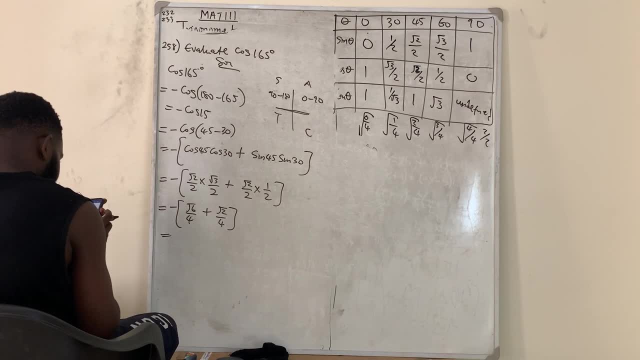 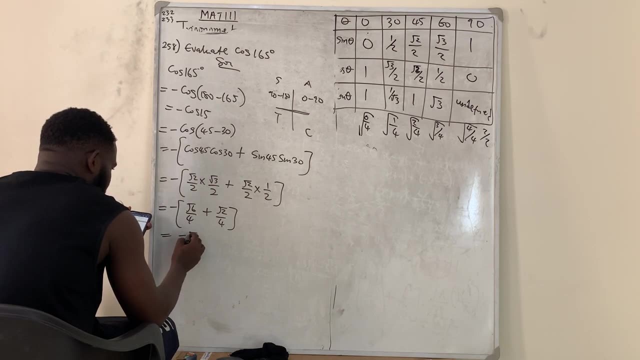 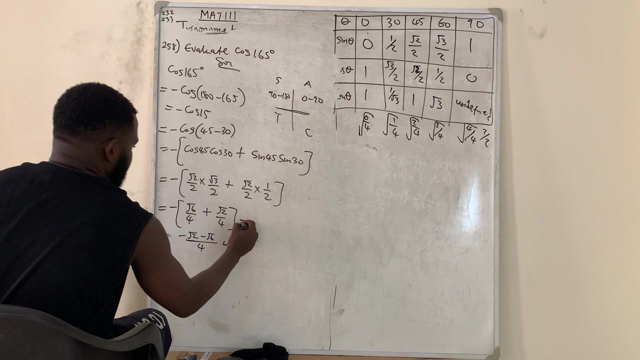 over 4.. okay, so let me check the option they have there. so if i open this bracket, it's going to be according to the their option: minus root 2 over. minus root 2, minus root 6- everybody over 4.. so that is this according to lcf, because this is. 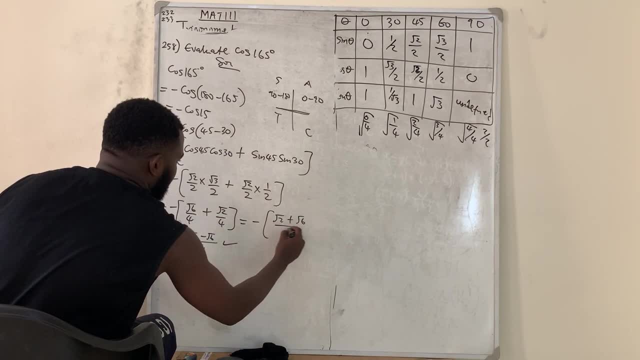 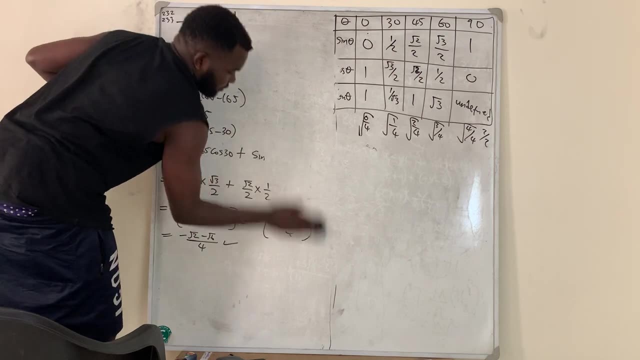 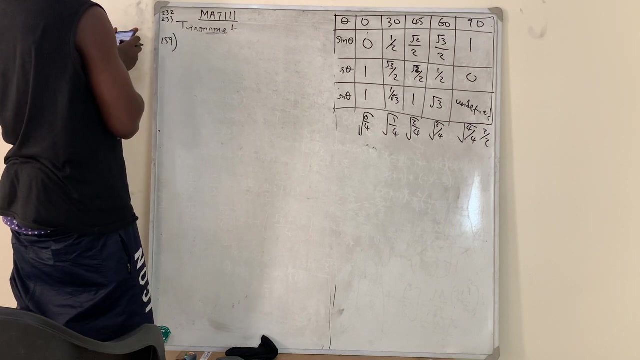 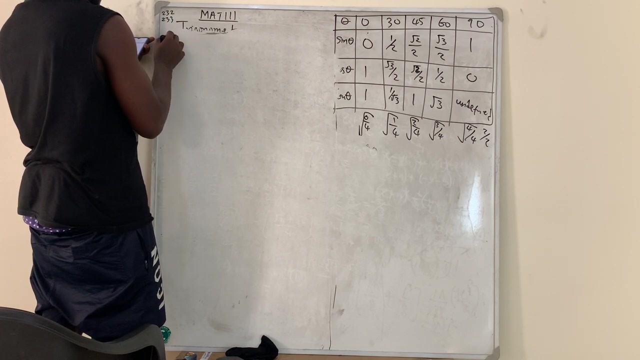 minus into root 2 plus root 6, all over 4.. so if you open the bracket with the minus, you have this as your answer. so we'll go to question number 159.. okay, question number 159 said. okay, no question number 159, but question number 262. sorry, 262.. 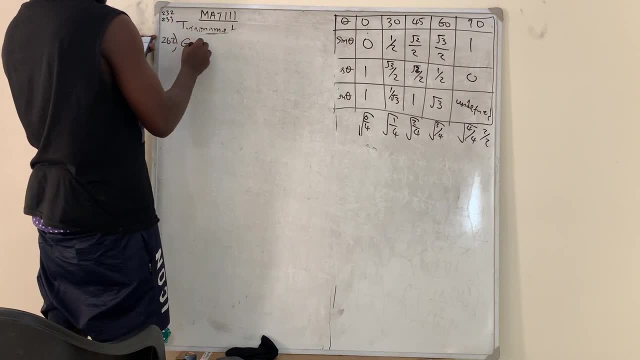 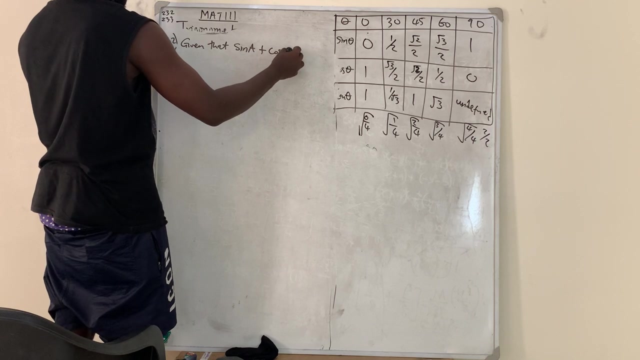 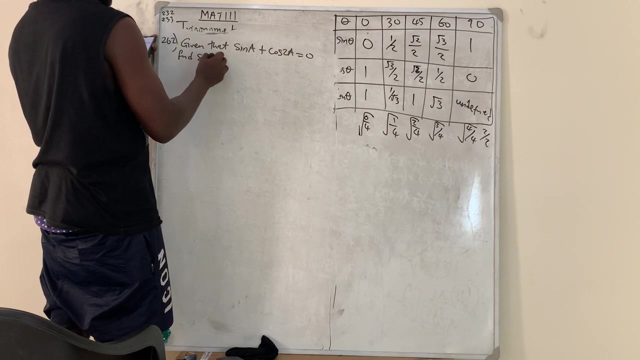 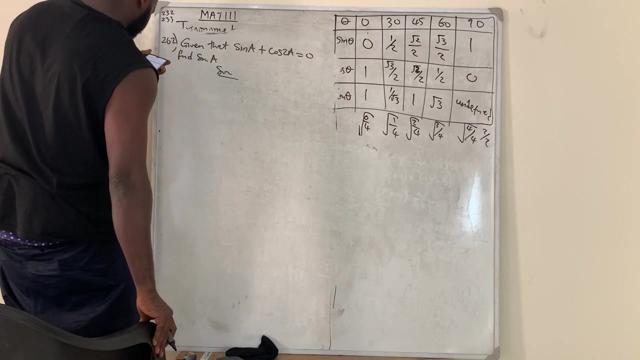 okay. 262 said: given that, given that cos, given that sign, sign a plus cos 2a is equal to 0. Then they now say: find sine a Solution. First of all we need to find a before finding the sine a. Okay, So now. 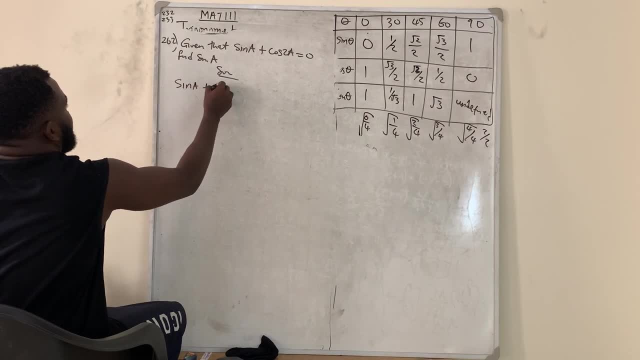 if you look at this, they gave us that sine a plus. what Cos 2a is equal to 0. But you should know that according to trigonometry, that cos 2a is equal to what Is equal to cos squared a minus. 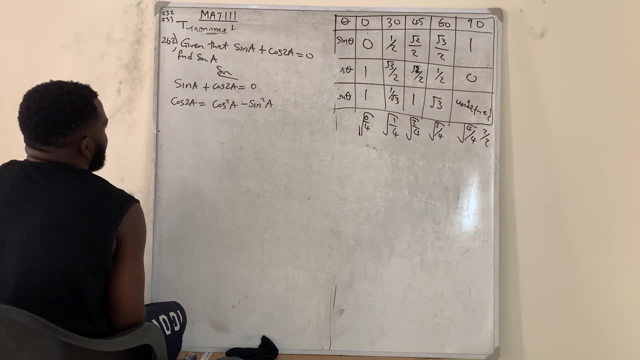 sine squared a. Okay So, but I want everybody to be in sine. So if everybody is going to be in sine, so it's going to be that. convert this one to sine Cos squared theta. you should know that cos squared a is equal to 1 minus. 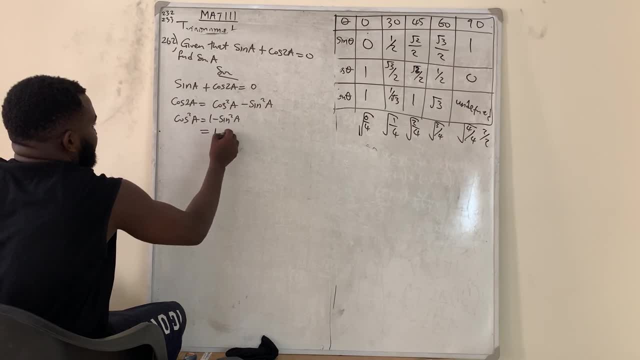 sine squared a. So instead of putting this thing, you now put it as 1 minus. so cos 2a, 2a is equal to this. one will change to 1 minus sine squared a, then minus another sine squared a, So which? 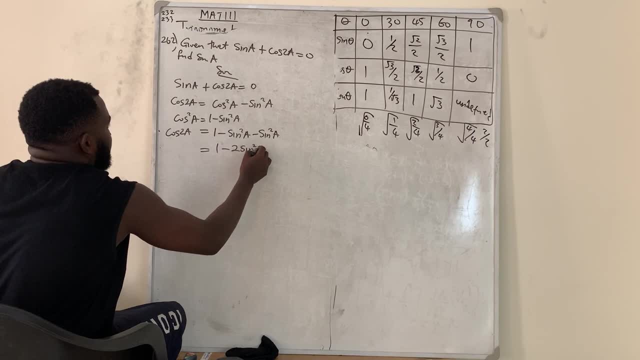 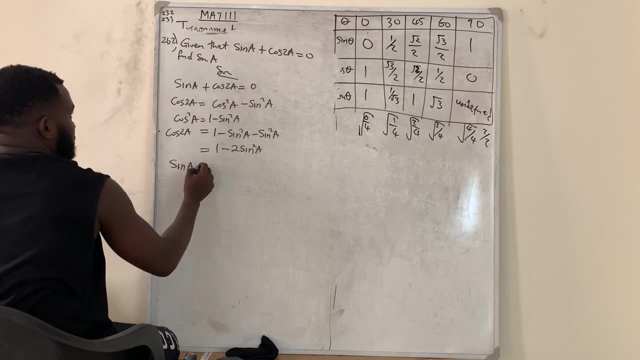 will give you 1 minus 2 sine squared a, So we now put it in that equation. So my equation said: what Sine a. Instead of putting this one, I'll put it as: what Plus 1 minus 2 sine squared a is equal to 0.. So 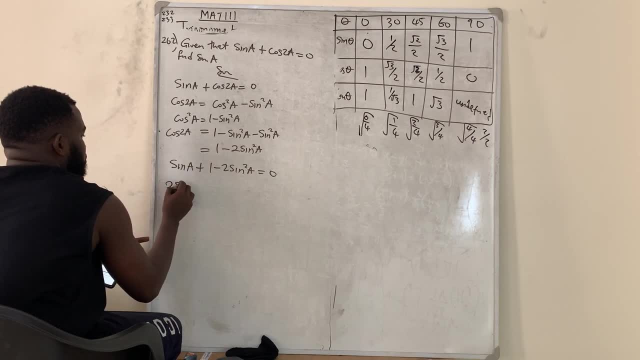 if you arrange it very well, this one moving to this side, I'm going to have 2 sine squared, a minus sine a, then minus 1.. Everybody moving to this side is equal to 0.. Okay, So now this is a quadratic equation. 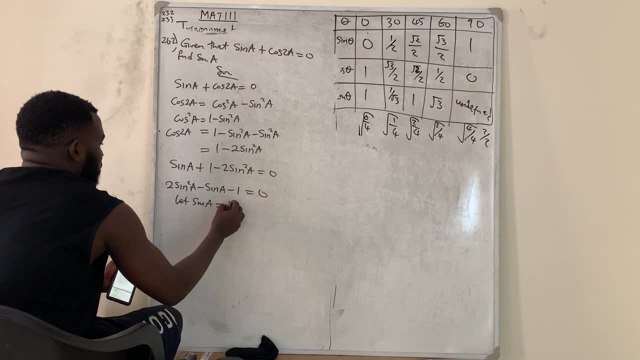 So I'll say: let sine a be equal to what y. So anywhere I see this, I'll put. or let me say: let it be equal to x, I love x. So I'm going to say: 2x squared minus x minus 1 is equal to 0.. So if I factorize, I'm going to. 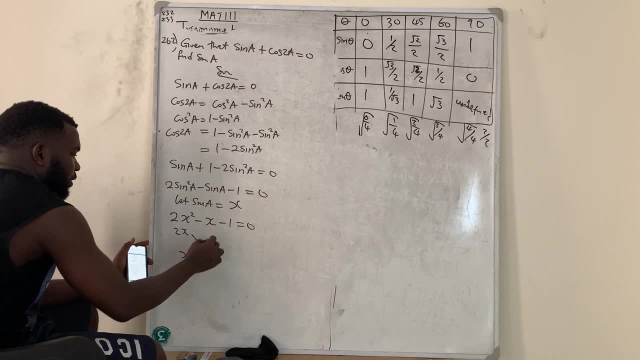 have 2x here and x, So I'm going to have minus 1 and 1.. So if you're going to check, you say that 2x plus 1 and x minus 1 is equal to 0.. So therefore, 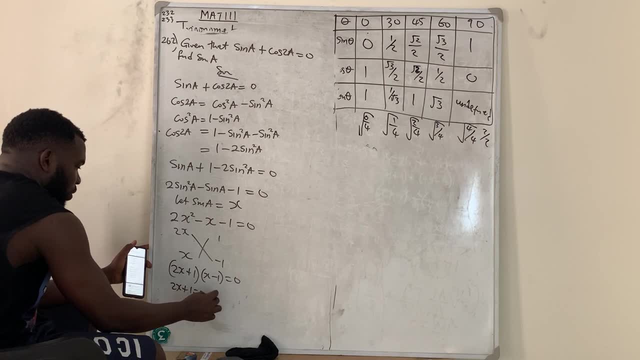 2x plus 1 is equal to 0, or x minus 1 is equal to 0. So, therefore, x is equal to minus 1 over 2, or x is equal to what 1.. So therefore, we have said that sine a is equal to 1 over 2.. So therefore, 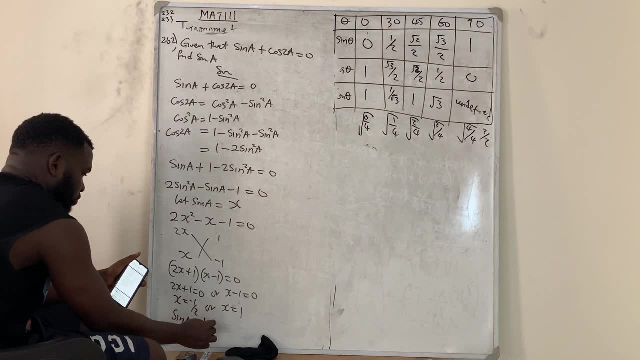 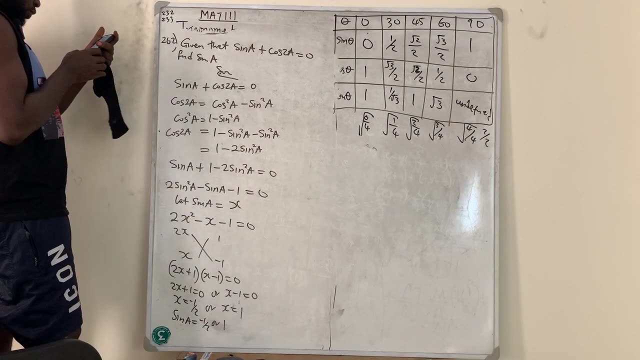 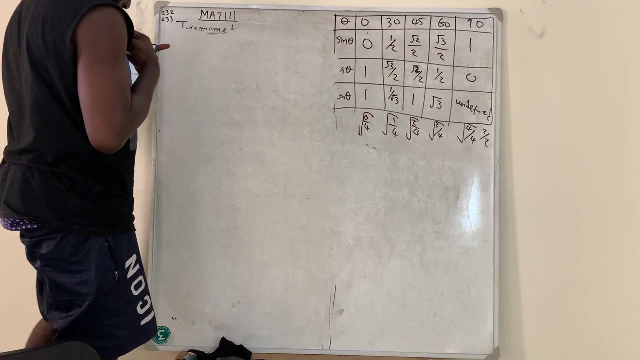 sine a is equal to either minus 1 over 2 or 1.. So that is that or that. Let's go to the next question, Question number 162.. Now 163.. Question number 163, 263.. Question number 263.. 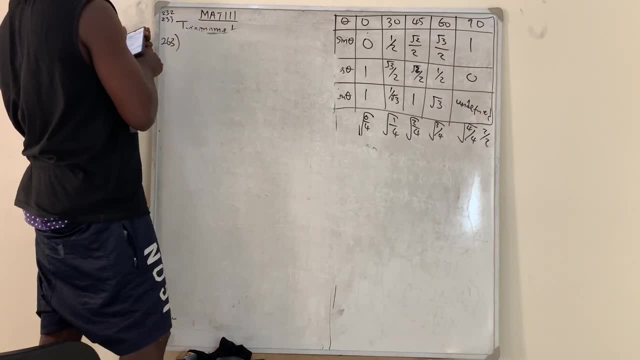 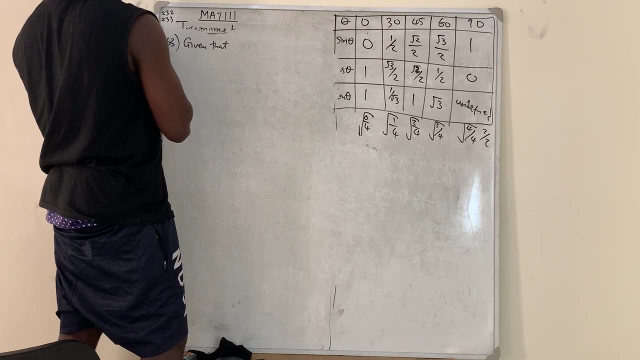 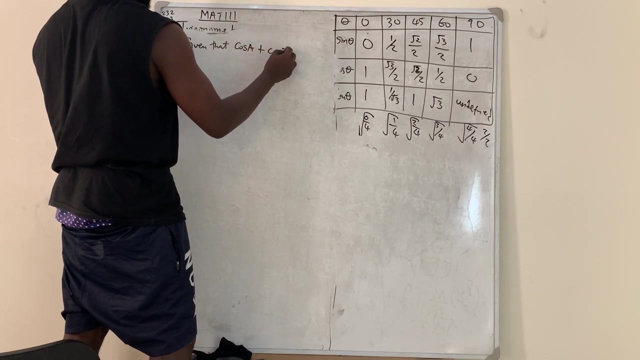 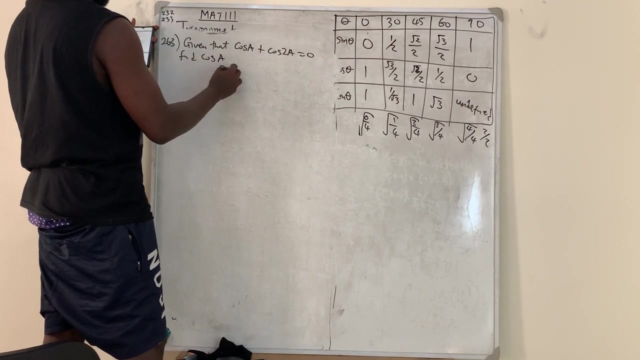 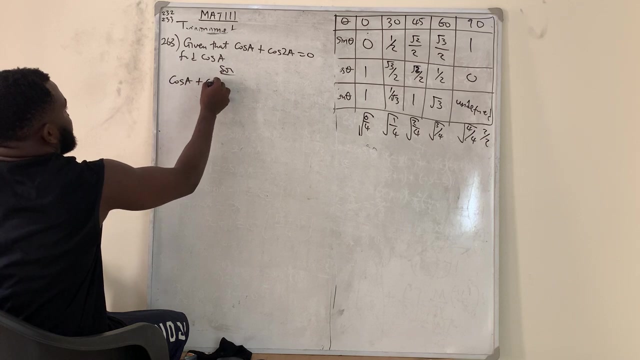 So then, given that 163 said: given that that that cos a plus cos 2a is equal to 0. Then I say: find cos a Okay Solution. The same method is applied here again. So they gave us that cos a plus cos 2a is equal to 0.. 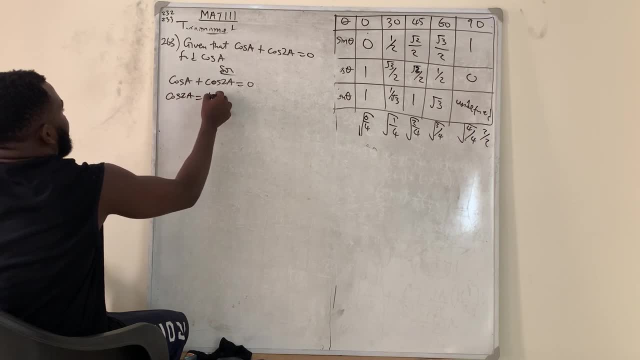 I told you before that cos 2a is equal to what 1 minus sorry, is equal to cos squared a minus, sine squared a Right. So but I want everybody to be in cos. I want everybody to be in cos. 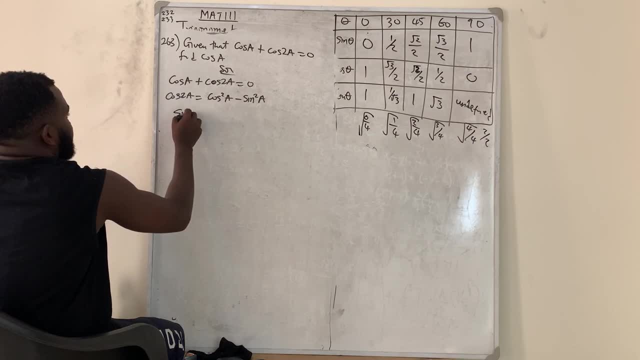 So it's going to be convert this one. You should know that sine squared a is equal to 1 minus cos squared a. Okay, So if you now put it, you are going to have that cos 2a is equal to bring down this one. 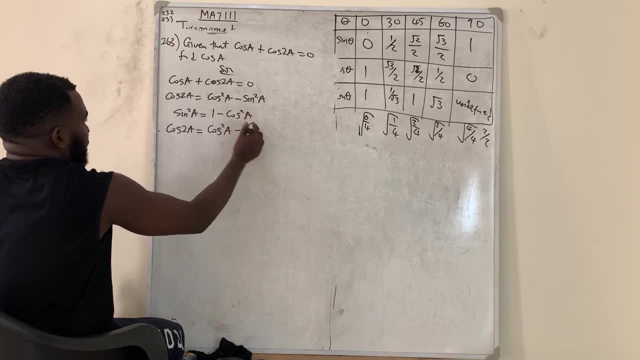 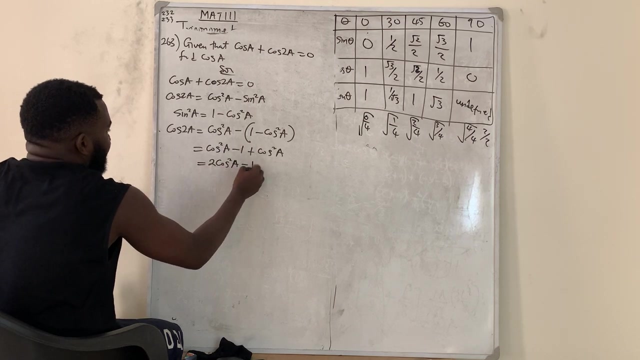 cos squared a minus into. Instead of writing these people, I'm going to write 1 minus cos squared a. Okay, So this is equal to cos squared a minus 1 plus cos squared a, So I'm going to have that this is 2 cos squared a minus 1.. 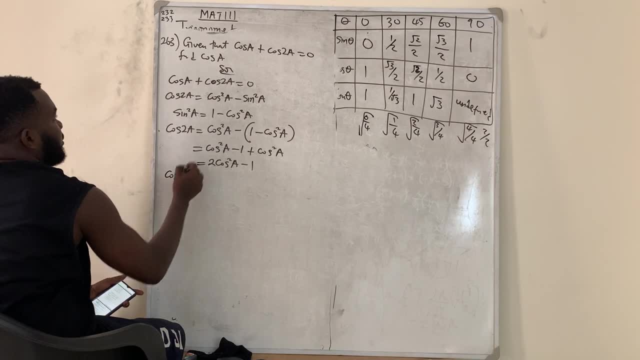 So put it back in your equation to have that what Cos a? Instead of writing this one, I'm going to put it as well: 2 cos squared a minus 1 is equal to 0.. So I already got it. I have that 2 cos squared a plus cos a. 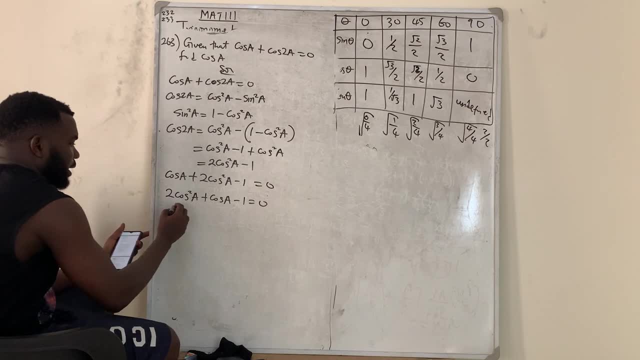 Minus 1 is equal to 0. So this is a quadratic equation. I can say that let that cos a be equal to what x. So you have 2x squared plus x minus 1 is equal to 0. So if I solve this way, 2x and x. 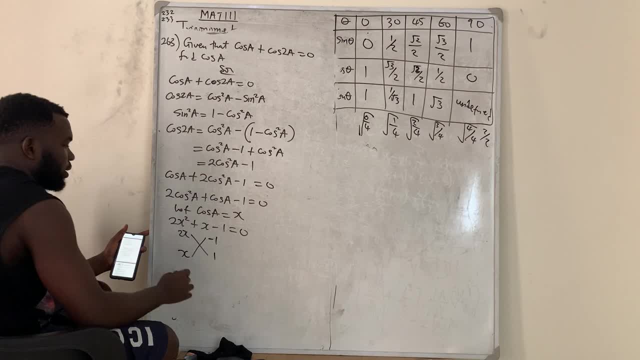 So I'm going to have minus 1 and 1.. So if I cross multiply, I'm going to have this. So, since that, I'm going to have that 2x minus 1 and x plus 1 is equal to 0.. 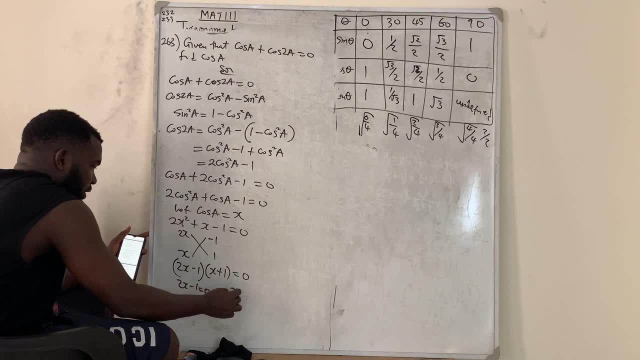 So therefore, 2x minus 1.. x plus 1 is 0 or x plus 1 is 0. So therefore, x is equal to what? 1 over 2 or minus 1.. So, since we have said that cos a is equal to x, 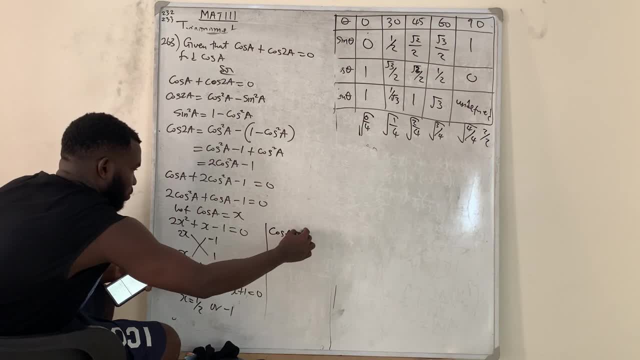 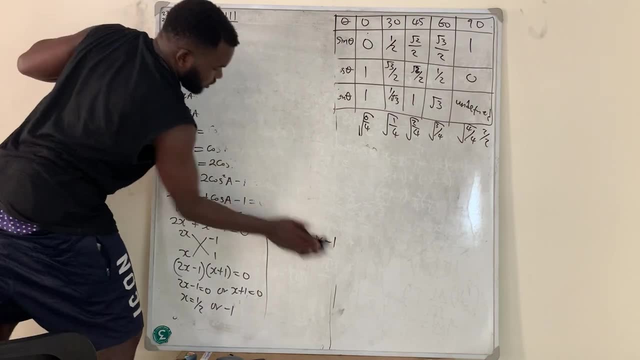 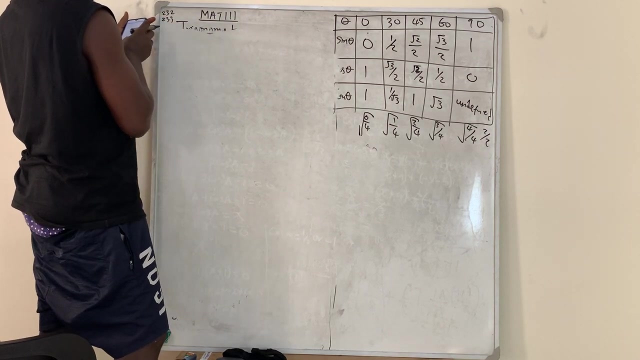 Okay, So therefore, cos a is equal to 1 over 2 or minus 1.. So that is that for now. So we'll move to the next question, which is question number. Question number: Where am I? Question number 264.. 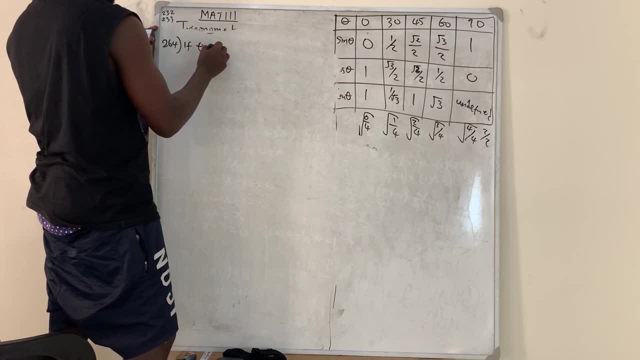 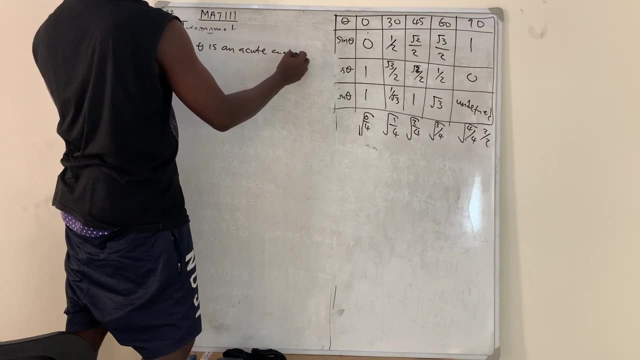 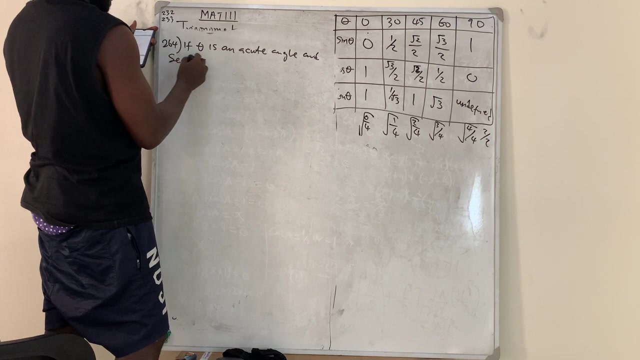 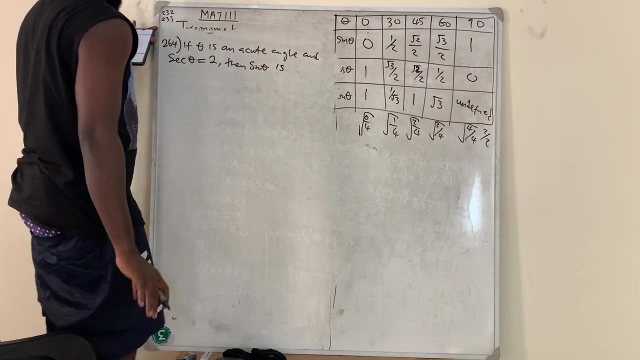 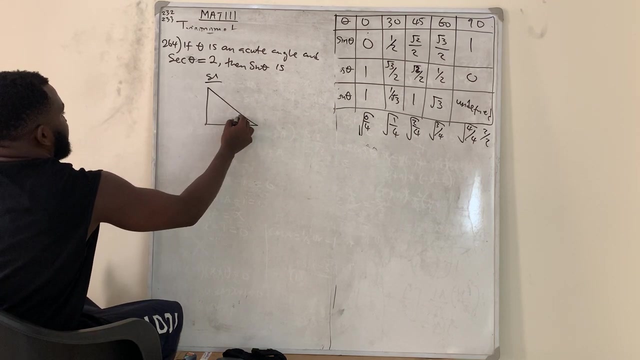 Question number 264 said: if theta is an acute angle and the sec theta is equal to 2, then sine theta, What is Okay? So this is a very simple question Solution. We are going to draw. If I draw, I'm going to have that. here is my theta. 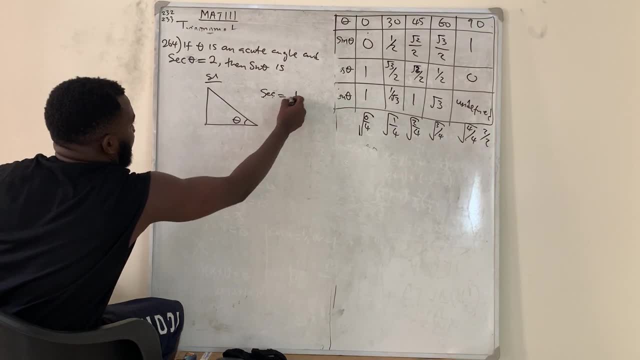 And I told you that sec, Sec is equal to 1 to the 1 over cos, Cos, theta, Which is what Supposed to be adjacent to the hypotenuse. So it's going to be hypotenuse over adjacent. So which is what? 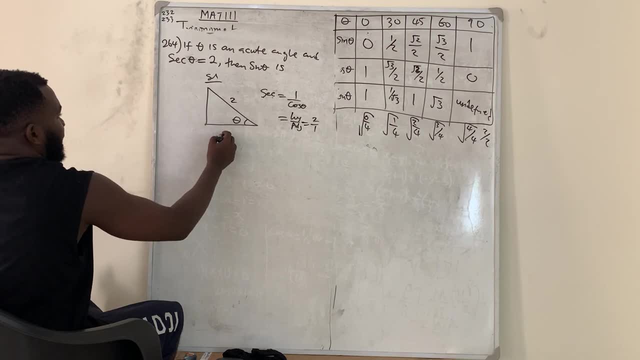 We will give it as 2 over 1.. So my hypotenuse is 2 and my adjacent is 1.. So here it's going to be with 3.. So therefore, sine theta will not be what Opposite with 3 over hypotenuse 2.. 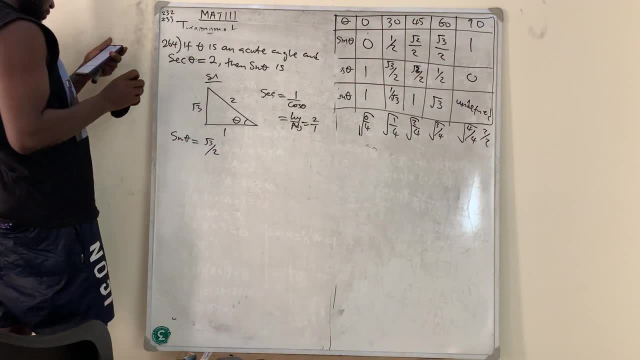 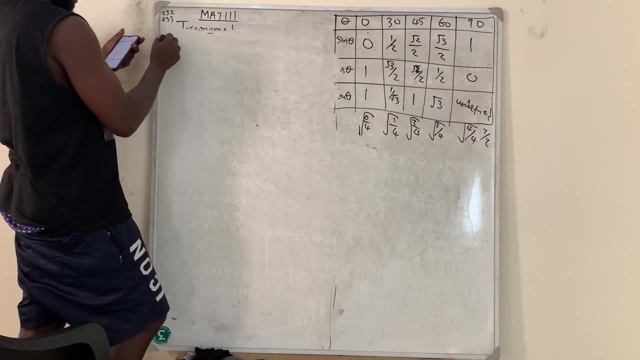 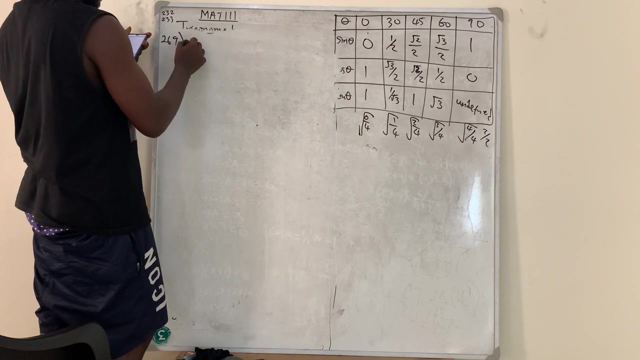 So my answer is with 3 over 2.. Okay, We'll move to the next question, Question number 625.. 265.. Question number 26.. Okay, They don't have 265.. They say 269.. And 269 said that if theta. 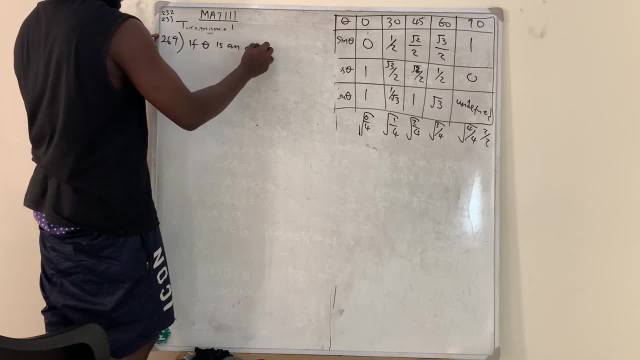 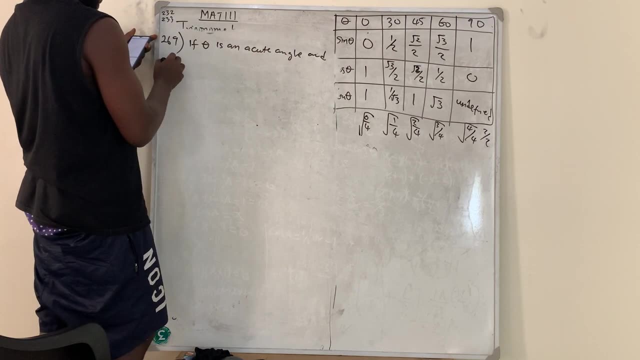 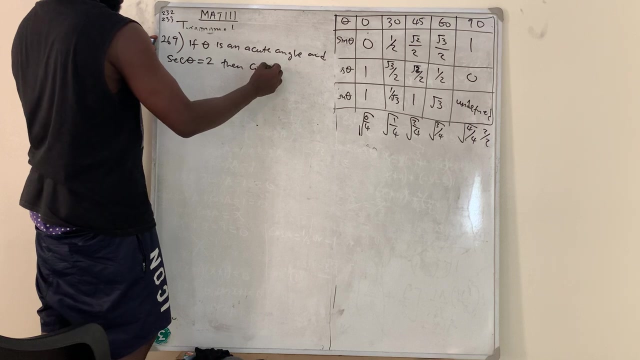 If theta is an acute angle, again Acute Angle 269.. And And sec Theta is equal to 2.. Then they now say: then If you find cos 2 theta, Okay, All right Solution. The same thing is applicable again. 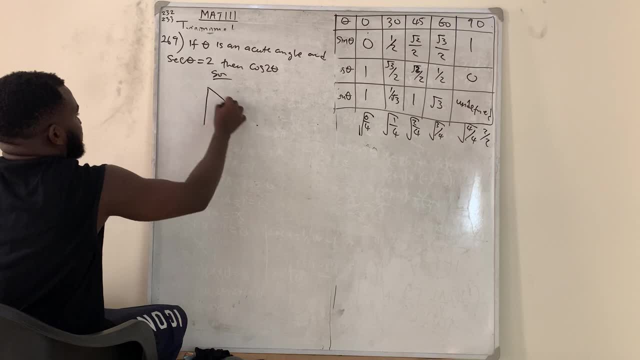 The way we did it before. Let's repeat again. So we have that According to what we did that time. Don't forget that. we have that. here is theta. We got that. here is 2.. Here is 1. And here. 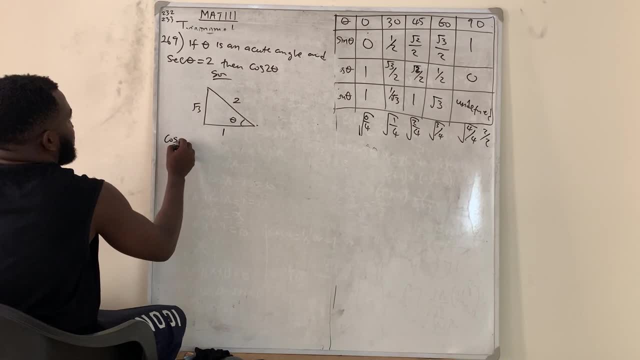 Is root 3.. Don't forget. So therefore we have that. cos Cos 2 theta Means Cos 2 theta, Don't forget, is what. Cos square theta Minus sine square theta. Okay, And cos is what? 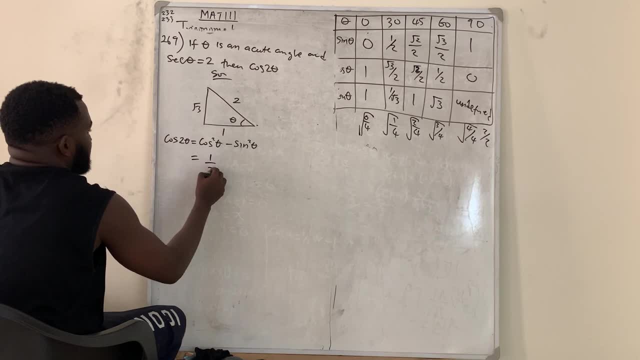 Opposite And adjacent over hypotenuse is 1 over 2.. This has squared, All squared, Minus Opposite over hypotenuse. What is what Root? 3. Over 2. All squared. So this one is giving me 1 over 4.. 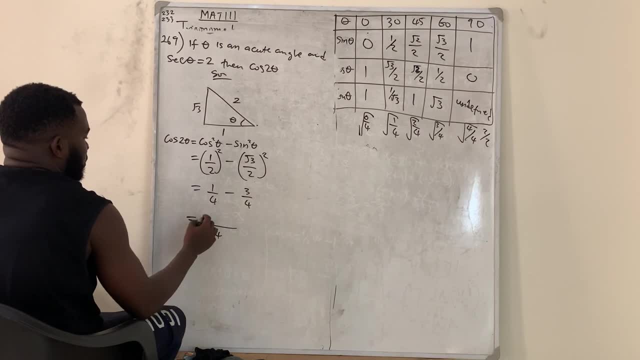 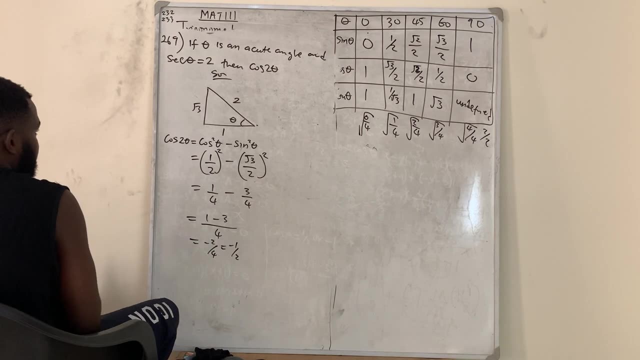 Minus 3 over 4.. So I'm going to have 4 here, 1 minus 3.. Which is what Minus 2 over 4.? Which is minus 1 over 2.. So minus 1 over 2 is the correct answer to that question. 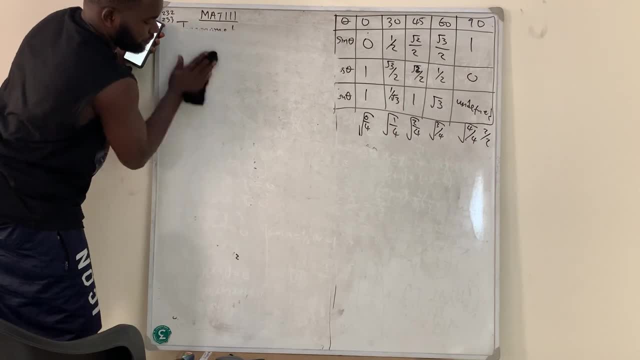 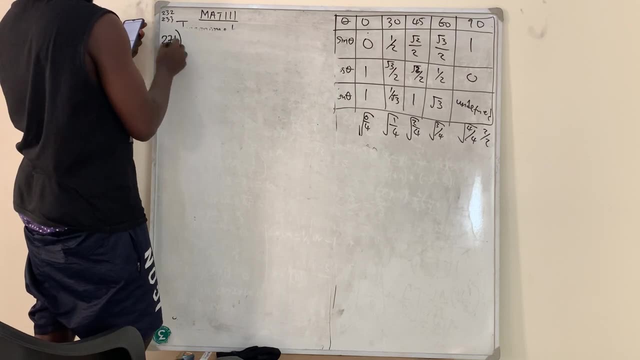 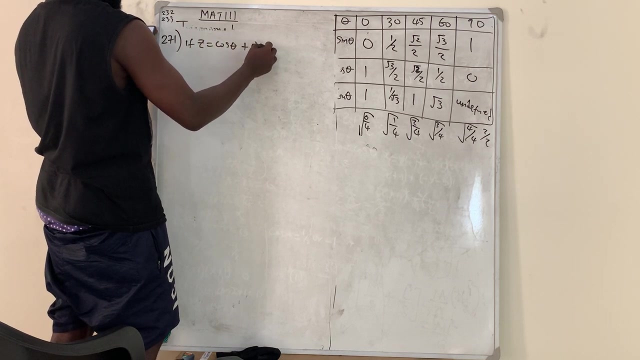 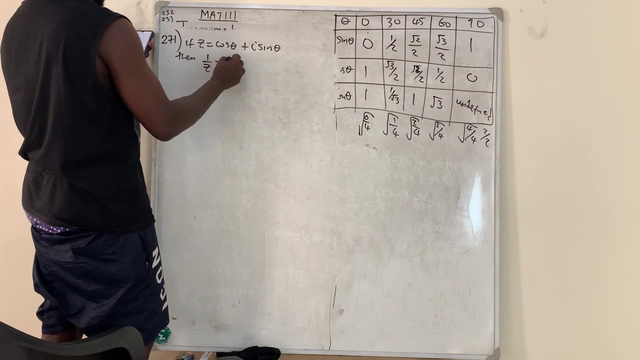 Okay, So we move to the next question, Which is question number 271.. Question number 271 said: If z is equal to cos Theta plus i sine theta, This is complex number. Then I say: then Then 1 over z minus z is: 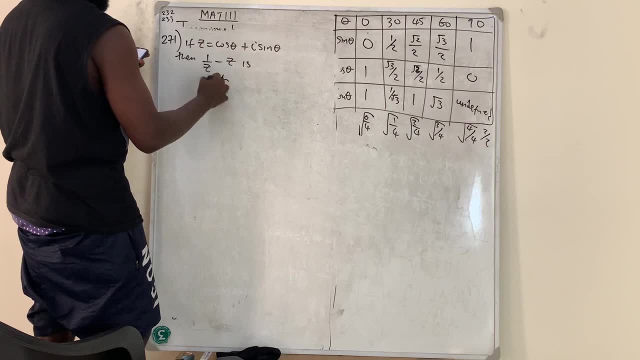 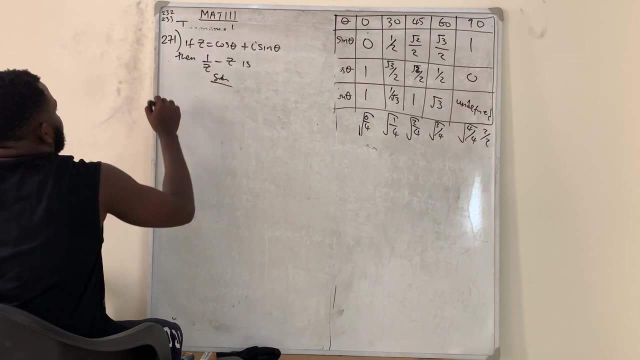 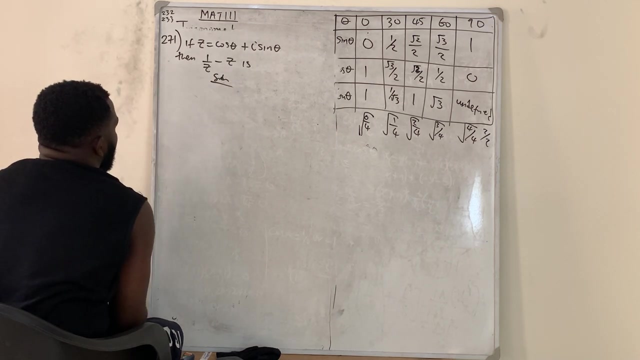 Okay, Solution Now. Now, 1 over z. 1 over z means inverse of this. I have them. What do I do? Do I start from here or do I start from here? Okay, Now I have 1 over z. 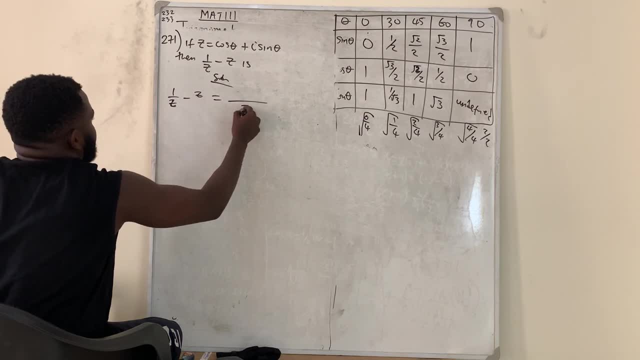 1 over z minus z, Which is what Elysium is z. I'm going to have: z divided by z is 1. 1 times 1 is 1. Minus Then z squared. Okay, So I have that distance. 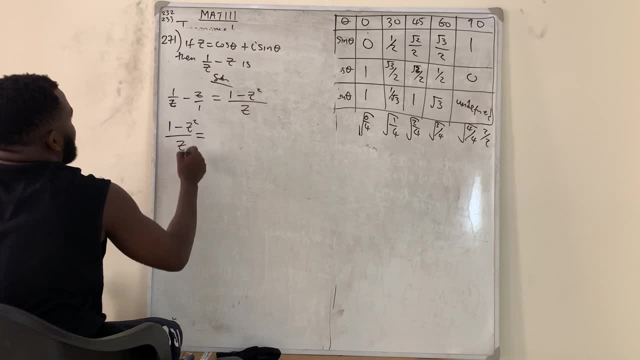 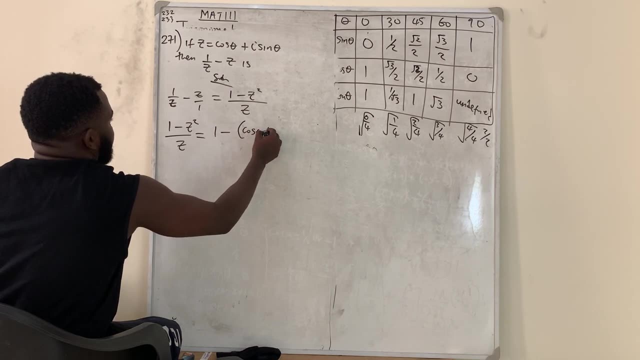 1 minus z squared over z. So which is what? 1 minus What is my z? My z is cos theta plus i sine theta. All squared Then, all over my z, This is cos theta plus i sine theta. Okay. 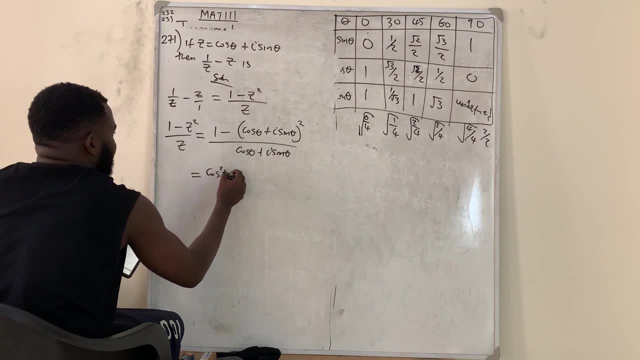 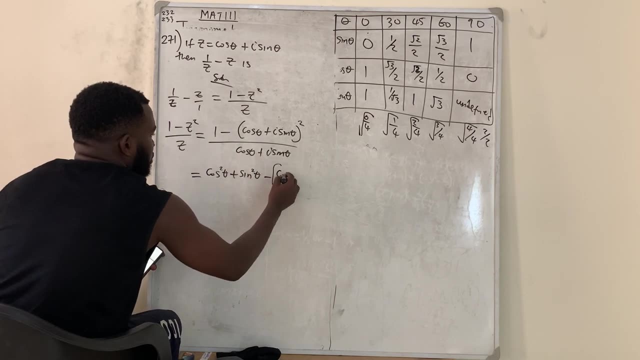 So now, Don't forget that 1 is the same thing as saying cos squared theta, plus sine squared theta, That's the mean of 1.. Then minus into- Let me open here: Cos squared theta. Okay, Now, This times is double it. 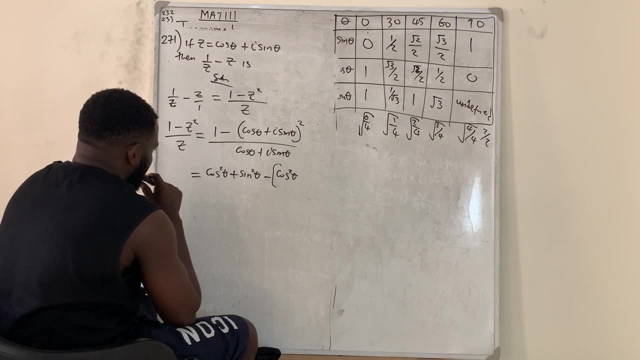 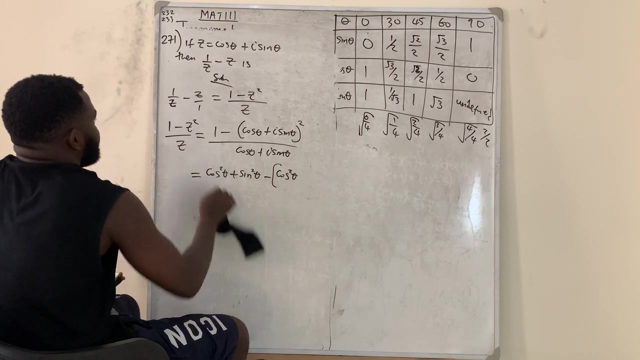 Will give you. This times is double. it Will give you what I'm trying to get: something Okay, This times is double. it Will give you. Or? Let me not start from here, Let me go straight to the point. 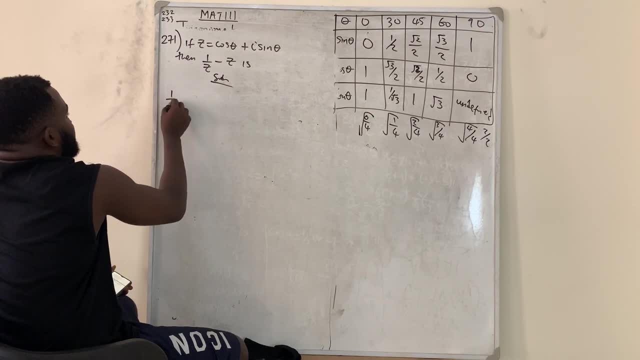 So that I don't want to make mistake. So I have, Let me say 1 over z. Let's see 1 over z. 1 over z is equal to 1 over cos theta plus i sine theta. So if I rationalize, 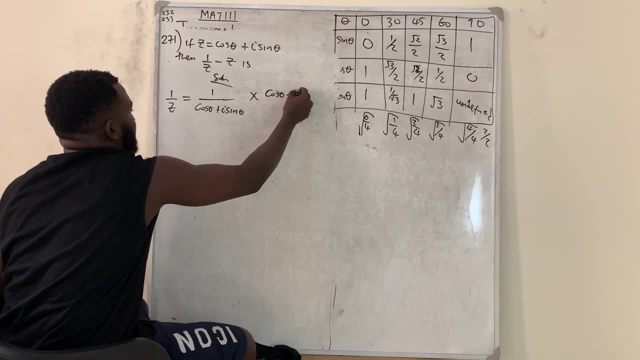 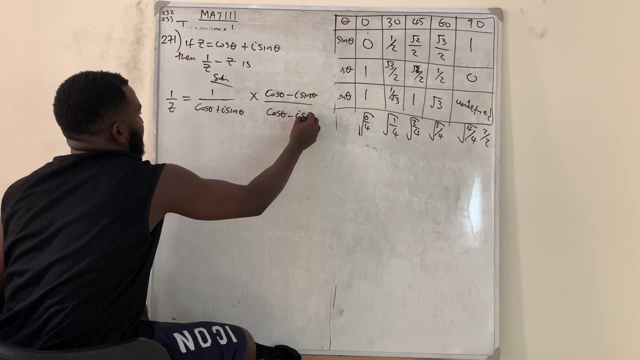 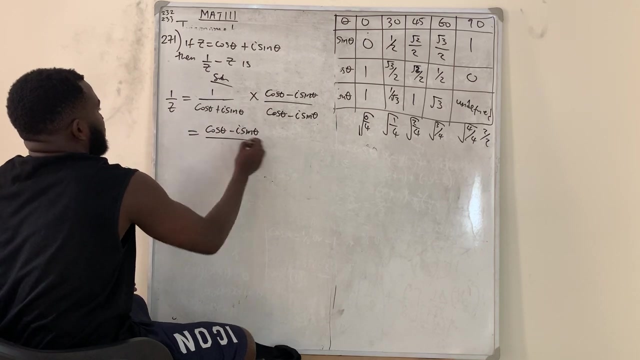 It's going to be times cos theta minus i sine theta All over. Cos theta minus i sine theta. So this times 1 will give you cos theta minus i sine theta All over. This time this will give you cos squared theta. 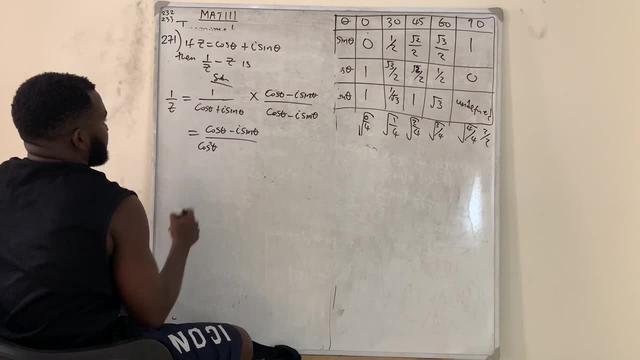 Okay, This time this will give you minus times minus, Minus times plus will give you plus sine squared theta. Yes, Do it, You will see that. So this is 1.. So this is giving me just Cos theta minus, i sine theta. 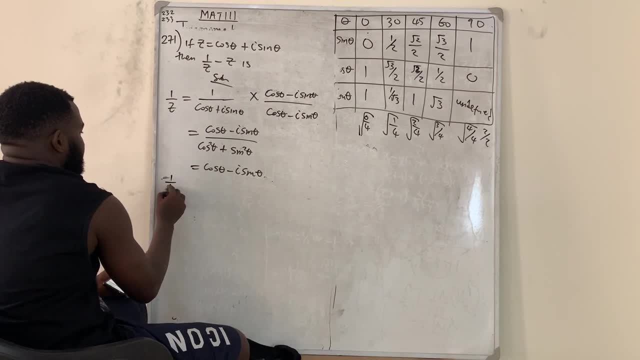 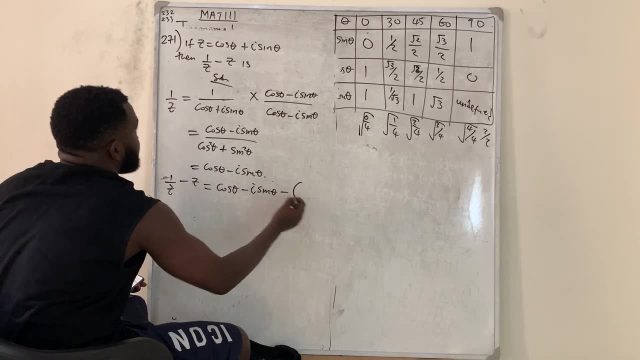 So if you now put it here, You now see that 1 over z, 1 over z minus z, is 17 hours. 1 over z gave me cos theta minus i sine theta Minus into This. one is giving me cos theta plus i sine theta. 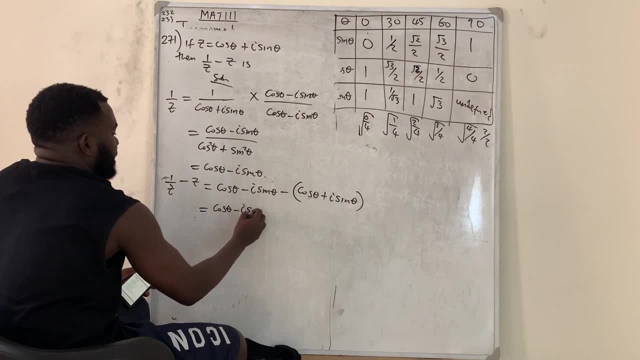 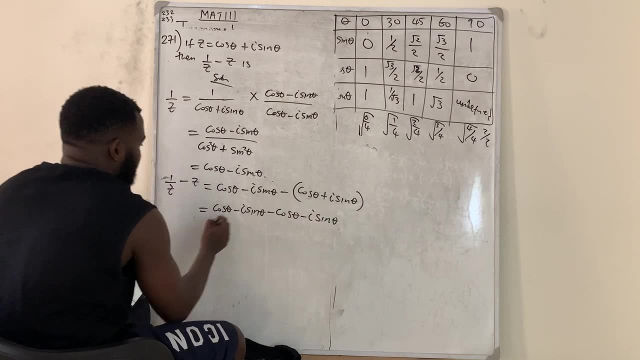 So if you open the bracket, You are going to have cos theta minus i sine theta Minus, cos theta minus i sine theta. So if you now do that, You are going to have This minus. This is cos This times will give you minus 2 i sine theta. 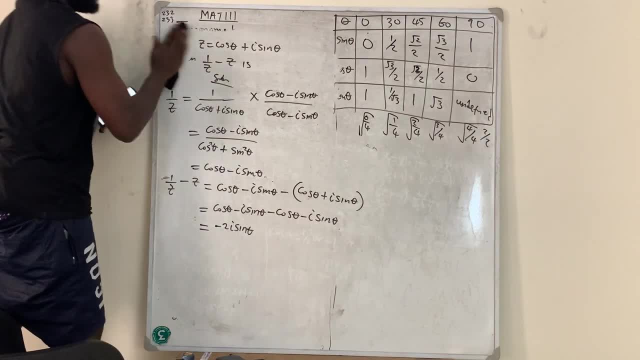 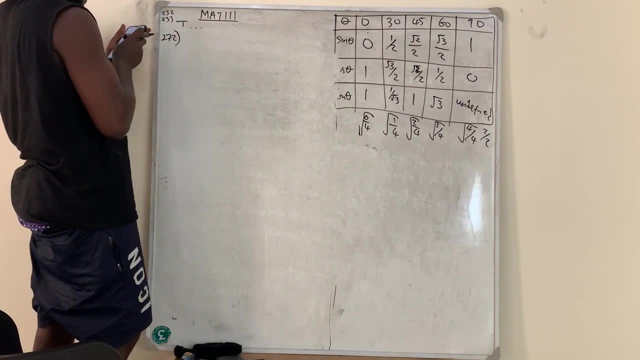 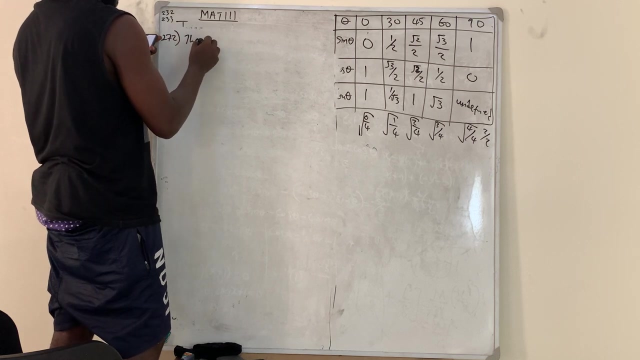 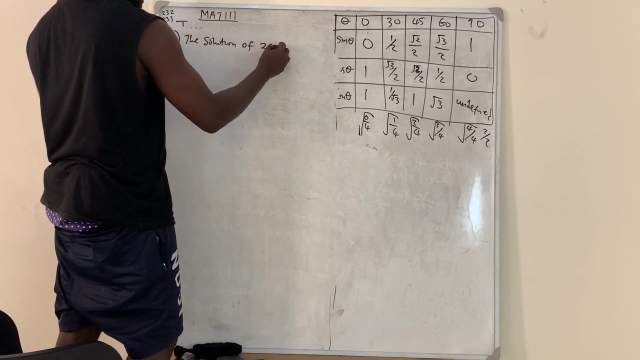 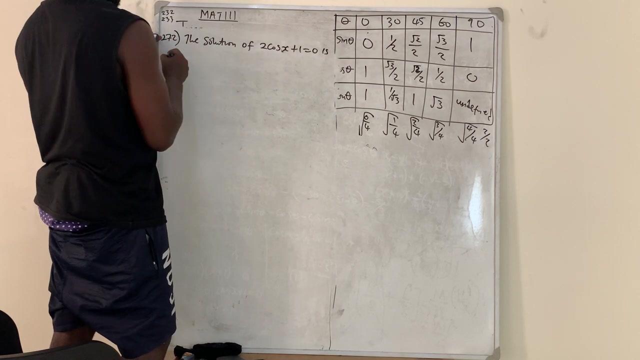 So that is the result. Okay, So we go to the next question, Question number 272.. Question number 272.. Question number 272.. To set the solution. To set the solution: The solution of 2 cos, 2 cos x. 2 cos x plus 1 is equal to 0, is 4.. 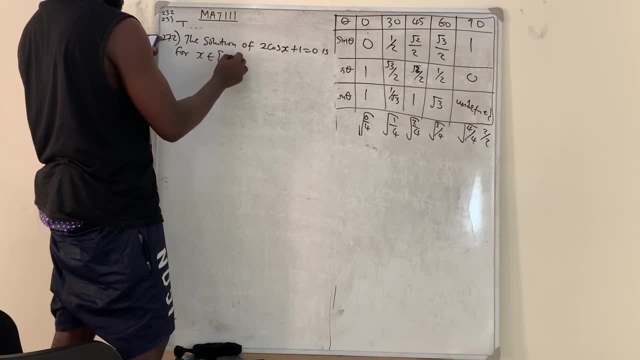 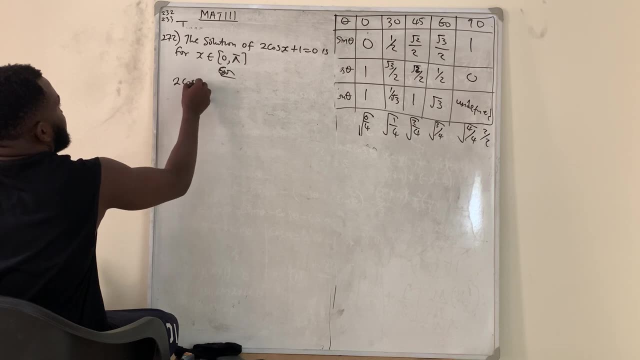 Then I say: 4 x is an element of from 0 to 1, 8. Okay Solution. So they gave me that 2 cos 2 cos x plus 1 is equal to 0. Therefore, 2 cos x is equal to minus 1.. 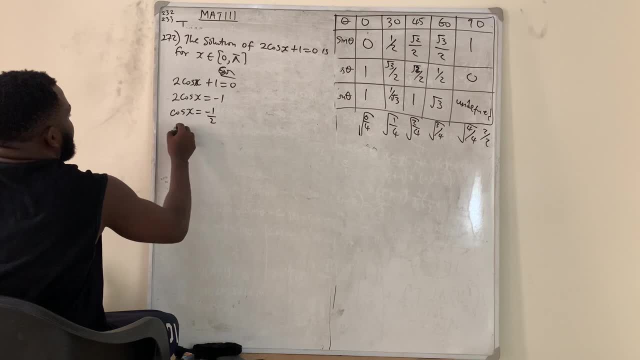 So x, sorry, cos x is equal to minus 1 over 2.. So x, So x will not be what my cos inverse, cos inverse of minus 1 over 2.. So which will give you what, In fact? which is 60.. 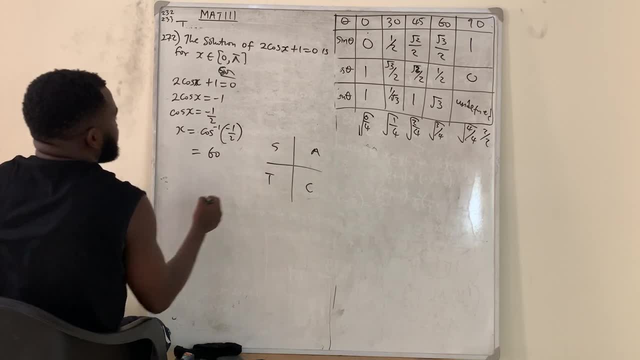 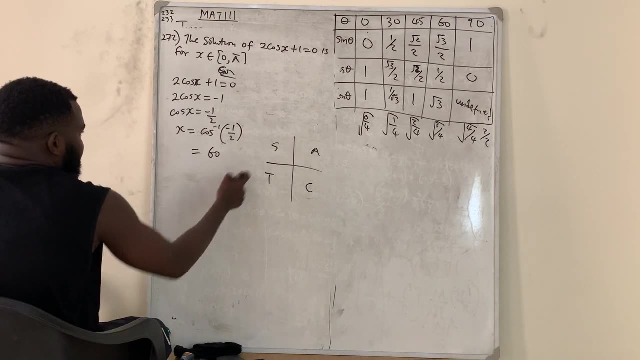 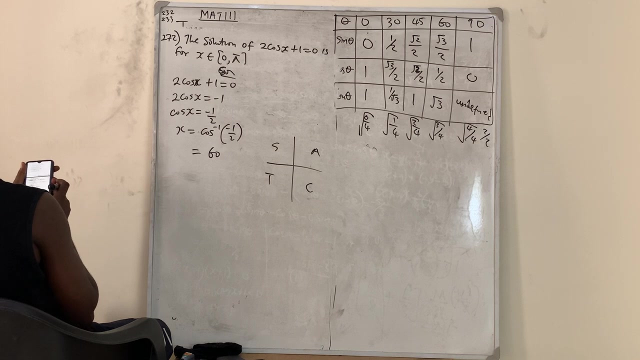 But this is C? A S T. So at what point is cos negative? Cos is negative at the second and the third programs, The second and the third program. So what do we do? So 180 minus 60.. 180 minus 60.. 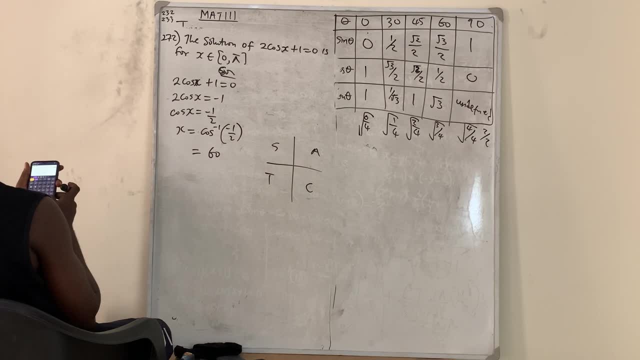 So give 180 minus 60. To give you 120. and I know that, cos the 120 is negative Absolutely, My X is 120.. 120 is one of them, Then another one, Let me take it There's another one that can give you. 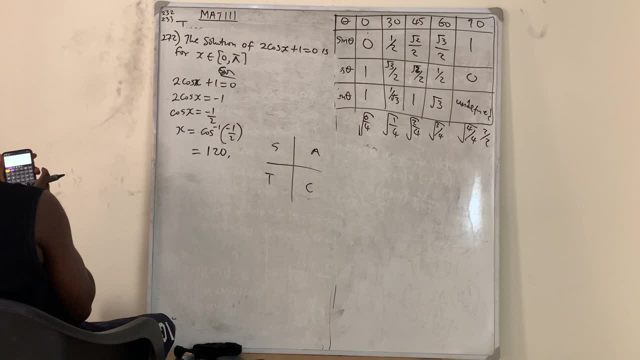 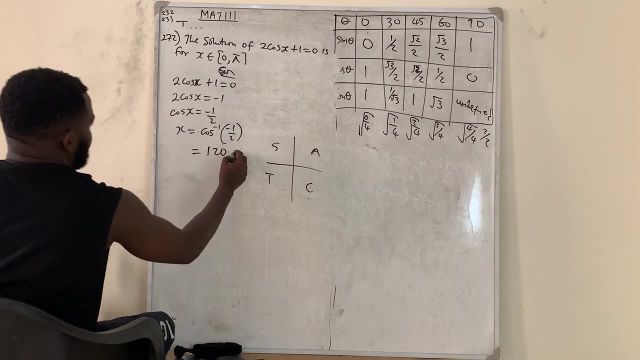 I don't think there's any other one, Because if you see 180 plus 60. I bet you have to 40.. So if you have cost to 40. Oh, minus Our 2, 40.. 40 is the only part of the answer. okay, but they say that it's from 0 to 180, so the only answer 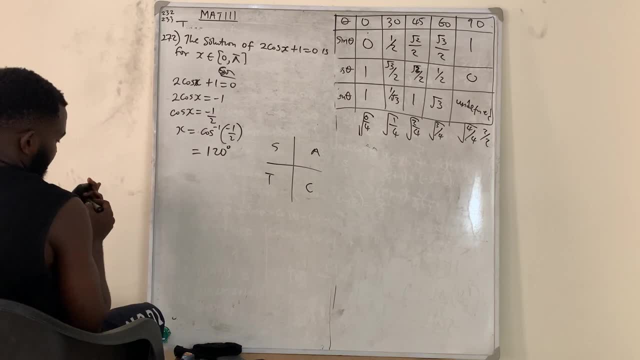 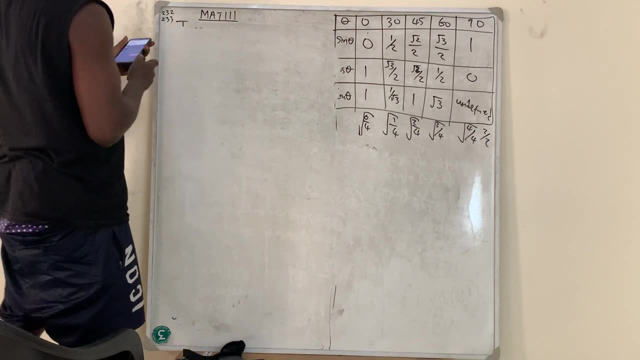 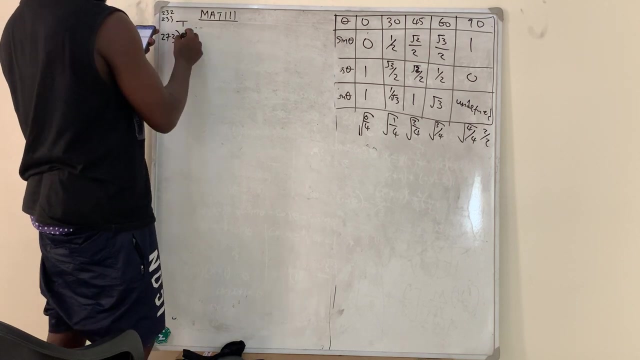 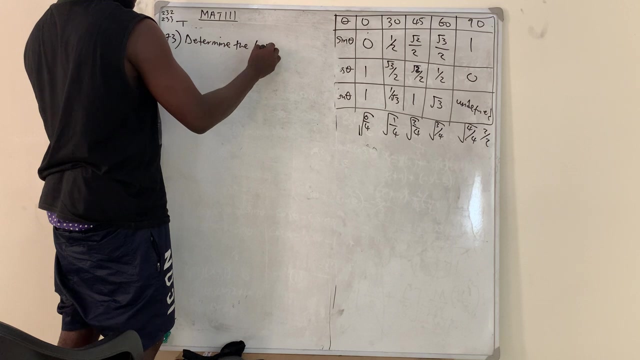 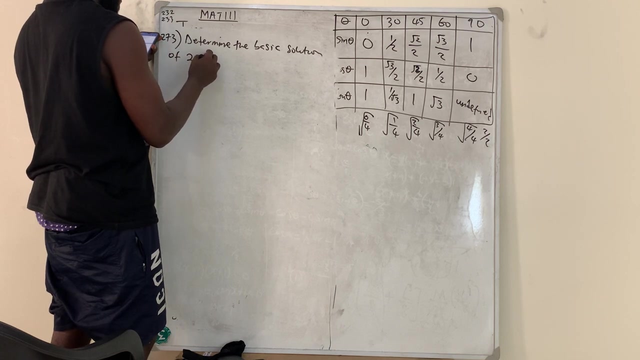 here is just 120, so 120 is the only answer here. okay, so we move to the next question. so, moving to the next question, i have question number 273. and question number 273 said: determine, determine the base. the basic solution of 2 cos square, theta plus cos, theta minus 1 is equal to: 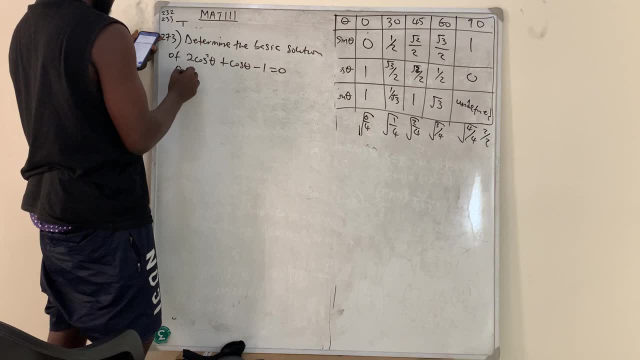 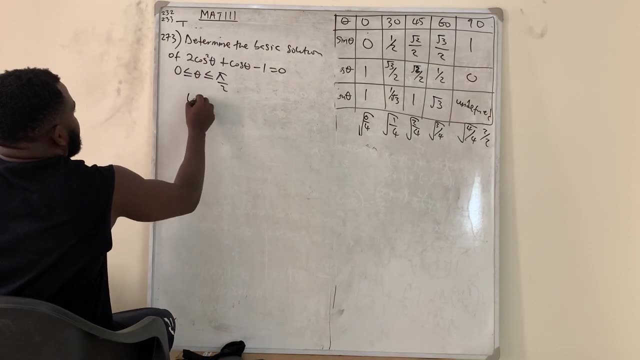 0. when i say for theta is less, for 0 is less than equal to theta, which is less than equal to pi over 2. okay, so let us solve this. we tell them that let's solution let, um, let's cos theta let's consider equal to x. so from here i'm going to have 2x. 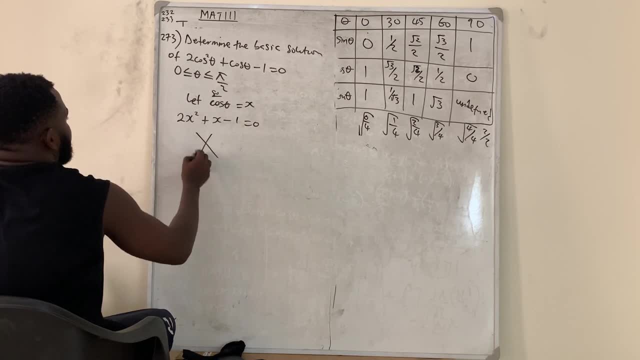 squared plus x, minus 1 is equal to z. so if i solve like this: x, uh, 2x and x, i'm going to say minus 1 and 1. okay to have that 2x minus 1 and x plus 1 is equal to z. this is normal factorization. 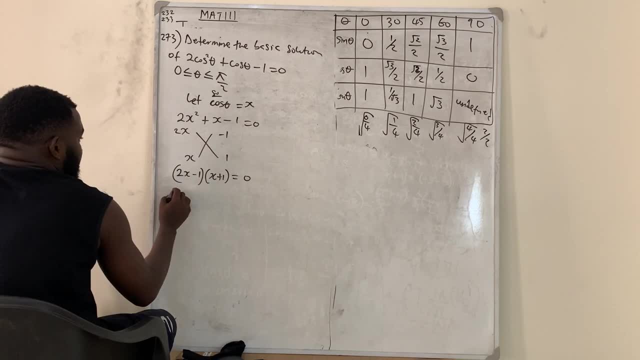 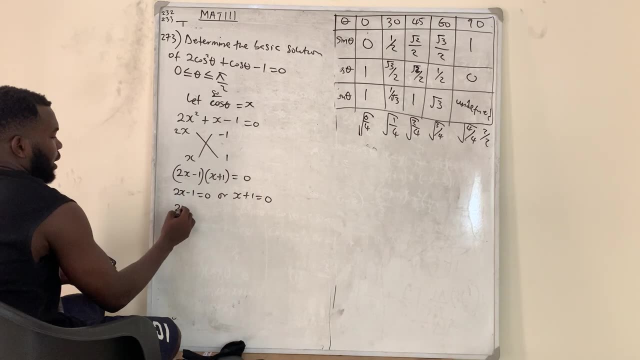 if you don't understand this type, do your normal factorization that you understand. so you have that 2x minus 1 is zero, or x plus 1 is zero. so what do you have? that um 2x is equal to 1, so x will not be worth. 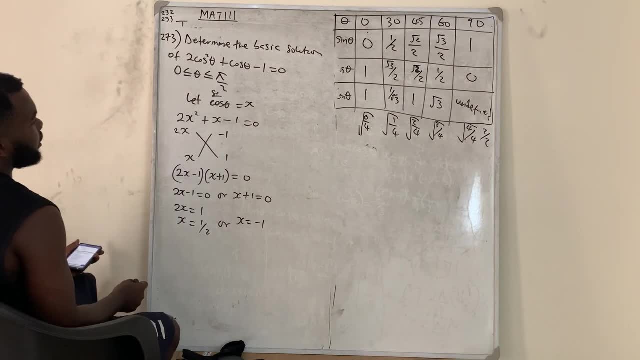 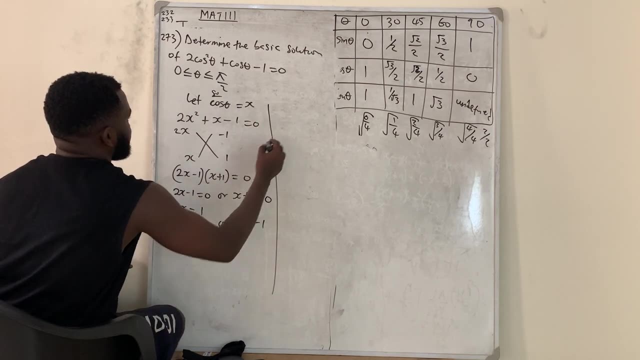 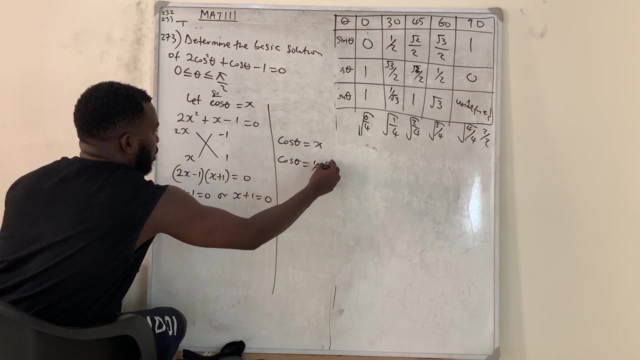 1 over 2 or x equal to minus 1. okay, so am i looking for x? no, i'm looking for theta. so we tell them that, um, there is a place. we say that cos theta, cos theta is equal to x. so therefore, cos theta is equal to 1 over 2, or cos theta is equal to minus 1, so therefore theta is equal. 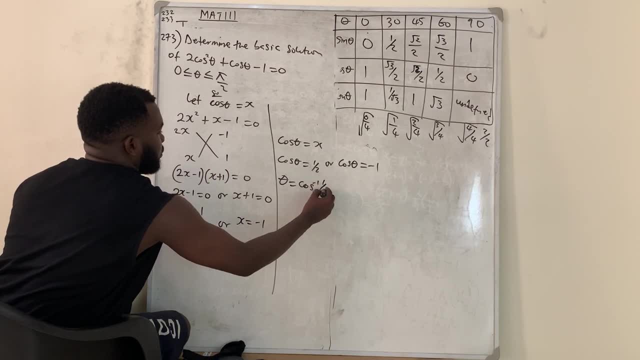 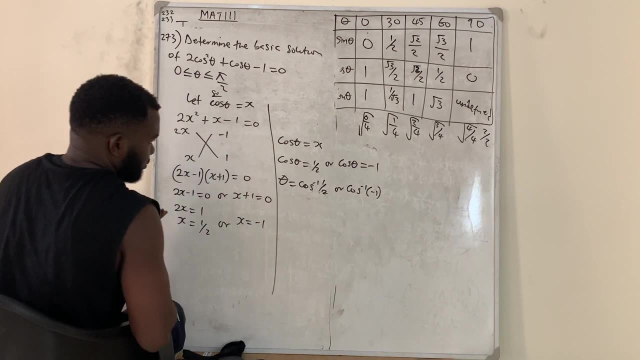 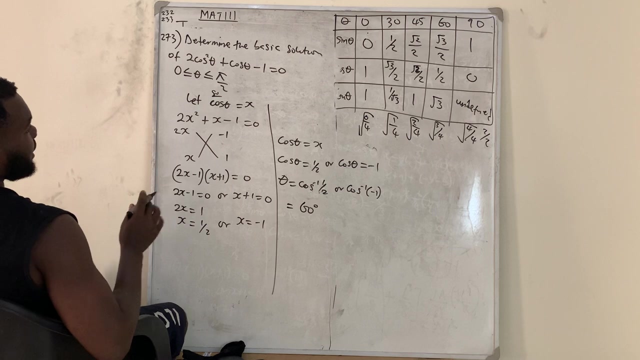 to cos inverse of 1 over 2, cos inverse of 1 over 2 or cos inverse of minus 1. so so, therefore, cos inverse of 1 over 2 is um 60, 60 degrees. okay, and that is the only answer there, because they say that is from 0 to 90.. i over t is 90, so the only answer here is this: 60, because 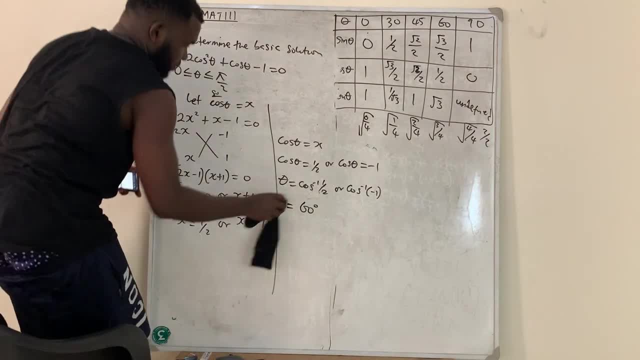 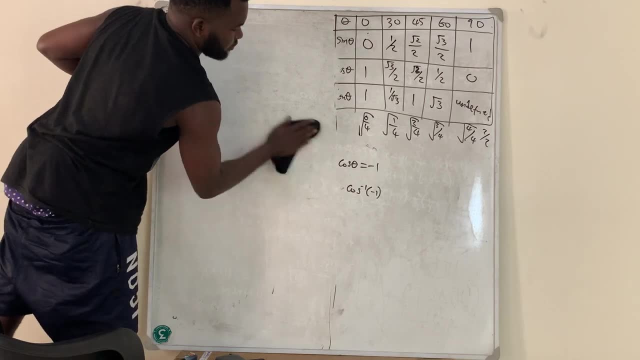 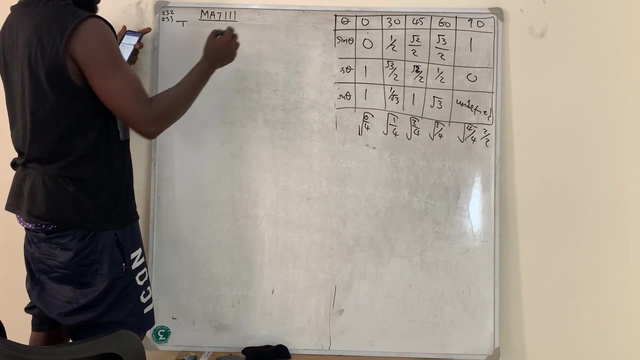 that one will give you something in the second and top order. so 60 is the only solution here. okay, that's the basic solution. okay, so that is that. so we move to the second, to the last question. okay, and 60. what is this? they are always irregular. 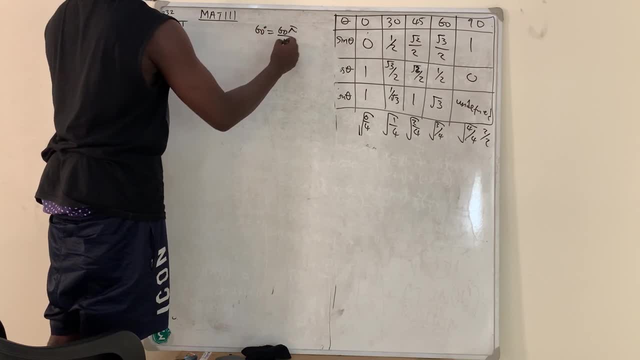 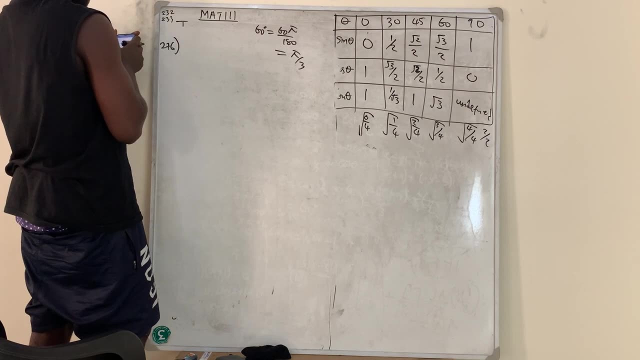 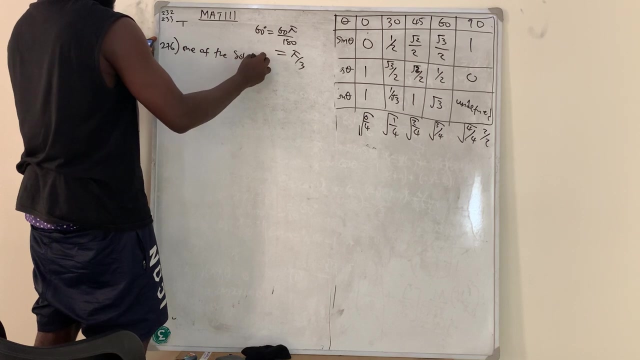 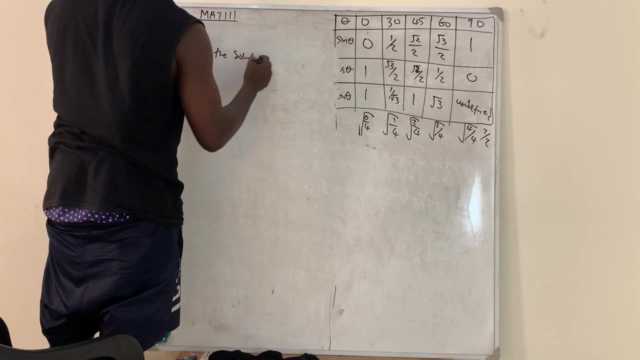 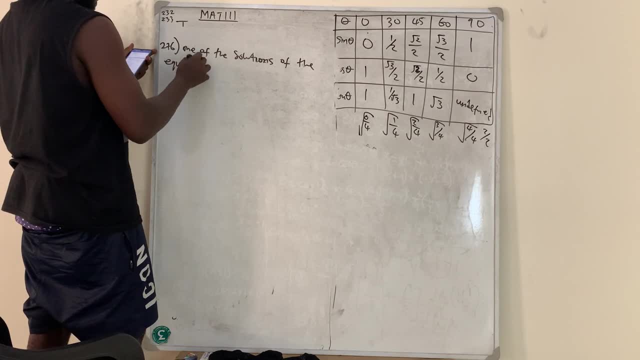 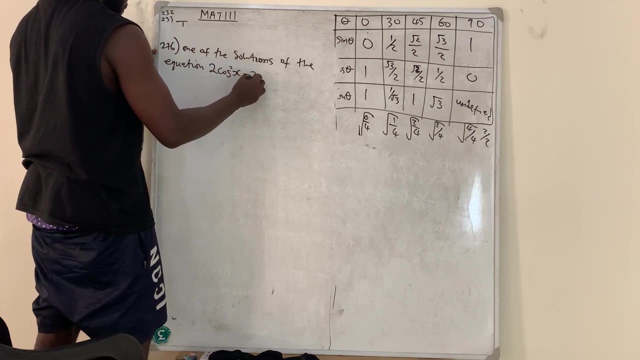 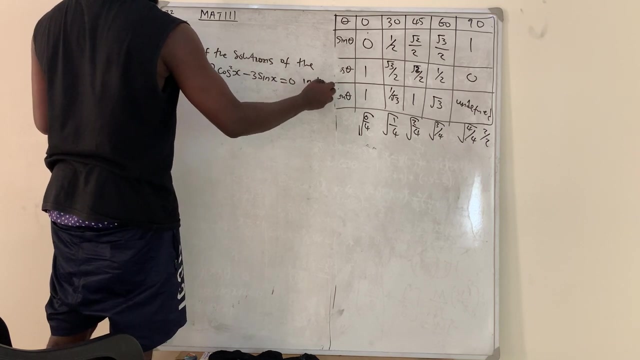 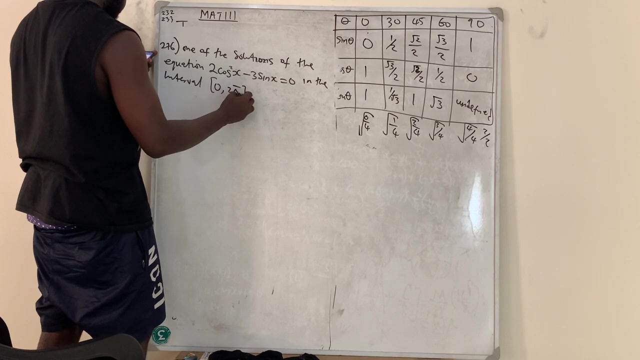 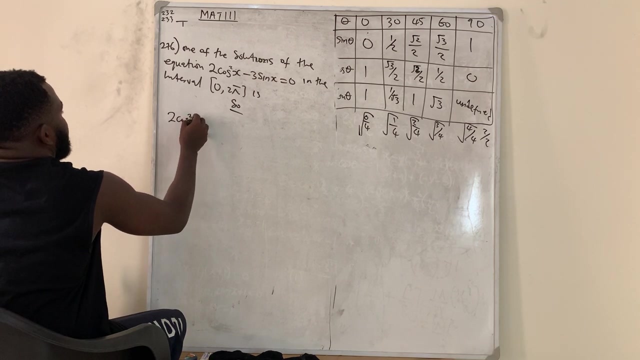 of the equation. one of the solutions of the equation: two plus squared x minus three sine x is equal to zero in the interval zero and two pi is okay. one of the solutions. now they gave me two cos squared x minus two sine x is equal to zero. the concentration is here. i want everybody to be uniform, so let me. 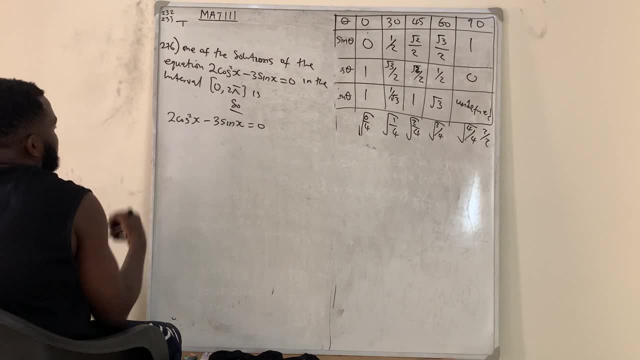 change this one. changing this one to cause will be difficult, but changing this one to sine will not be difficult. you know that cos squared x is the same as saying 1 minus sine squared x. so if you put it here, i'm going to have two in bracket. 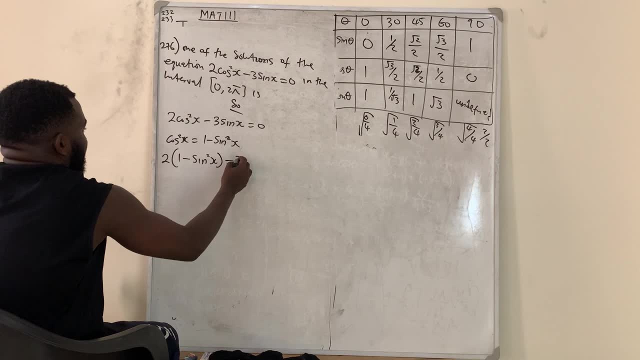 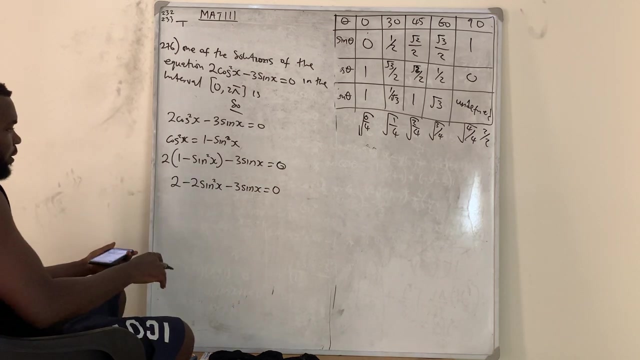 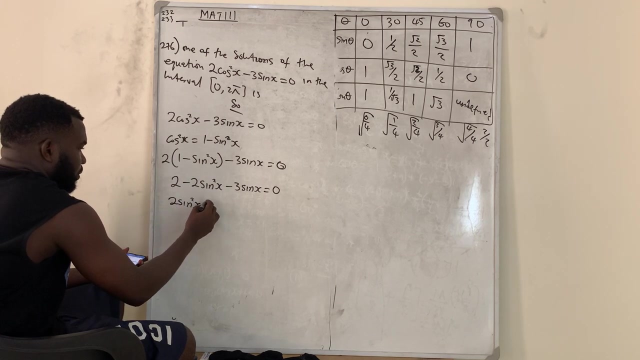 of 1 minus sine squared x, then minus 3 sine x is equal to zero. this time needs to give you two. this time needs to give you minus 2 sine squared x, then minus 3 sine x is equal to zero. so what do you have now? i'm going to have um, let everybody move. here. you have 2 sine squared x plus 3 sine x. 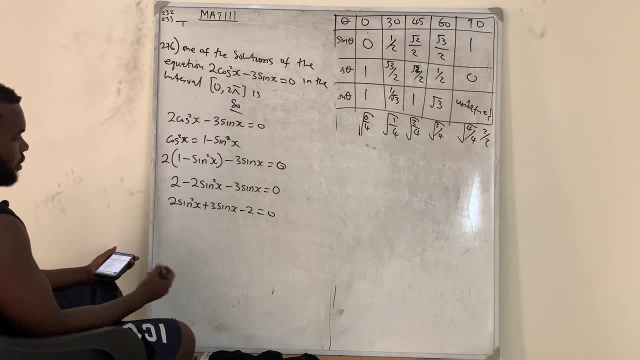 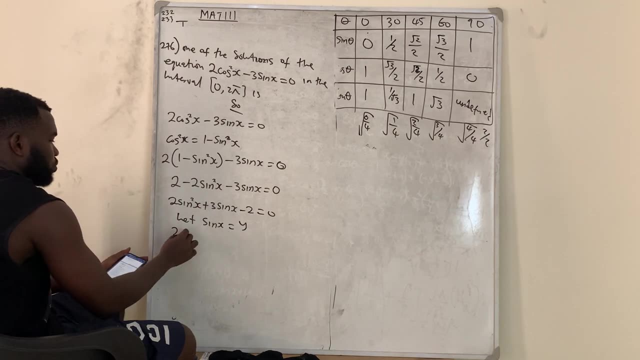 then this one moving you have minus 2 is equal to zero. okay, so you're gonna say, let's, let's sine x be equal to what y. so i'm going to have 2y squared plus 3y. minus 2 is equal to zero. so if